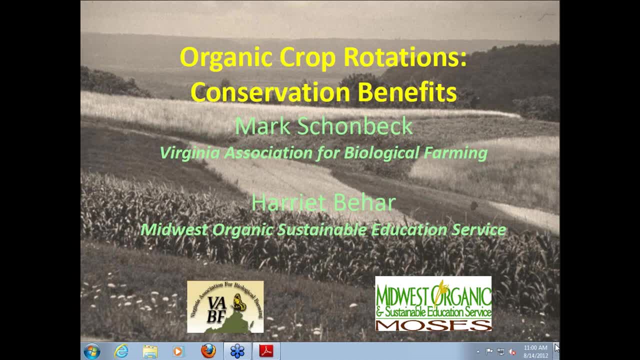 Hello everyone and welcome to today's webinar. My name is Jeff Szczesinski and I'm a project manager and agriculture economist at the National Center for Appropriate Technology, more commonly known as NCAT. I will be assisting in broadcasting this webinar. Organic Crop Rotations: Conservation Benefits. 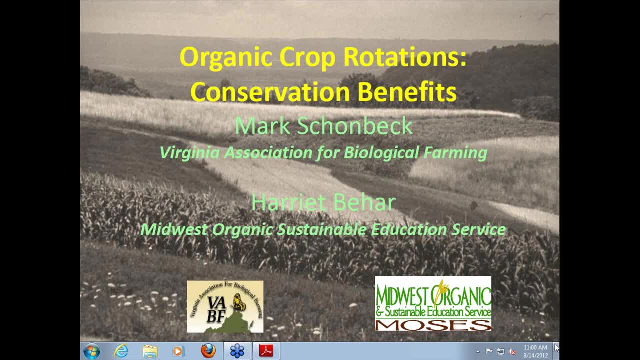 NCAT is one of 11 organizations who have joined with the Natural Resources Conservation Service, NRCS, in the three-year National Conservation Innovation Project that is working to better integrate sustainable and organic agriculture production systems into NRCS programs and procedures. Part of this project is to provide critical information and training like this to NRCS staff, farmers and others who may provide technical service to organic and sustainable farmers. 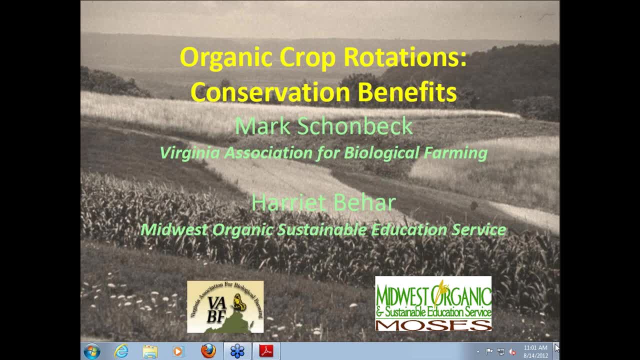 We are grateful to NRCS for its funding and support of this webinar and project. The 11 organizations who are joining with NRCS and NCAT in this effort are: the National Center for Appropriate Technology, NRCS and NCAT, The Center for Rural Affairs, the Institute for Agriculture and Trade Policy, the National Sustainable Agriculture Coalition. 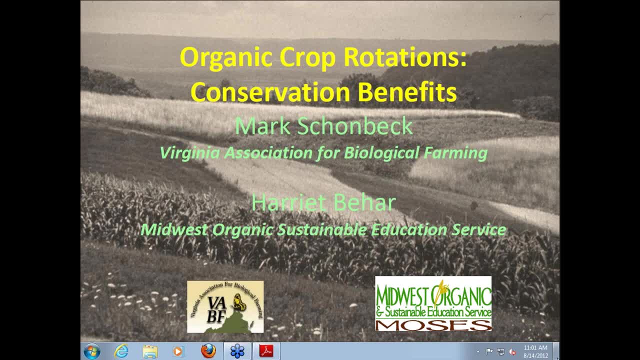 the Midwest Organic and Sustainable Education Service, Organic Farming Research Foundation, Virginia Association for Biological Farming, Florida Organic Growers, Kansas Rural Center, Wild Farm Alliance, Land Stewardship Project and Practical Farmers of Iowa. In addition to this project, one of the sustainable agriculture programs, 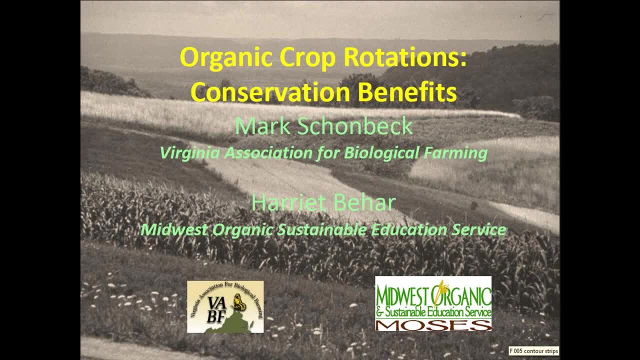 that NCAT manages. the National Sustainable Agriculture Information Service, which is better known as ATTRA, provides publications, technical assistance through our telephone hotline and website, webinars and other information to farmers, ranchers and educators, extension agents and those involved in sustainable agriculture across the country. 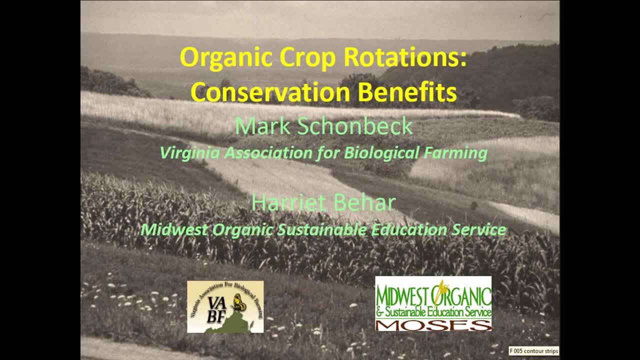 Today's webinar is being recorded and will be available on NCAT's ATTRA web page as well as through a link on the NRCS website and other project member websites. Our presenters today are: Mark Schoenbuck of the Virginia Association for Biological Farming. 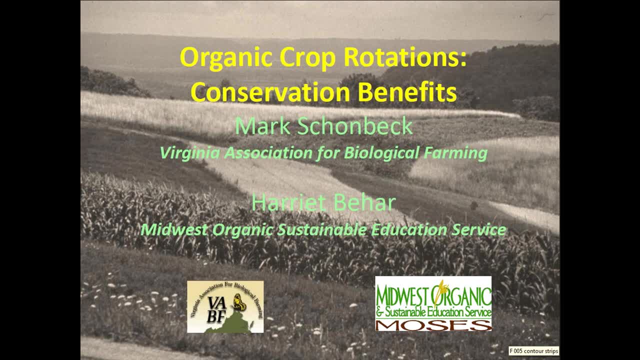 and Harriet Behar of the Midwest Organic and Sustainable Education Service. They will be discussing crop rotation strategies that many types and scales of organic farms can use to meet conservation objectives, market needs and USDA organic requirements. Specific strategies used by organic farms in different parts of the United States will be given. 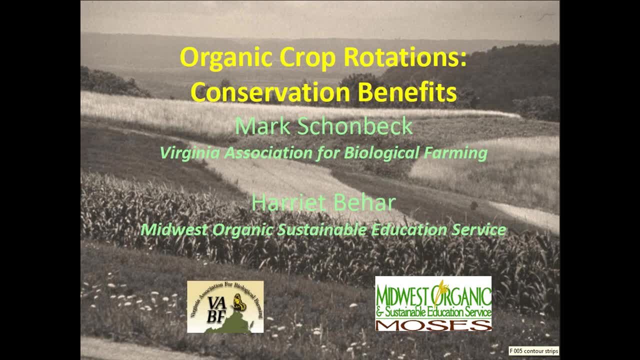 As you're listening to this, I'd like to thank you for joining us today, Today's webinar. you can type in any question you might have in the field you see on your screen. I'll gather them up, sort them out and have Harriet and Mark answer as many as we have time for at the end of this presentation. 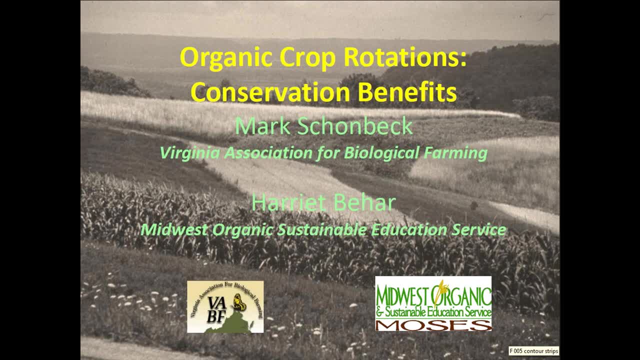 Please don't be shy about asking questions. We won't be able to get to all of them during the webinar, but we will get back to you via email in the days to come. Also, before we begin, I just want to remind our viewers to take a few minutes to complete the survey. 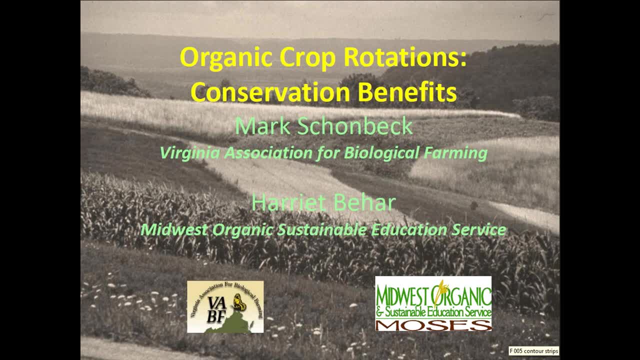 you'll see on your screen immediately after we close here. In fact, we always welcome your questions to ATRA. You're welcome to call our toll-free technical assistance line, 1-800-346-9140.. We also invite you to go to our website, wwwatrancatorg. 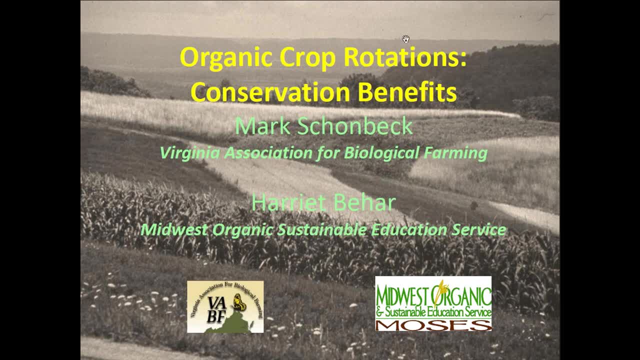 and click on Ask an Ag Expert button to send us a question by email. Don't worry, if you don't get that phone number or website, They'll be on your screen at the end of the webinar. We respond to all questions we receive and this service is offered free of charge. 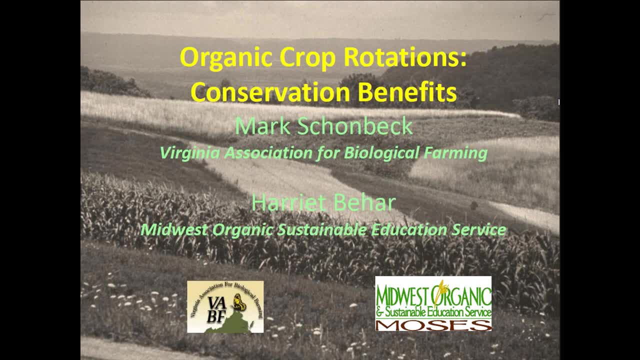 Our presenters, Harriet Behar and Mark Schoenbeck, have extensive experience in organic agriculture production. Harriet is an organic specialist with MOSES, the Midwest Organic and Sustainable Education Service, staffing their toll-free organic information line. writing organic fact sheets and articles. 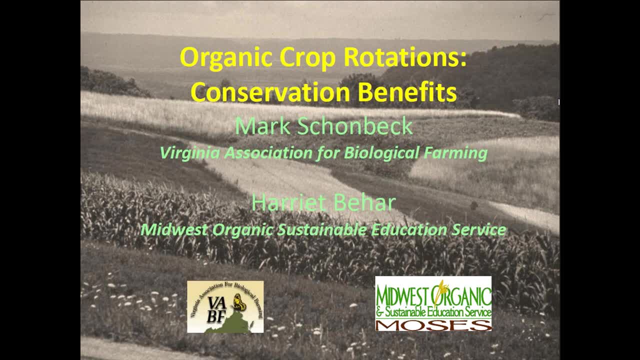 leading workshops and field days, as well as writing NRCS conservation activity plans for those who are interested in organic agriculture. She has over 20 years of experience as an organic inspector, with knowledge of organic, agronomic and horticultural crops, livestock and food processing. 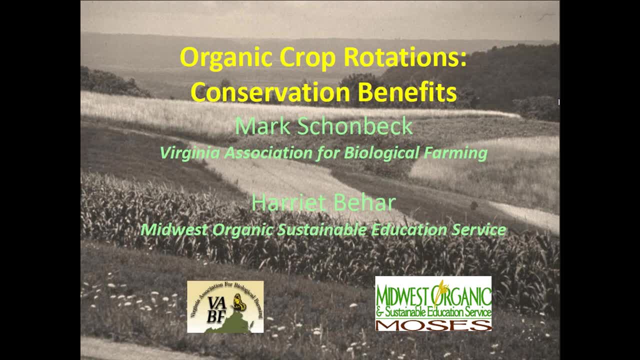 She and her husband run a certified organic vegetable and small grain operation in southwest Wisconsin. Mark has done sustainable agriculture research, consulting and technical writing for the past 25 years. His area's experiences include organic vegetable production, soil and nutrient management, soil test interpretation for organic systems, cover crops, mulchers, sustainable weed management. 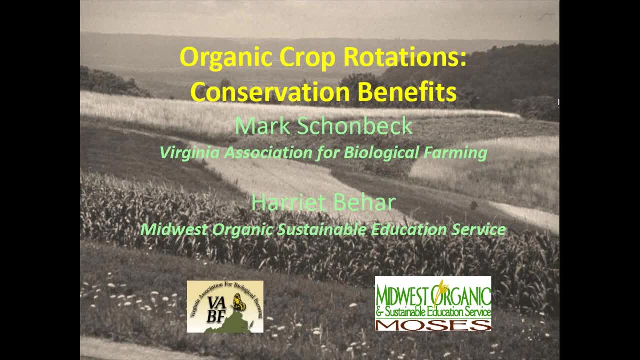 and soil and resource conservation. He edits the Virginia Biological Farmer, the quarterly 12-page newsletter of the Virginia Association for Biological Farming, and helps maintain a homestead garden for a small community of 15 people. He serves on the board of directors of the Southern Sustainable Agriculture Working Group. 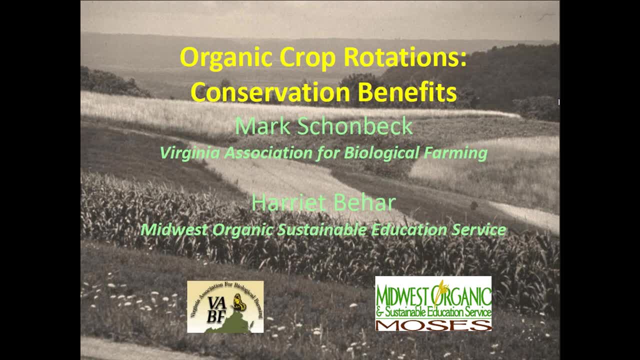 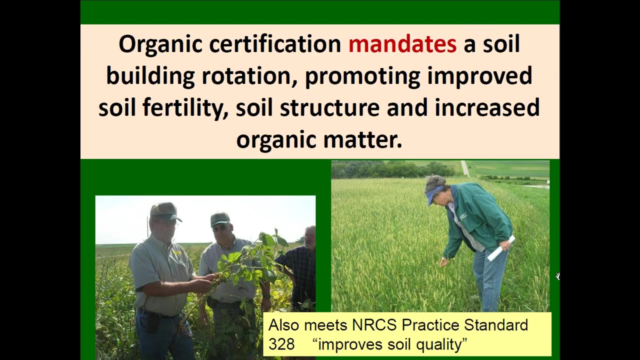 and does volunteer work in policy education and advocacy for family farmers. Thank you, Okay. our next slide for any. Welcome everyone. I just wanted to mention- I think most of you know- that the USDA has a law managing the word organic farming. 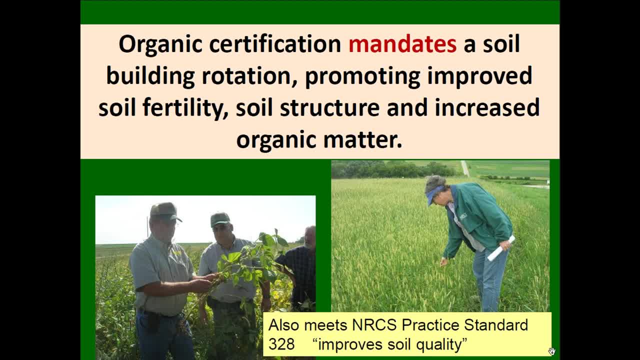 in the marketplace And part of that is that if you sell more than $5,000 a year, you have to be certified, And under that organic certification regulation there's a mandate that there is a soil building rotation where soil fertility and soil structure and increased organic matter are. 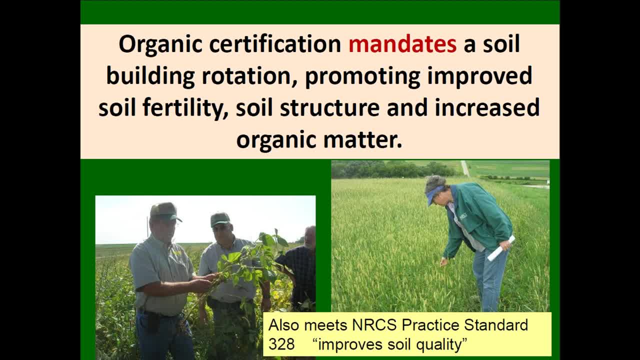 really the foundation of an organic farmer's production system on their farm And of course the NRCS believes in that as well, And many transitioning to organic farmers as well as existing organic farmers will use that conservation crop rotation practice, standard 328- to help them accomplish their goals of soil improvement. Next slide: 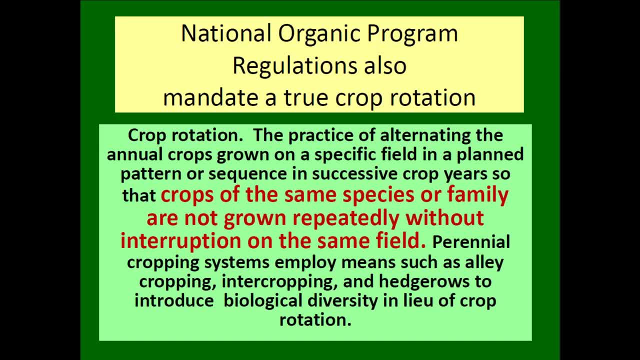 So this is actually the organic regulation of the words in red, or what's important here, This is the definition of crop rotation under the National Organic Program regulations, And that is that the same species or family are not grown repeatedly in the same field without interruption. So this is very important. So a corn on corn rotation. 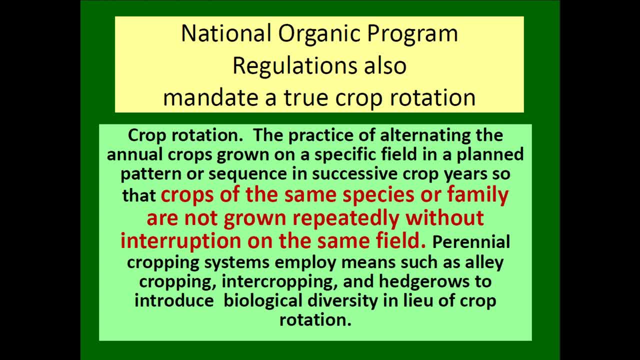 even a corn beans, corn beans, corn beans rotation would not be acceptable in an organic system And the farmer would not be able to grow in an organic system without interruption. And if a crop is not grown in an organic system then it's difficult to make crop rotation. 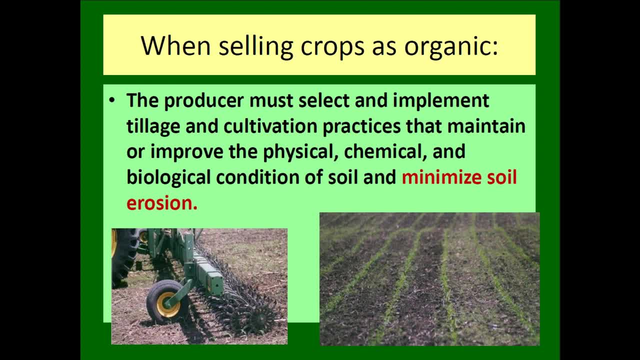 On the other hand, if it is a crop that is not grown properly- whether it's a grain crop or a crop that has been grown in the community for a period of time but it's not grown equally in a group of other organizations- then it is a crop that is not grown and it will not be certified. 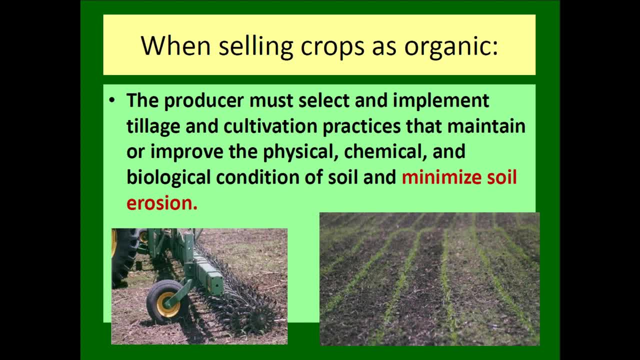 after a few years, if they don't include some sort of sod crop or legume in their rotation for soil building, may hear from their organic certifier that they need to put in contour strips or that they need to be putting in waterways, because an organic farm should be the gold standard. 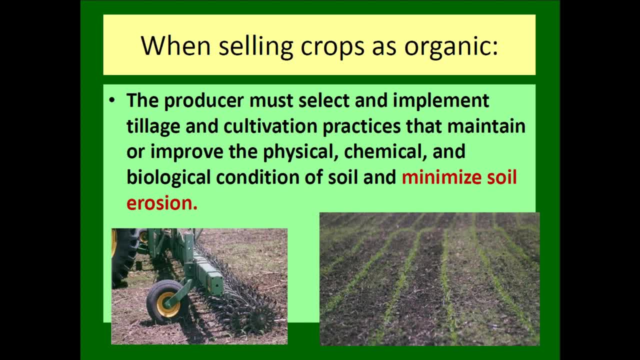 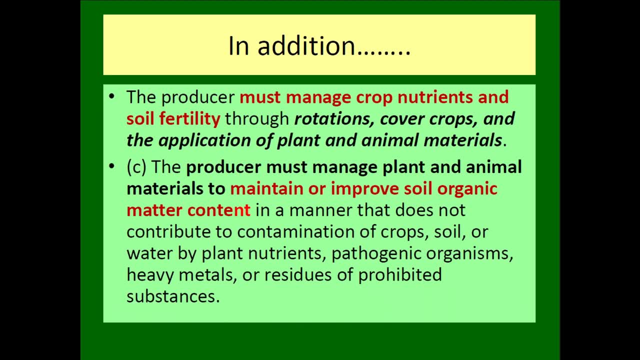 of protecting the soil and the water in their region. Next slide: There's other reasons too for crop rotations besides improving soil fertility and tilth, because it also breaks pest and disease cycles and things like that. But the other thing too is that even in the application of manures- animal manures- those need to be put on the 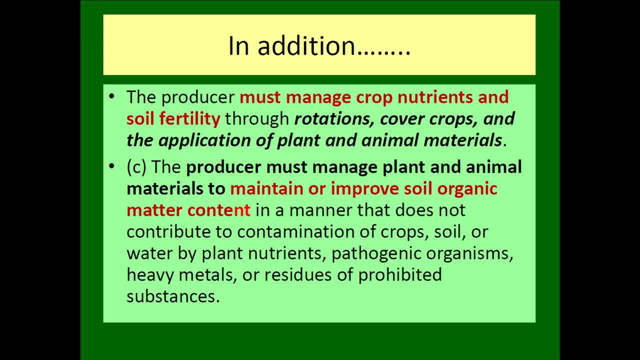 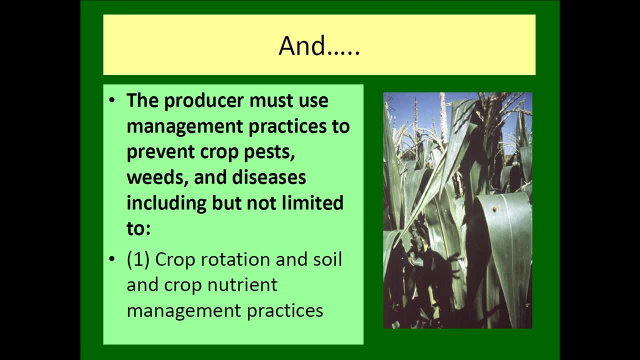 soil at a time and in such a way as to prevent pollution to crops or soil by those plant nutrients- Next slide. So, like I was saying too, pests, weeds, diseases are all broken when there is a diverse crop rotation, which is something that organic producers are doing on all their farms, and 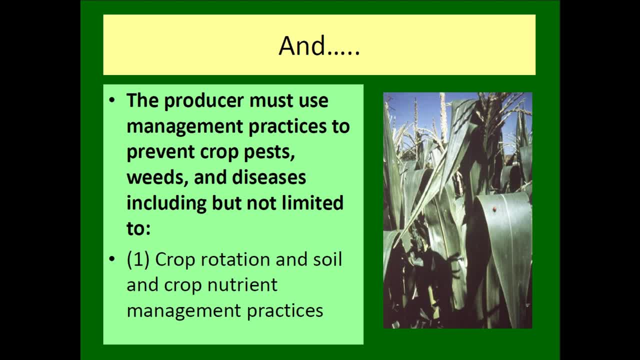 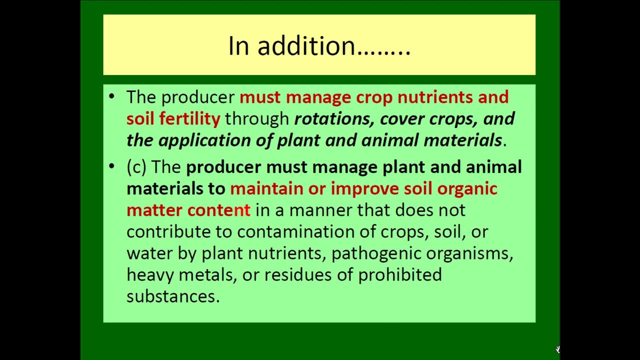 it's being actually overseen by the organic inspectors and the organic certification agencies during their annual visits. Next slide: So organic producers actually view organic production very holistically. They see that when they are adding this organic matter to their soil through the use of green manures, cover cropping compost. 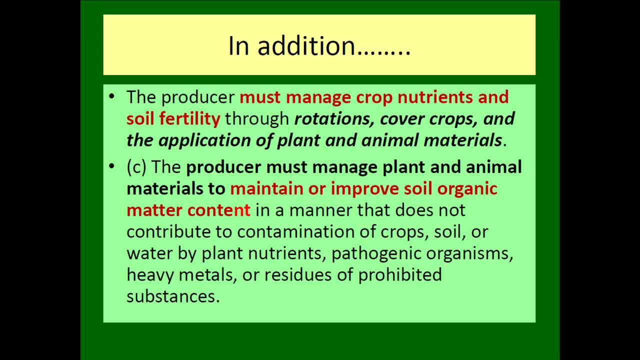 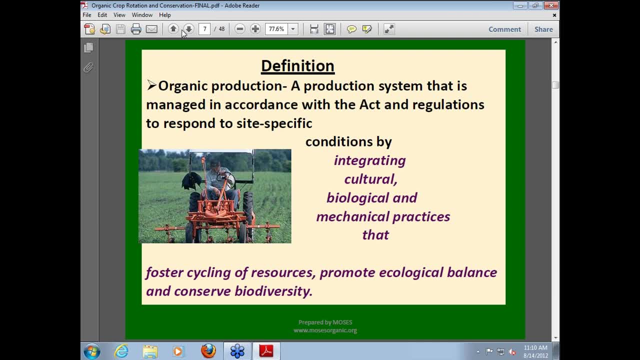 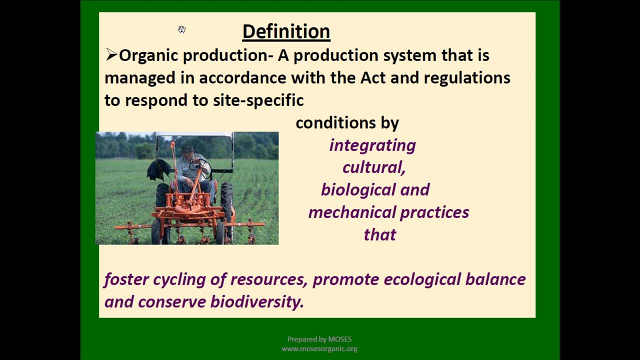 Okay, I think you went backwards actually Good. So this is actually the definition of organic production in the law And, if you notice, it doesn't really say what organic producers don't use, that they're not using synthetic fertility inputs or pest control. 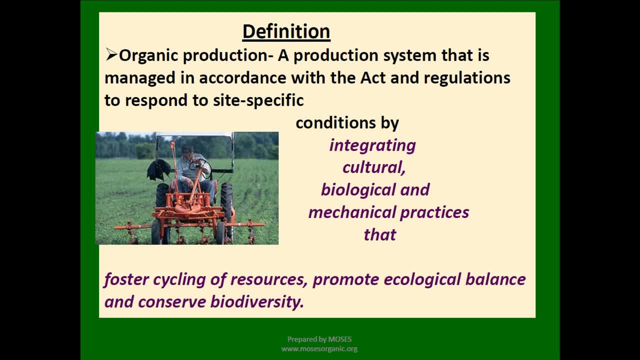 materials. It's much more of a holistic way of looking at their production system. So it's site-specific and it integrates cultural, biological and mechanical practices that foster the cycling of resources, promote ecological balance and conserve biodiversity. So that's. 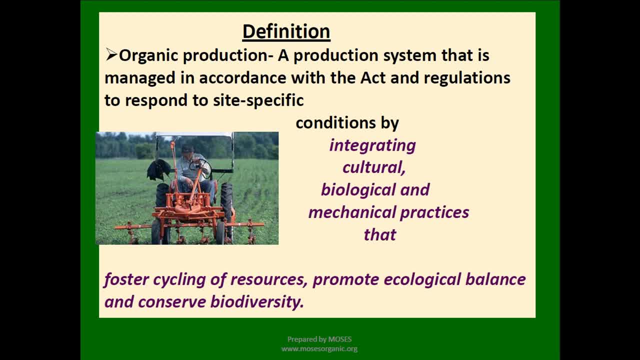 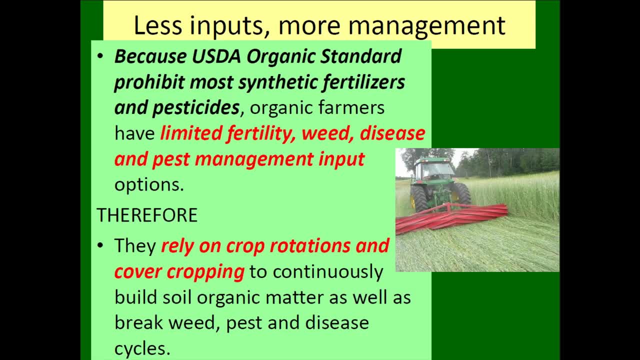 a very big picture Next slide. So under organic you're going to find that the producers are much more interested in management than input, because they have really a very limited scope of input that they can use for fertility, weed and disease management, So therefore they rely on cover. 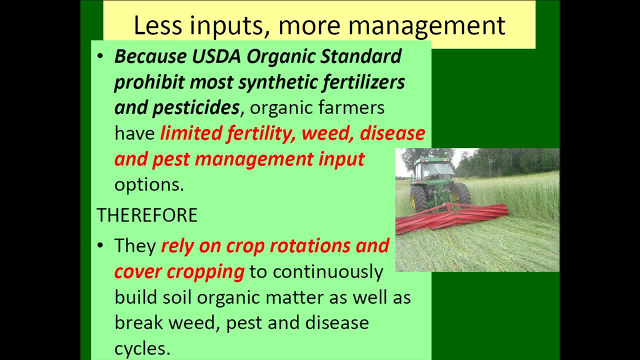 cropping and crop rotations to control their pest control. Okay, So that's the vision of organic agriculture. Next slide, Next slide. So organic farmers are interested in the use of organic materials to control their pests and disease problems, to break those weed cycles and, of course, to build soil. 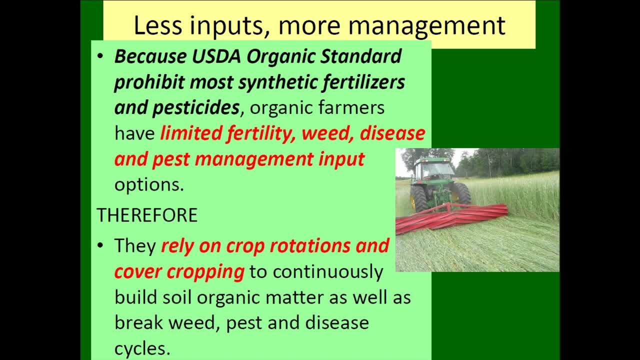 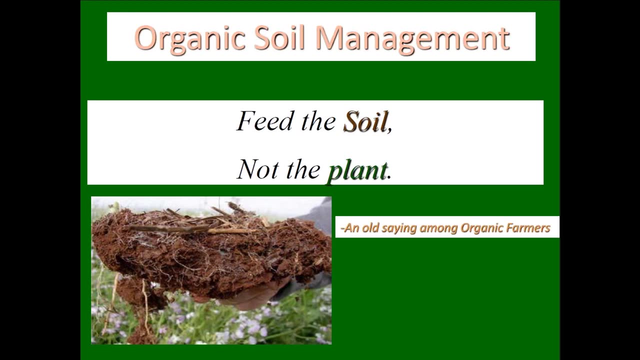 organic matter, which gives them better soil tilts and makes their cultivation more effective, and all kinds of wonderful things Next slide. This is an old saying amongst organic farmers that feed the soil, not the plant. So they're always looking at improving the soil biological balance. So they're always looking at improving 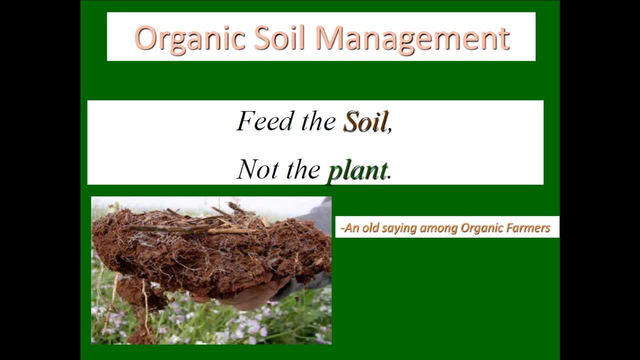 the soil biological balance. So they're always looking at improving the soil biological balance. They're always looking at improving the soil biological balance. So if you need a term for it, you can use organic farming instead of help. So organic farming is one of the two ways to remove weeds to decrease the smell of. 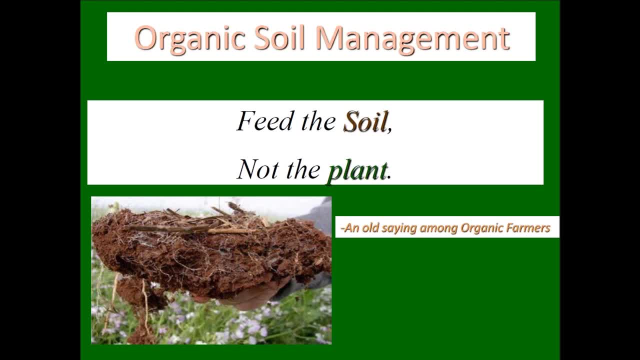 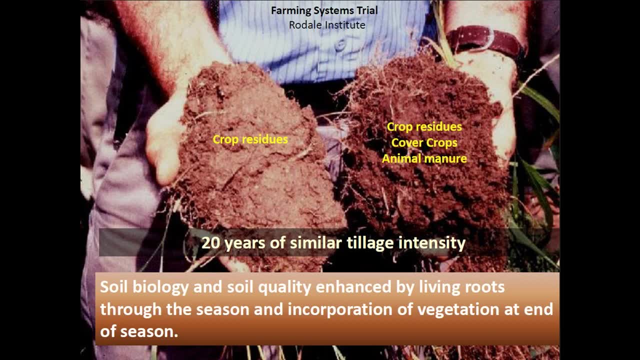 weeds to reduce the amount of diseases such as the tuberculosis virus. and of course, it can be used with organic products. but the older you are, the better it can be if you have the organic method. Okay, So next slide. 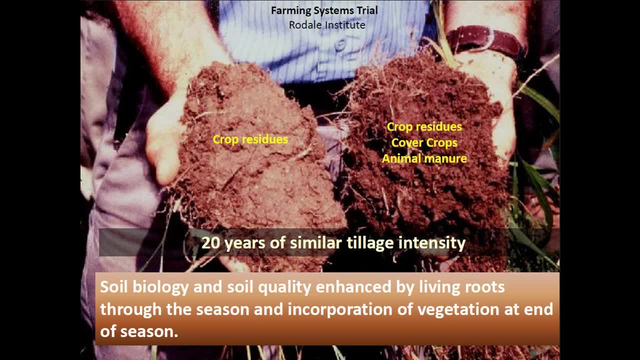 This is a slide from the Rodale Institute: The people who have been producing the organic gardening magazine- and they had New Farm Magazine for many years- comparing the soil color and tilt between 20 years of similar tillage intensity, with just crop residues returning to the soil. 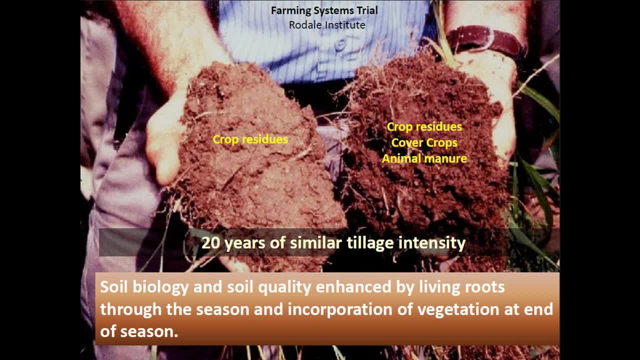 Next slide. Next slide turn to the soil, and with an active system of adding cover crops and animal manures in the same time, And they have side-by-side conventional and organic trials going on. that have been over 20 years, And so we have quite a bit of scientific evidence and, of course, many of you soil agronomists. 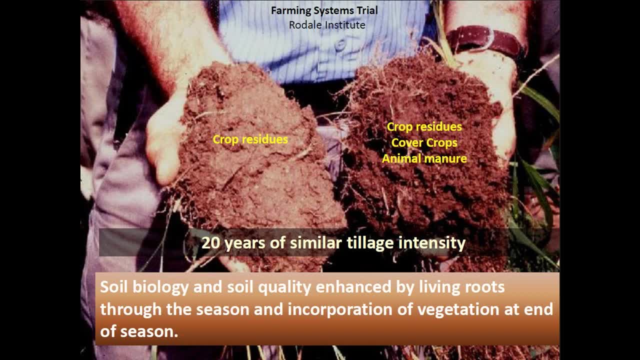 know that when you do continually work at adding organic matter to the soil, you are going to get that deeper color, better smell and better soil tilt. The other thing that organic farmers also really understand is that if they can have those living roots, that the incorporation, 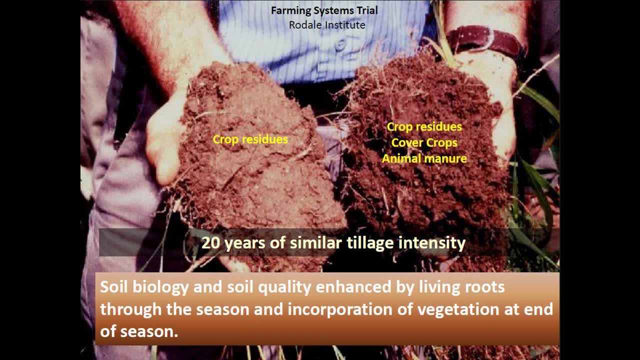 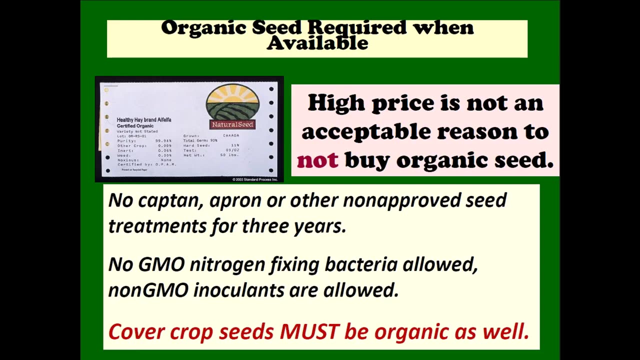 of organic matter is not just basically brown organic matter but living vegetation with living roots, because those really do attract the soil biology and enhance that Next slide. Just as a little reminder: if you are working with organic producers, they do need to use 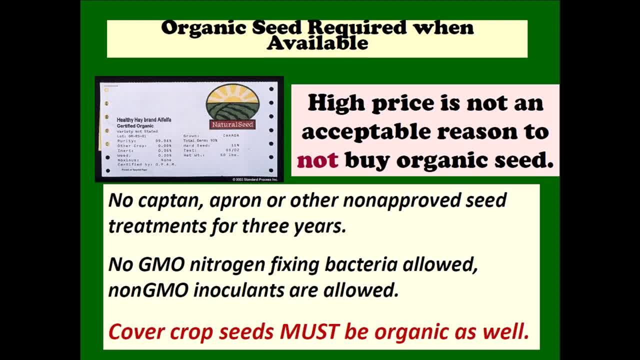 organic seeds, and that includes any cover crop seed or green manure seed. If it's available as organic, they must use it, And high price is not an acceptable reason to not buy organic seeds. And most synthetic seed treatments are not allowed and GMO nitrogen fixing bacteria. 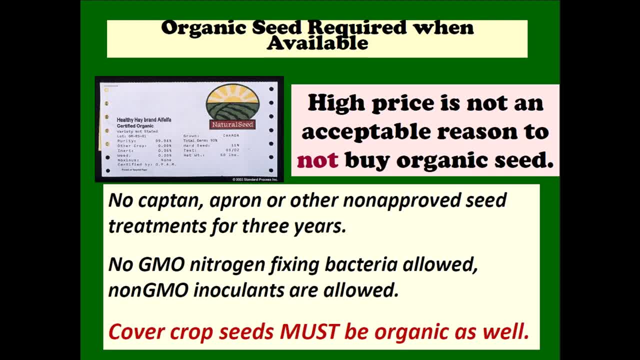 is also not allowed, And there are GMO rhizobial bacteria out there. so that's something that the organic producer has to be watching out for, because if they use any prohibited synthetics, including that GMO bacteria, they will then be back to their three-year transition to organic. 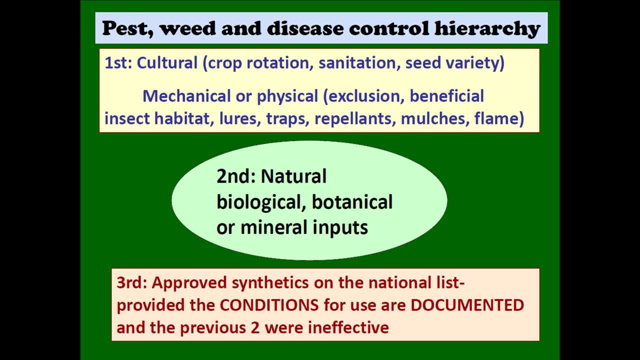 Next slide. Also in the regulation, is an actual hierarchy in what the organic producer must do in order to control diseases, weeds and pests in their field. So the first thing they should be looking at are cultural activities like crop rotation, sanitation, mechanical or physical exclusion, planting of 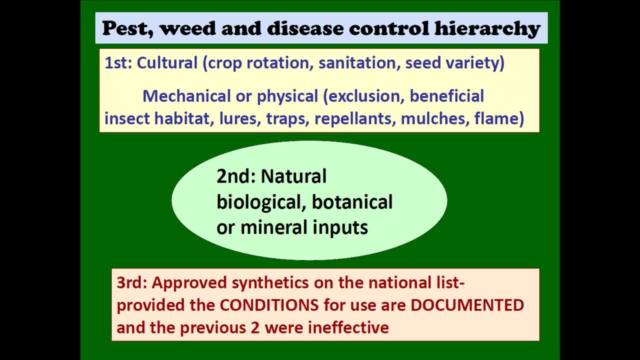 beneficial insect habitat, repellents, mulching, flaming, that sort of thing. Second, they're allowed to move to biological or botanical or mineral inputs if the first has not been effective. And lastly, there are a list of approved synthetics on a national list for organic producers. 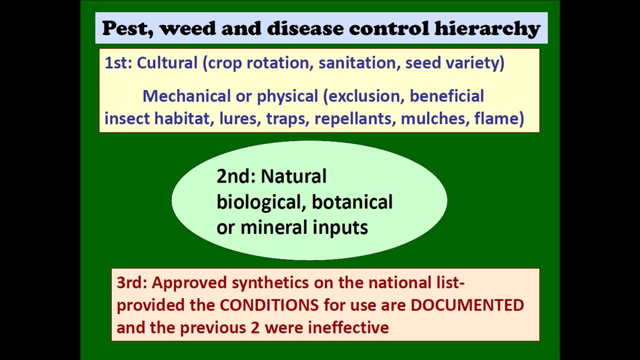 but if they're going to use any of those synthetics they have to prove that the first two were ineffective. with some sort of observation log or soil fertility or whatever their pest problems. They have to be documenting that they tried the first two, basically a systems-based. 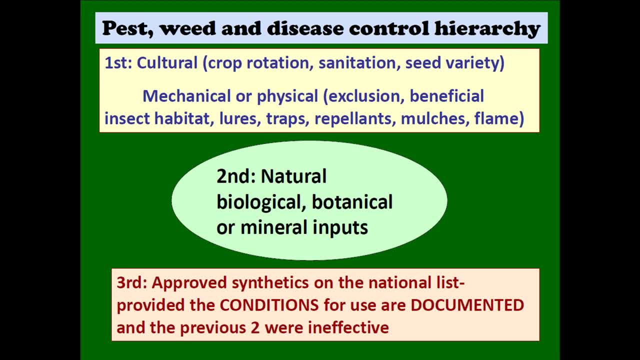 approach or something using natural inputs before they can move to synthetics. So for those farmers transitioning to organic, it is kind of a big change. We're not just substituting an approved organic input from the conventional input. You really are approaching pest weed. 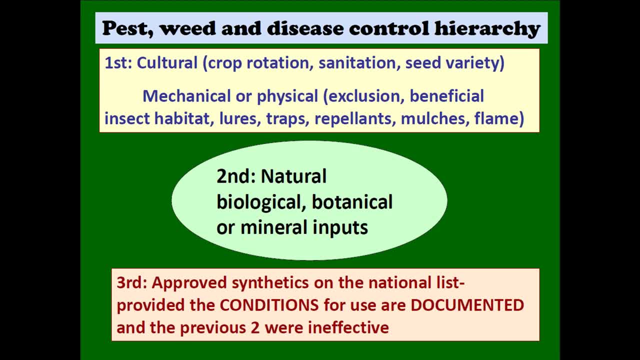 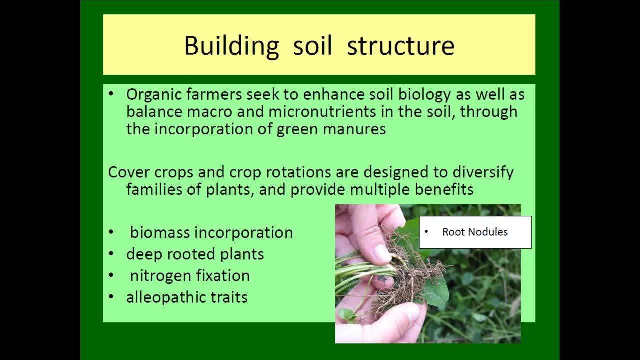 and disease control, as well as fertility management from a holistic system. Next slide, Next slide. So organic farmers really work at that soil biology, balancing macro and micronutrients in the soil. You'll see them really want to get full soil tests, not just NPK, And they're really paying attention to the various types. 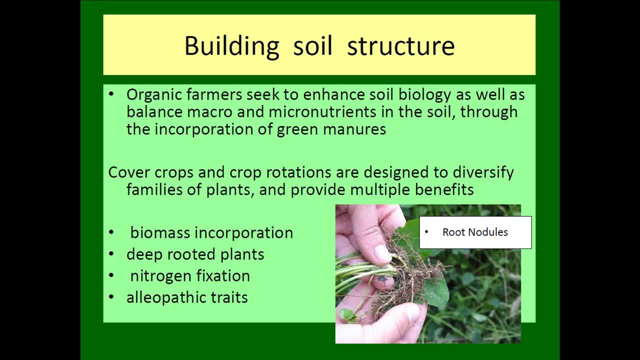 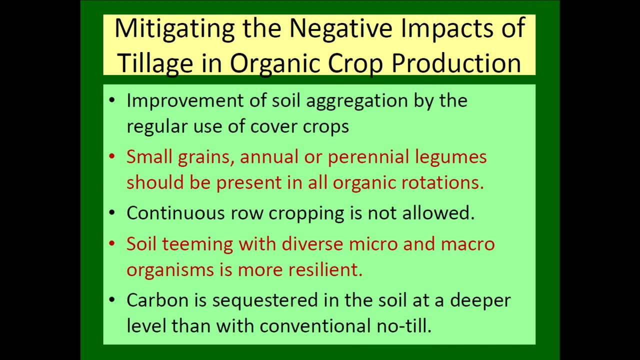 of green manures, ones that are deeply rooted versus shallow rooted ones, that are nitrogen fixing, ones that are have allopathic traits and, of course, those that would have more biomass incorporation. Next slide, next slide, and i know that there's a lot of concern with the nrcs about the negative impacts. 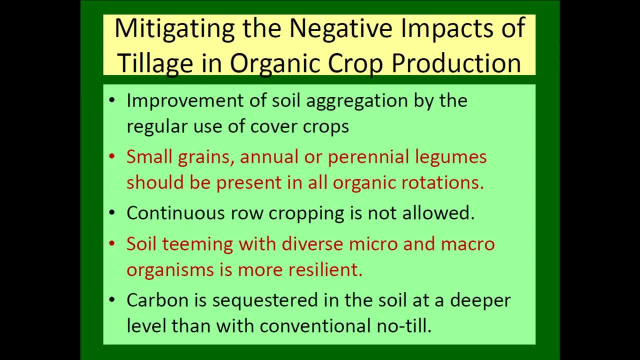 of tillage in organic crop rotation, um, but when the organic producer is is adding these cover crops and brin and incorporating a lot of biomass with living roots, they really are mitigating these negative impacts. of course, you know there will be tillage to incorporate these, but they are adding. 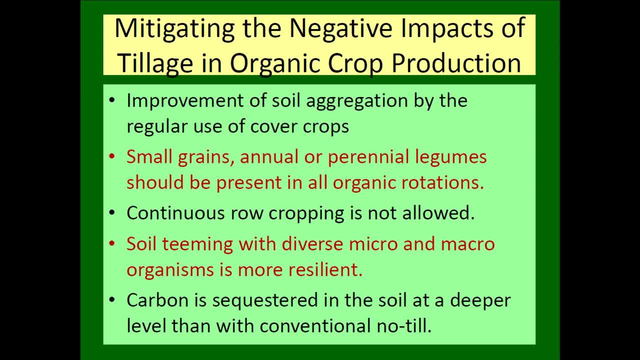 so much organic matter and improving the soil tilt dramatically that this this really does help. the other thing is that, since the organic farmer cannot have continuous row crops, there are only numerous years in the rotation when there is no tillage at all, when they're growing small grains or legumes, and that's even in a horticultural system. there should be at least 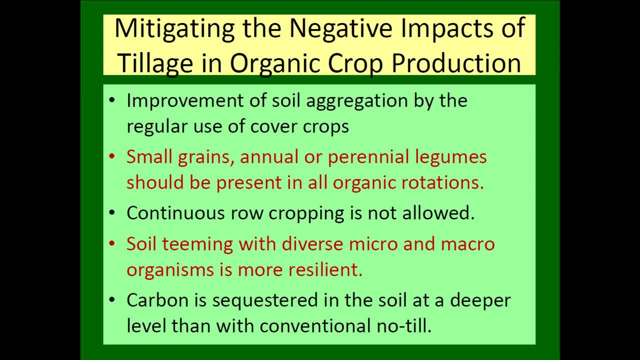 some time. it may not be the entire season, but there could be a breakup the middle of the season or the end of the season, where they are basically putting in a sod crop and letting that soil rest um, and of course there is carbon sequestration going on um at that time. so 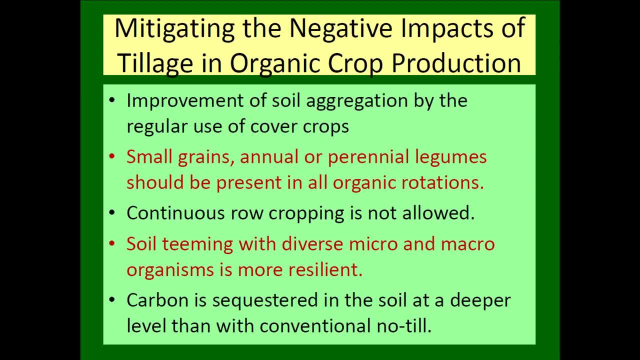 so they're. they're doing a lot of um beneficial activities on an organic farm and typically here in the upper midwest an organic farmer might rotary hoe maybe twice and do that fairly shallow. so they're doing that with two times, sometimes only one where they're actually doing row crop. 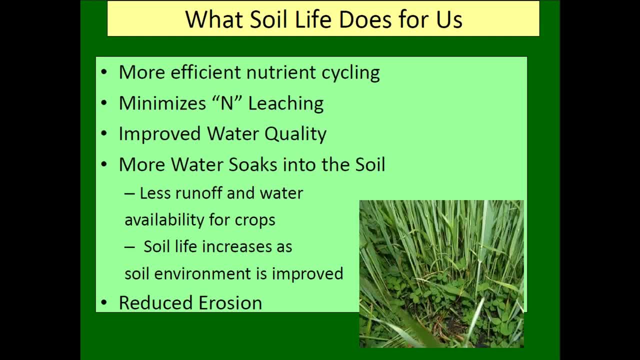 cultivation. next slide and mark. that's up to you. okay, so what does soil life, uh, do for us? in nature, soil life is the entire source of soil, fertility and nutrition for whatever native vegetation is present, the forest, the prairie. life breaks down all of the plant residues, the leaves that fall each year, the annual plants. 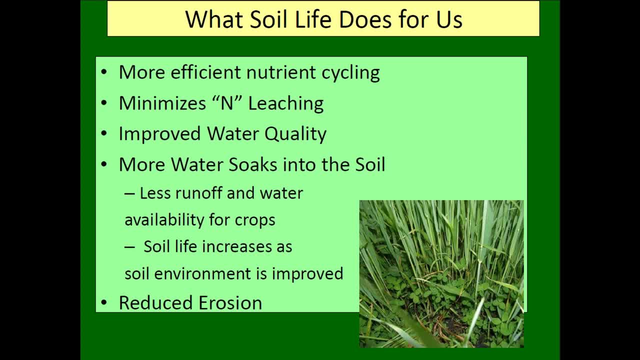 that die the dung from the animals and any dead animals and insects and they basically recycle the nutrients into a plant available form. and they don't do this in the same way that an application of a conventional fertilizer of pouring a large amount of soluble nutrients on at once. instead, there is a gradual release. 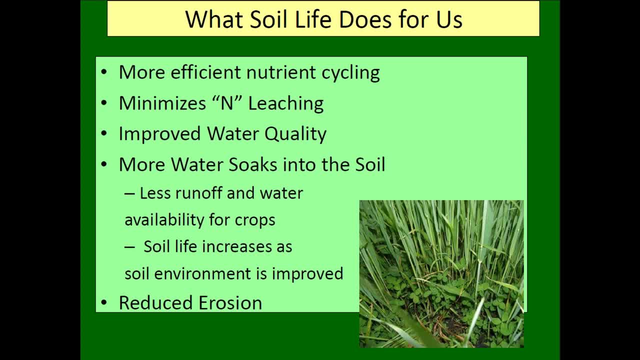 over the course of the year, and they produce a much larger ingredient list in the spring and winter of the season. that is often fairly well in tune with crop needs, and so, in effect, you have a much more efficient nutrient cycling when the crop rotation is designed to simulate as much as practical the natural condition of the 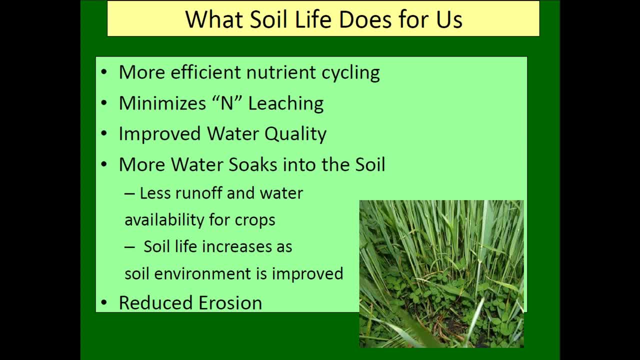 crops and other life residues, regenerating soil fertility. and another thing that happens when you have active soil life, if the soil life is well fed, if you're returning a sufficient quantity and diversity of plant residues to the system and also animal manures, you get a greater diversity and greater. 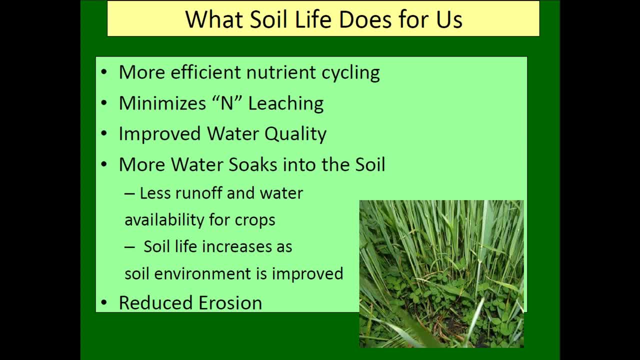 quantity of soil life and the more biological activity in the soil, the less likely you are to lose nutrients through leaching and, in particular, water quality. concern is nitrogen leaching in farming systems, in addition to soluble fertilizers, frequent tillage and intensive cropping, especially when there are bare soil periods while you're. 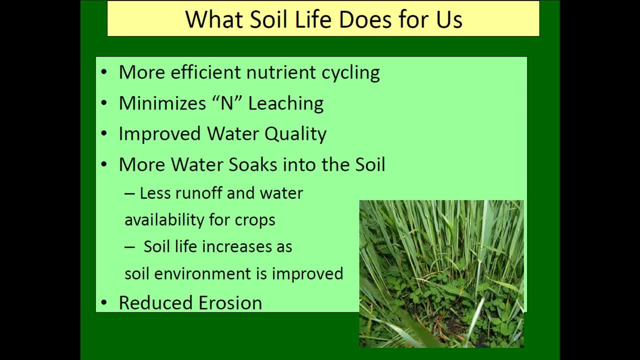 waiting for the soil for the emerging crop to get established. those are vulnerable times for the leaching. however, the more activity you have in the soil, the less risk of leaching will occur. in addition of the soil, life improves the tilt or structure of the soil. in addition of the soil, life improves the tilt or structure of the soil. 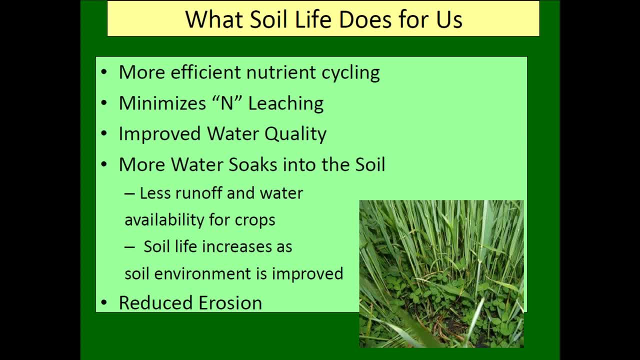 so that crusting is less severe, the soil surface is more open, more moisture can run into the soil. during a rain event, that's runoff and as a result is more availability, water to the crop and another outcome of a biologically active soil is less prone to erosion. now, if you plow such a soil, and on a slope, and it 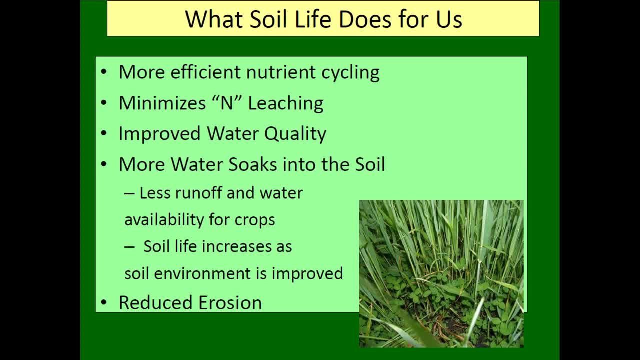 was a heavy rain. yes, it will erode. however, over the course of a well-managed rotation, rotate out. the erosion can be reduced to a minimum by active soil life. another thing that soil life does is the more diversity and abundance and balance you have in the soil food web, the less likely will a 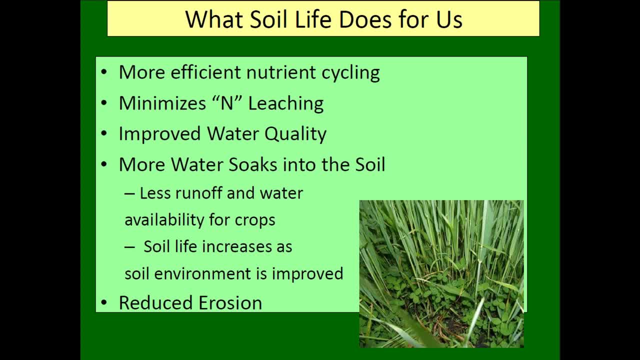 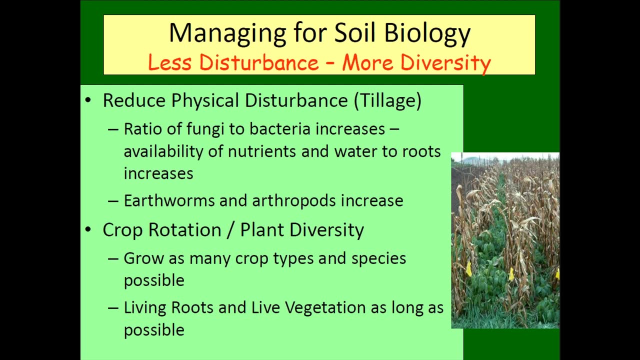 soil borne pathogen. less likely is that a soil borne pathogen will reach population levels that cause a serious amount of crop disease. next slide: okay, there's three things. there's two were spelled out here, but basically there are three strategies that organic growers can use to manage for optimum. 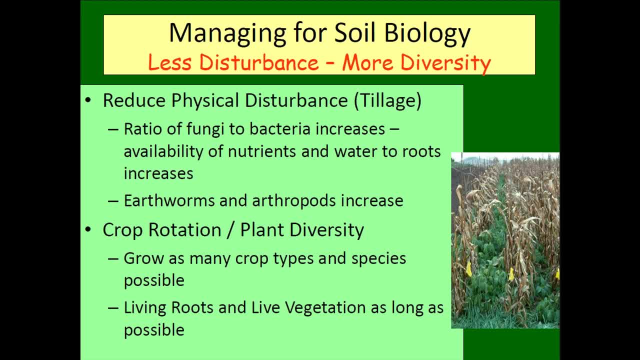 soil biology. one is to reduce tillage when practical. now in an organic system, where herbicides are not are not used because they're not synthetic. herbicides are not permitted and organic plants are not permitted to use organic pesticides by the organic standards, and none of the naturally based herbicides are very practical. 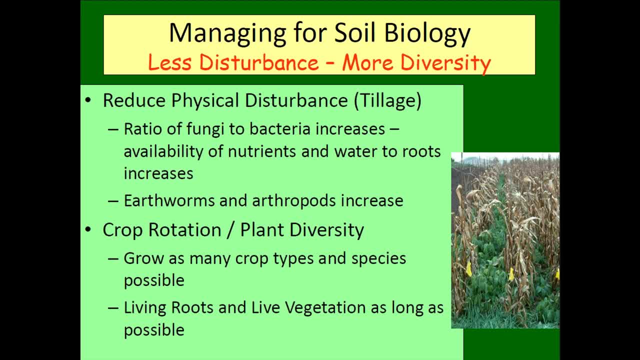 at a field level. Organic growers do depend to some extent on tillage. however, the approach for sustainable organic production is to till only when necessary and to reduce the amount of disturbance of the rotation. When this is done, there'll be more fungi in the soil. get more of a balance between. 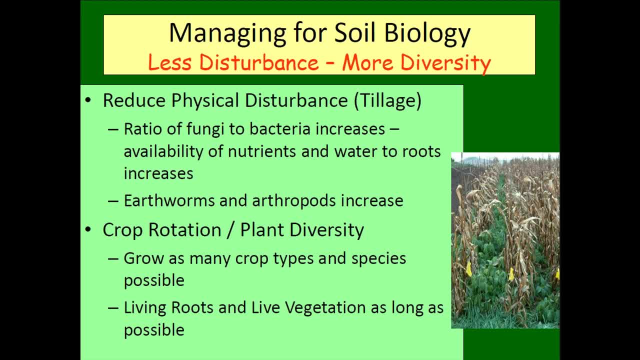 fungi and bacteria, and this really is favorable to most crops and, in particular, the larger organisms that can be physically damaged by the frequent tillage. the earthworms and the small insects and mites will increase as well. The second main approach is through the crop rotation itself, the plant diversity and designing. 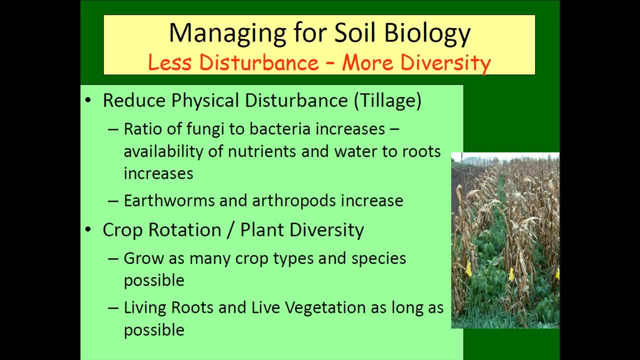 the rotation to maintain living roots and living vegetation for a long time, For as long of the season as possible. And the third aspect that's related to it is, in designing that rotation you try to maximize soil coverage and minimize the periods of bare soil. 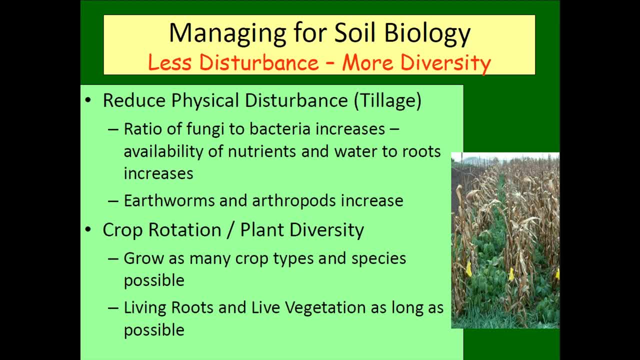 Perfect example here in the photograph, this farmer planted sweet corn and then interplanted. when the corn was established, interplanted those foraged soybeans so that, after the sweet corn was harvested, the only thing being removed were the immature ears. you know, have a tremendous. 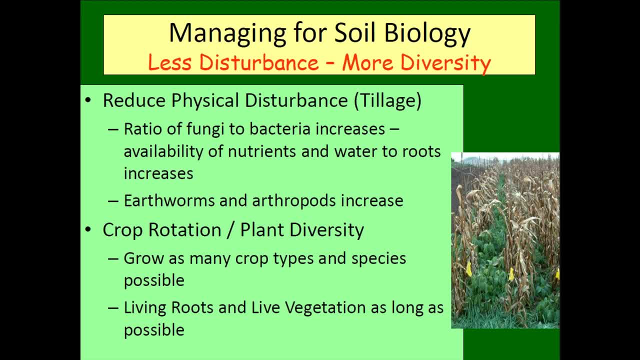 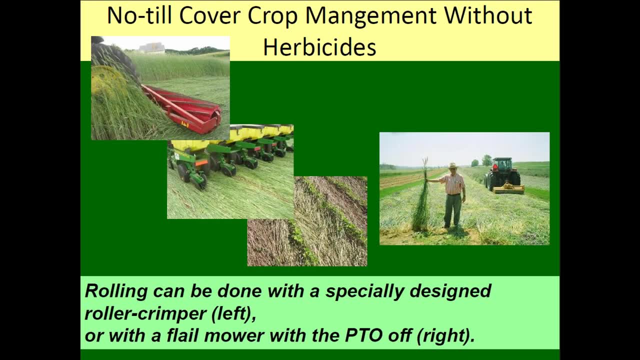 biomass that's ready to grow. And that's what we're trying to do. We're trying to go back to the soil when the frost finally knocked out the soybeans. Next, Next slide, please, Thank you. Thanks to some recent research and development of appropriate tools, organic farmers can. 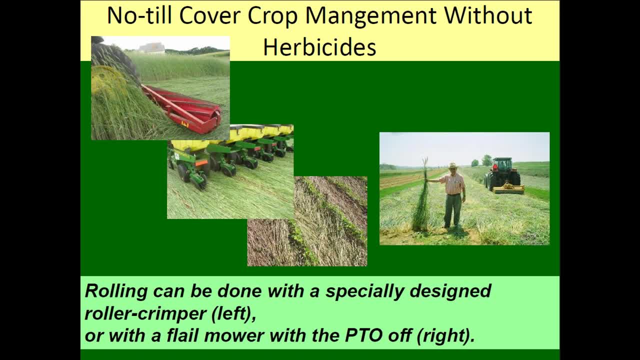 now use no-till methods for at least part of their rotation. although it's not likely that an entire three-year rotation, that every operation could be done No-till because of perennial weed pressure. It is very often practical when a heavy cover crop has been grown to maturity, such as in 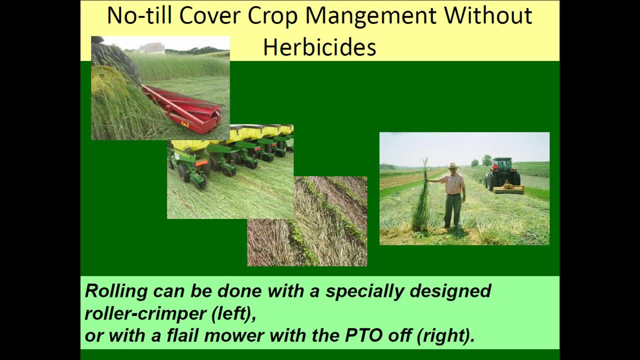 this photograph on the right that's Dr Ron Morse of Virginia Tech holding a strand of rye and veg at full height. It was about six feet tall. It was about three or four tons of biomass per acre. in that field They're using a flail mower with the power takeoff turned off so that it acts as a flail. 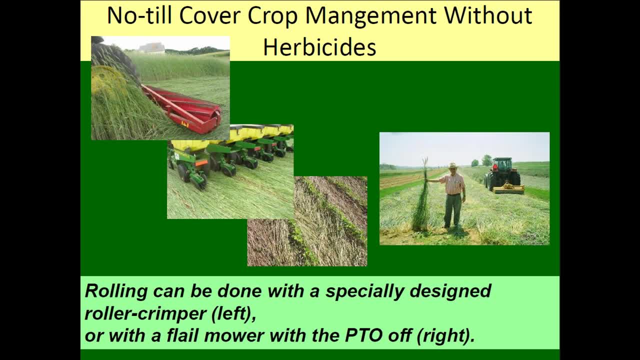 mower And it's knocking down that cover crop. In recent years, roller crimpers have been developed specifically for no-till management of cover crops without the use of herbicides. Upper left-hand picture And then a no-till planter can be used in that very uniformly oriented and roll crimped. 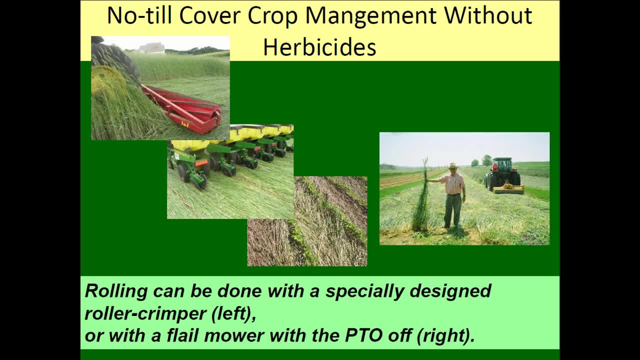 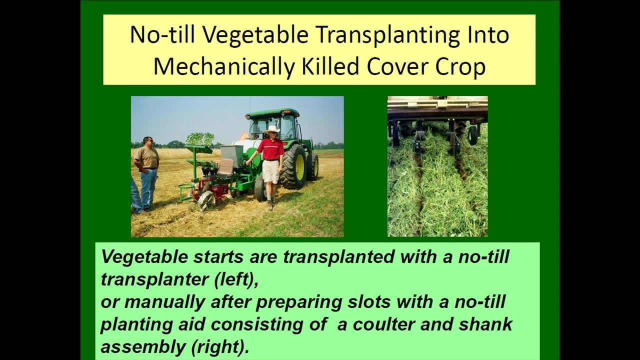 cover crop residue to establish the next production crop, Next slide. Here's an example with horticultural production in a rolled wheat cover crop on the left. It was rolled a couple weeks earlier, so it's died out. It's turned brown. 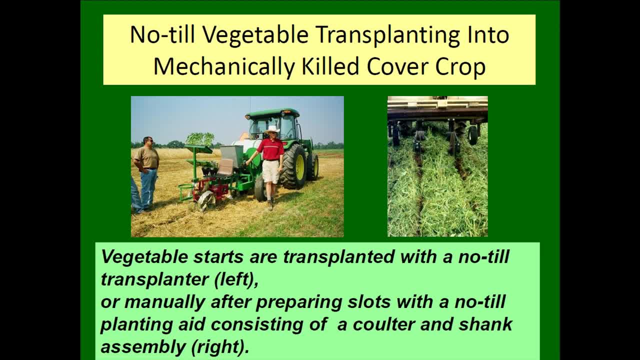 They are now using this no-till transplanter to create a part of the mulch, create a narrow slot in the soil and set the pepper plants all in one path And on the right For a much larger crop. For a much lesser capital investment, a farmer can buy or build a no-till planting aid which 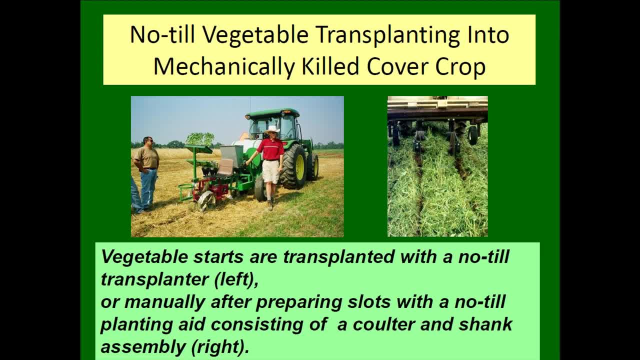 is simply a coulter and shank to create the slot in which either a conventional planter or a manual planting method can be used to establish the crop. This is very effective for transplanted and large seeded vegetable crops such as potato and garlic, and even beans, squash and sweet corn. 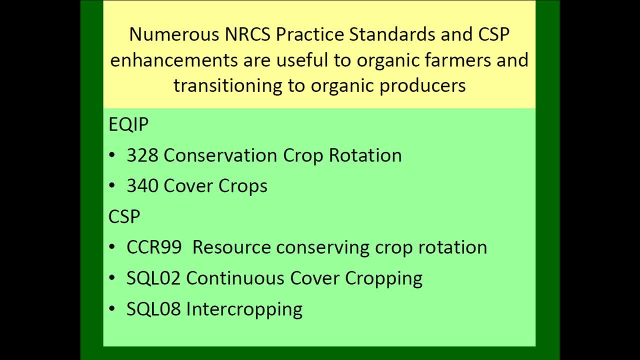 Next, Slide 10.. And there are several practice standards that the NRCS offers that relate to this. This is here the conservation crop rotation that was mentioned earlier: Cover crops- I just wanted to emphasize cover crops- are an especially important part of crop rotation. 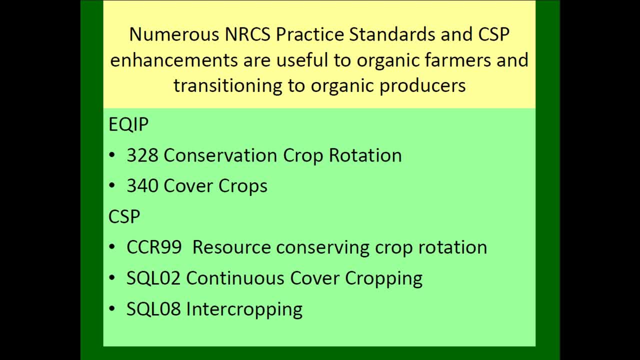 in organic systems because they perform so many different services. They replenish the soil with, like N6 nitrogen, which we'll talk about more in a little bit, And they're also playing an important role in the soil- Slide 11.. They play important roles in weed and pest management. 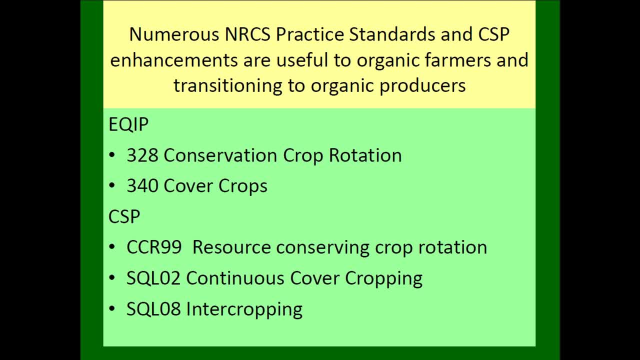 And, of course, the presence of a living cover crop protects against erosion On a sloping field. another EQIP practice that's not listed here is code 585, strip cropping. It's basically a conservation crop rotation arranged in relatively narrow strips where 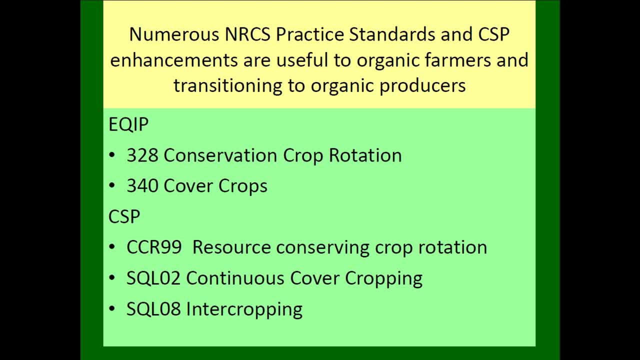 the different phases of the rotation alternate with each other And this provides enhanced benefits in terms of bringing unlike plant-based crop rotation- Slide 12.. The NRCS provides enhanced benefits in terms of bringing unlike plant-based crop rotation- Slide 13.. The NRCS provides enhanced benefits in terms of bringing unlike plant-based crop rotation. Slide 14.. The NRCS provides enhanced benefits in terms of bringing unlike plant-based crop rotation- Slide 15.. The NRCS provides enhanced benefits in terms of bringing unlike plant-based crop rotation- Slide 16.. npc- dois, like in clay class plantブ, such asさい, is offered toования plants and plants. 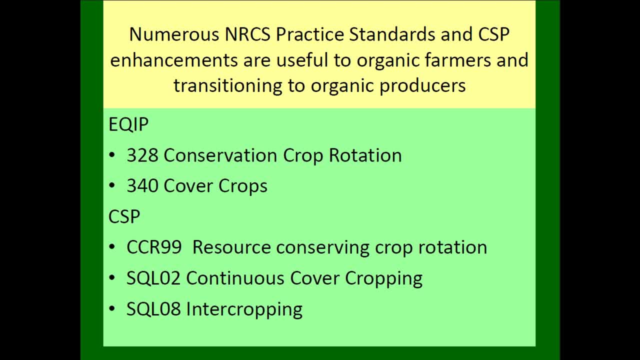 plants, even if the plant is análcological, which means that if plants are enclosed close together, in close proximity, and this can slow down the spread of diseases and provide habitat for beneficial insects- Slide 17.. The NRCS provides enhanced benefits in terms of bringing like n6 nitrogen. like n6 nitrogen. 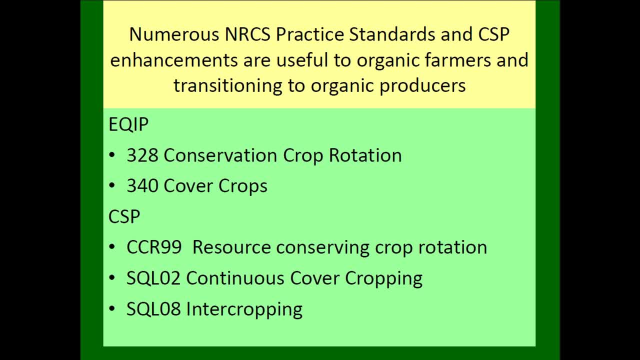 and none nitrogen until the soil is completely polluted- Slide 18.. admitted weed and pest management- Slide 19. United Bipełanctер cár�esen inJ. Slide 20.. As soon as one production crop is finished, the next crop- either a production or a cover. 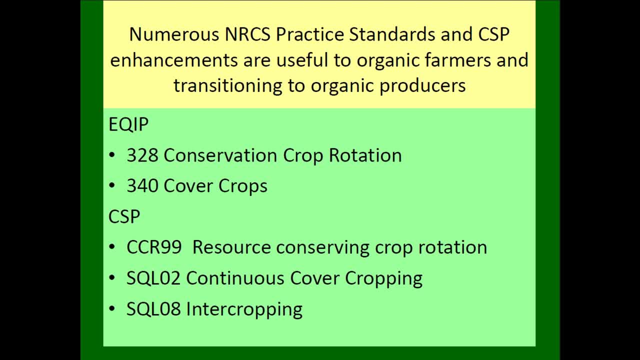 crop is planted, And this particular practice must include at least one cover crop every year and no extended fallow Intercropping, which I will show you an excellent example of relay intercropping in a few slides. that's basically planting two unlike crops in alternating rows or narrow swaths with 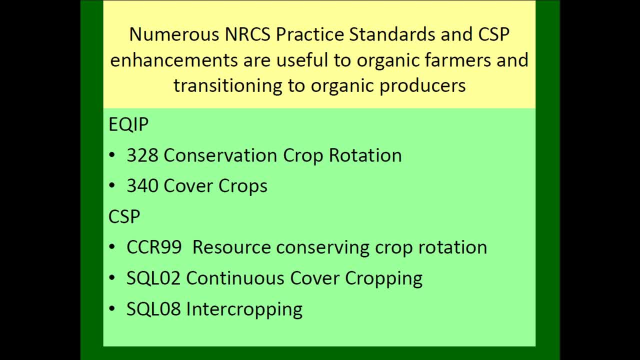 each other again, offering the potential for beneficial habitat, pest control as well as maximum use of the soil. And right, that sounds like okay. we're drawing down the soil's nutritional resources, etc. and working it harder. It's also keeping it covered more completely. 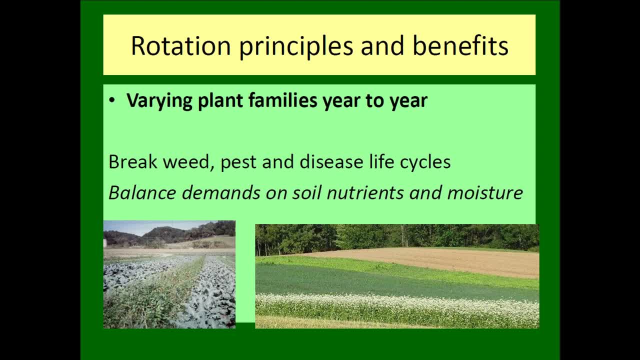 Next, Okay, a few principles and benefits and rotations. One is to vary the plant families year after year, so that on the left you see there's a broccoli crop in the alternate beds there, and so the next season we would not plant anything in those beds that are in the Brassica or Crucifer family. 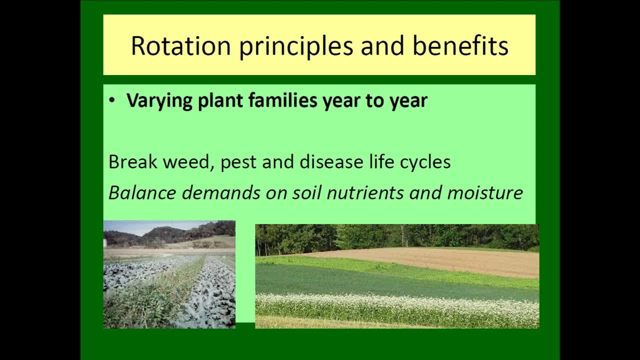 Like we would not go into a cover crop radish, or into arugula or mustard salad greens. We would go into a different plant family, such as a cereal grain cover crop, like you know, or a tomato family. On the right hand you see several strips of alternating different crop families as 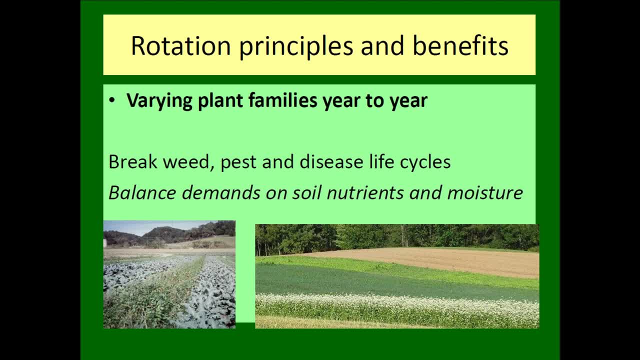 a buckwheat cover crop. It is hard to see from here, but it looks like there is some kind of an agronomic crop and then an actual sod, And what the alternating of plant families does is primarily the first thing it does. 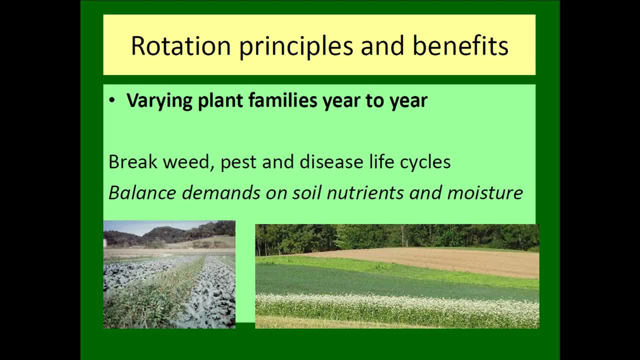 is to break up weed pests and disease life cycles. Most pests and diseases that we see in the plant family. they're not the same. They're not the same. Most diseases attack specific plant families. like a cabbage root maggot will attack broccoli. 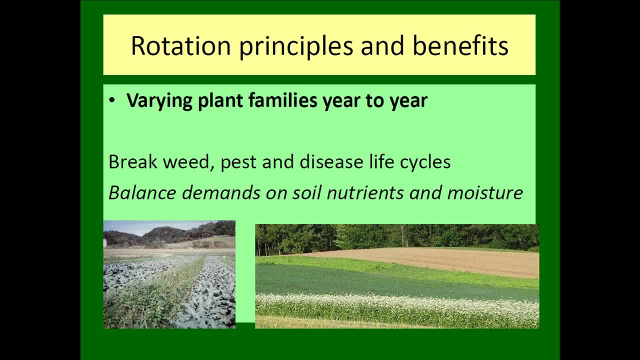 it will attack arugula, but it won't do anything to buckwheat. So if you go into buckwheat and you go into a cereal grain after that broccoli, you will not have a buildup of that maggot. In addition, in a diverse rotation you are often shifting the timing of planting and 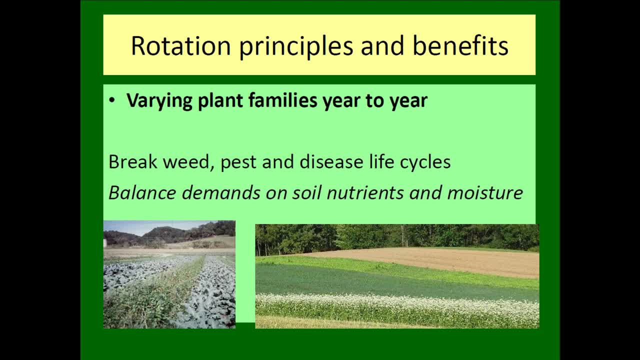 any tillage that is done and other field operations So that the times of soil disturbance and the short periods of exposed soil or plants that are being established occur at different times of the year And that helps break up weed life cycles because particular weed species will come. 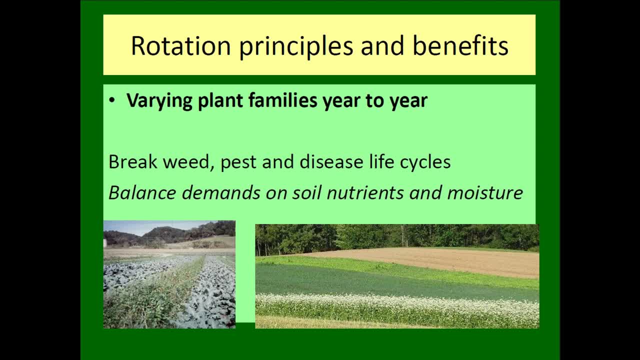 up at a certain time of year. In addition, this balances demands on soil nutrients and moisture. The broccoli is a moderately shallow-rooted, very heavy nitrogen-feeding crop. The buckwheat is shallow-rooted but it's a very light feeder and it tends to make. 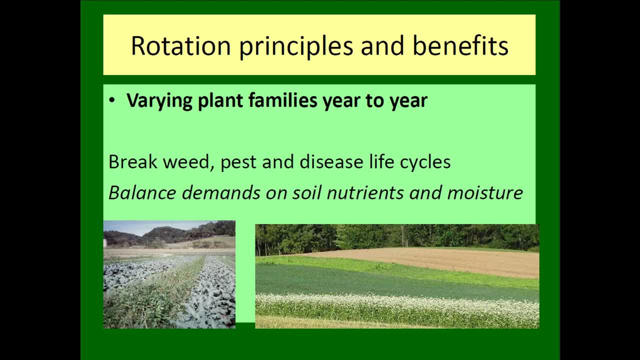 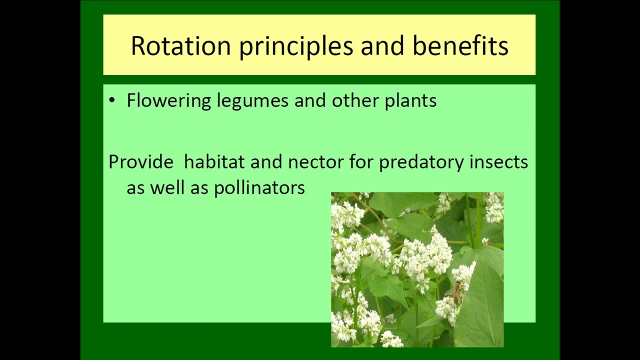 phosphorus more available in the soil. You get into a legume like sweet clover. it's very deep-rooted, it will be taking moisture from a much greater depth and it will also be fixing nitrogen. Another advantage of a very diversified rotation is if you can include flowering plants, particularly. 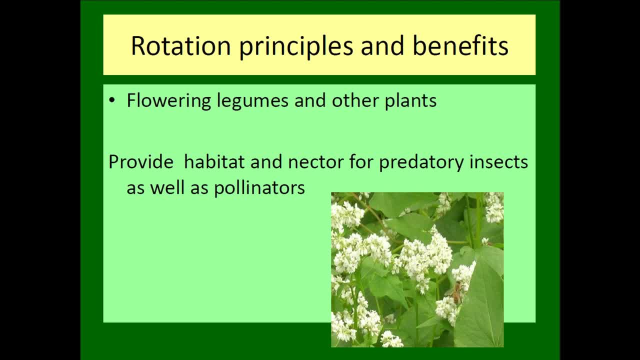 legumes, buckwheat and anything with relatively shallow flowers with accessible nectar. these are important habitat and food sources for both pollinators and for predatory insects and parasitoids that will control insect pests. Many of the parasitoids, the adult phase, is a very tiny wasp or fly that you will hardly. 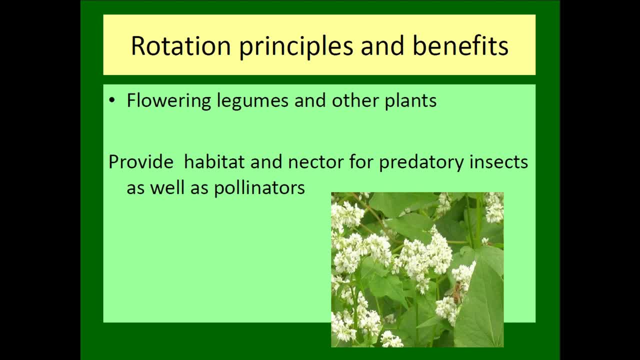 notice, You'll think you see gnats flying around your cut flowers. A lot of those are the adult phases of beneficial insects that will then go into the vegetable crops nearby or agronomic crops later. So that's a big advantage. Lay eggs on certain pests. they're very specific. they'll lay eggs on the pest and that pest. 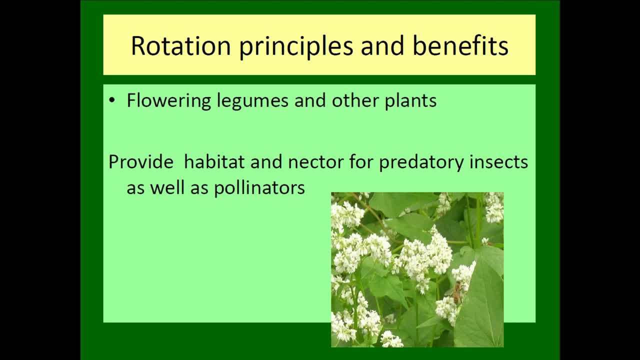 will be able to complete its life cycle and multiply. One thing that horticultural growers often can do, and often do, is diversify from just vegetables into cut flowers, and a lot of those cut flowers, like zinnias and sunflowers, are excellent nectar and habitat. 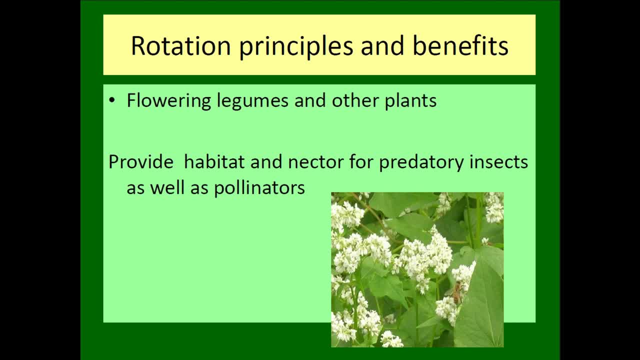 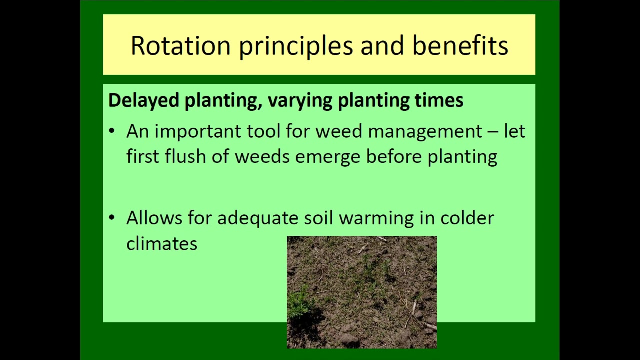 Also cover crops. letting cover crops come into flower, which is also recommended for getting maximum Biomats and nitrogen fixation, and also they must flower to be able to be killed by roll crimping Those flowering cover crops. many of them are also excellent nectar sources. 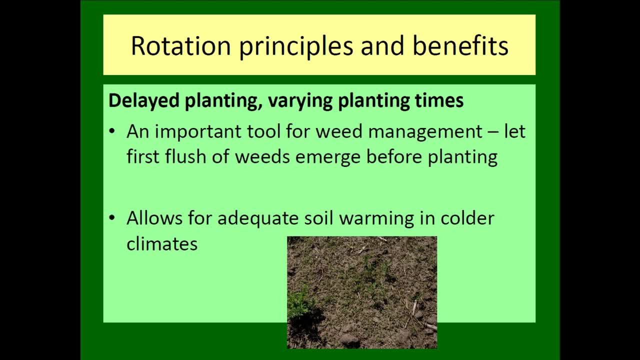 Another strategy that organic growers will use in designing their rotation is to delay the planting time for certain crops beyond the earliest possible time. That's what we're going to do. That's what we're going to do. We're going to try to keep the plant as fresh as possible. 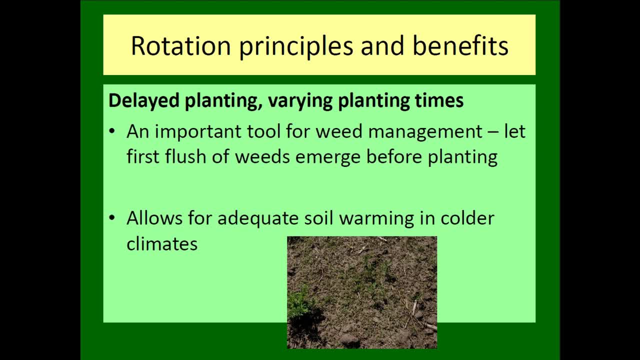 We're going to try to put them in their natural habitat so that they have a climate of their own, so that they can grow a little bit more quickly and that they can be planted in their natural habitat. We're just going to give them a couple of weeks to get them ready to plant and be ready. 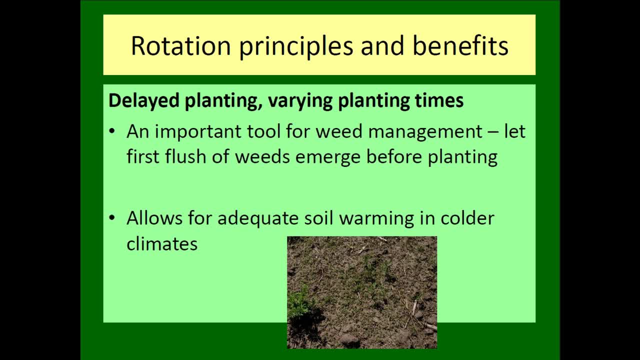 to plant again. One of these, one variant of this practice is to prepare the seed bed at the normal time but then wait a couple of weeks, just long enough for the weed seed banks to all germinate. Then, when they're very, very tiny, like you see in this picture, the grower will go through. 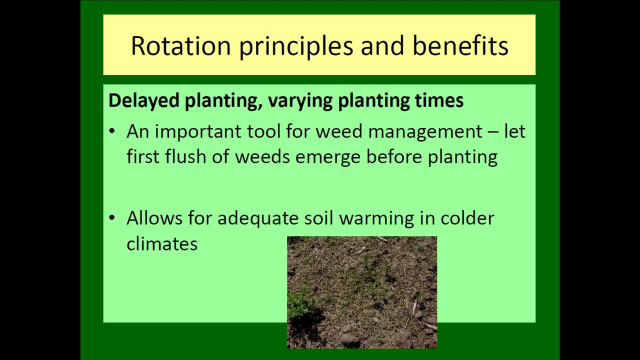 either with a flame weeder or the very, very shallow cultivation that does only a minimal amount of soil disturbance, and clean up those weeds and then immediately plant. This shortage is not an option in our data or we'll go through either with a flame weeder or the very, very shallow cultivation that does only a minimal amount of soil disturbance. 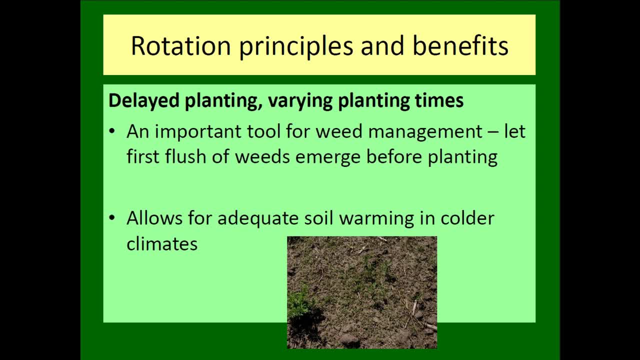 and clean up those weeds and then immediately plant This short bare soil fallow. in addition to allowing the removal of many weeds, will also allow the soil to warm up some more, And this can be important in colder climates. Another thing that has been found is when the crop is planted at a time where soil temperature will favor its rapid emergence. 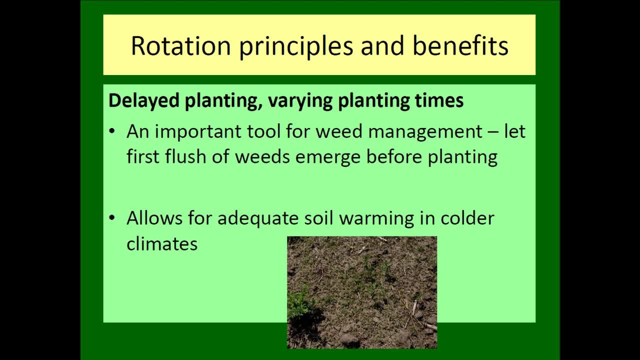 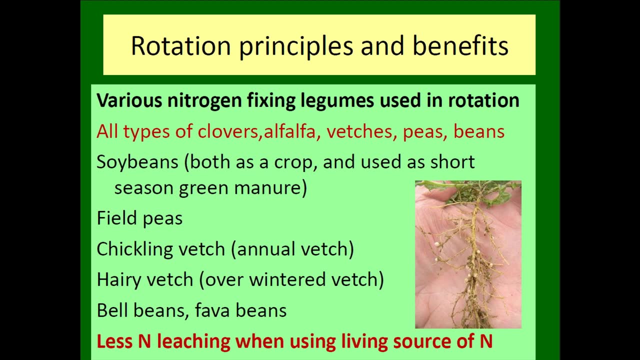 is that the crop is vulnerable to weed pressure only for a short time, So that can reduce the frequency and intensity of cultivation required after planting. Next slide: Legumes, which fix nitrogen from the air and can provide up to two hundred pounds, and very often at least one hundred pounds per acre of nitrogen. 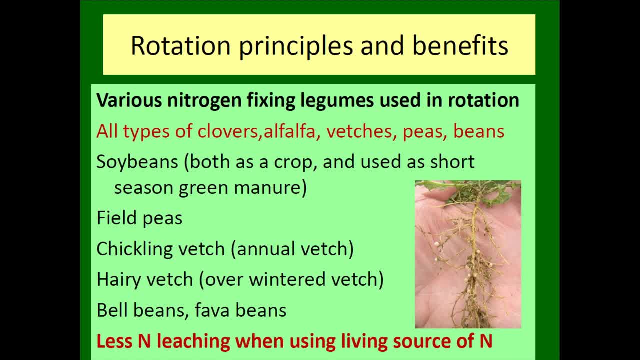 is exceedingly important for organic production systems because, by not using soluble synthetic nitrogen, organic growers do face the challenge of how to get sufficient nitrogen to their crops, especially very heavy feeding crops like corn or broccoli or some of the other greens, brassicas in particular. 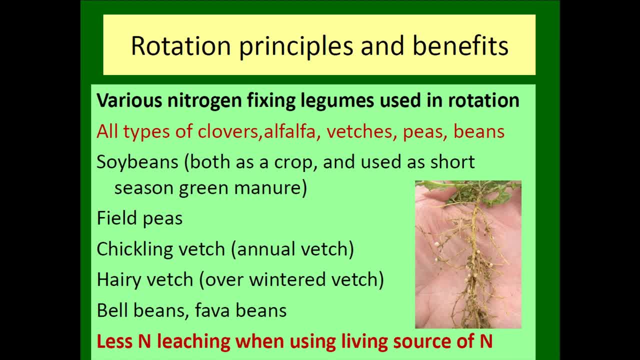 And what the legumes do is they fix this large quantity of nitrogen from the atmosphere. About half of it will become available to the succeeding crop, And the other half, however, is not lost. Instead, it becomes part of the soil: organic matter. 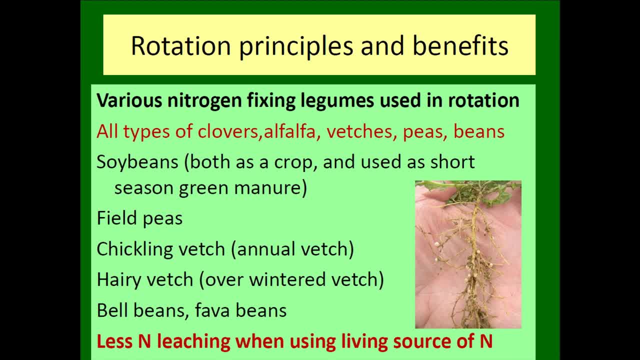 And soil biologically active. high organic matter soils will all of their own release nitrogen- About a hundred pounds or more of nitrogen per acre annually- just through nitrogen mineralization. So the organic grower's job is not to supply the crop directly with all of its nitrogen needs. 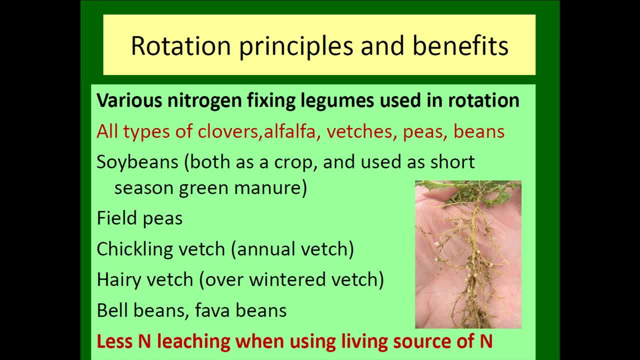 which might be between one and two hundred pounds per acre, but to provide, to replenish the soil so that the process of mineralization does not draw the soil down over time. So legumes play a vital role in this. Here's some examples of legumes: 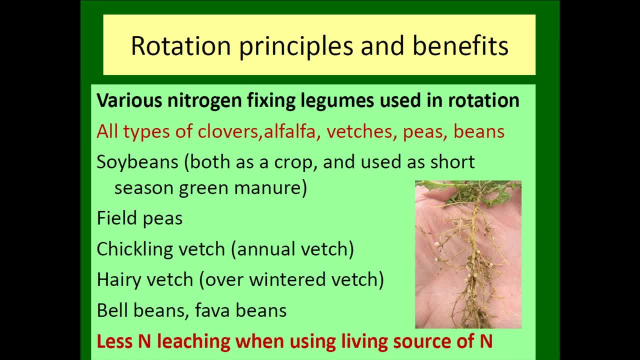 Here are clovers, alfalfa, soybeans, which is a warm season cover crop, Field peas, including Austrian winter field pea, cooler season. The Austrian winter will overwinter. zone six and south Chickling vetch is a summer annual vetch. 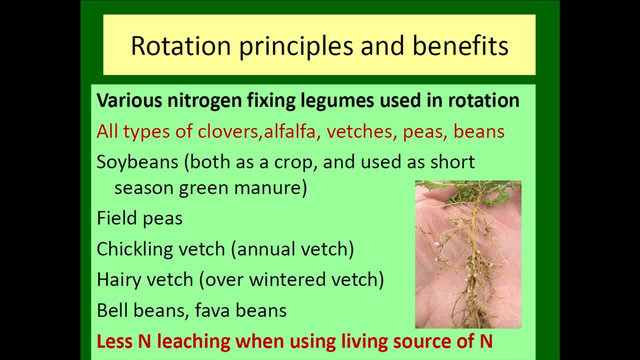 Hairy vetch is a very hardy winter vetch. Bell beans and fava beans are related to vetch, but their frost kills at about 20 degrees. They're either a winter cover crop in the south or a Spring cover crop in the north. 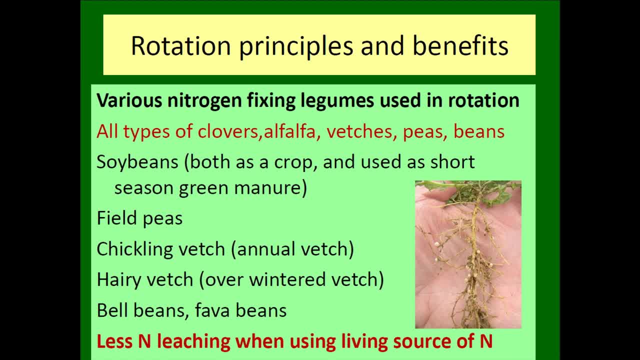 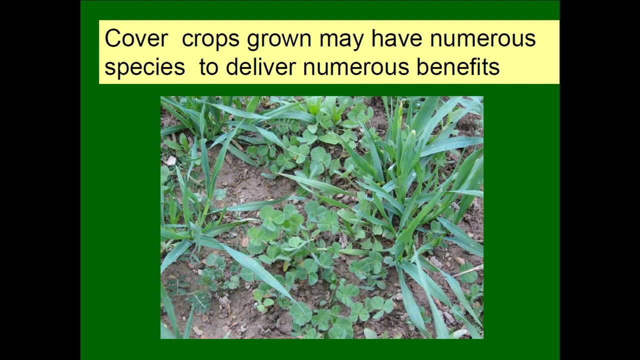 Generally, when legumes are used and legume cover crop nitrogen is used, there's less risk of nitrogen leaching than with synthetic nitrogen or raw manure. Next slide. One thing that is being done more and more often is growing combinations of two or more species of cover crops. 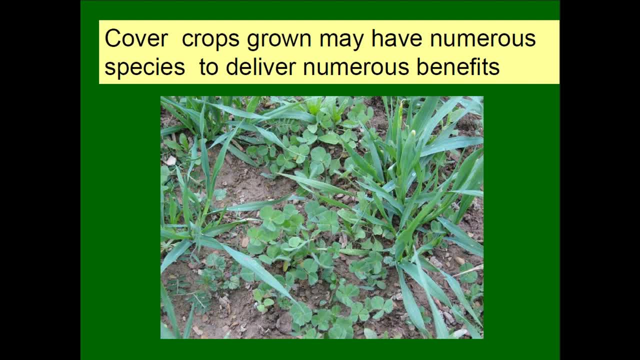 to get multiple benefits. This photograph shows a winter grain clover mixture, which is very commonly grown to produce nitrogen. There are three species here. there's some veg growing there as well, And in recent years farmers and NRCS personnel have been experimenting with much higher levels. 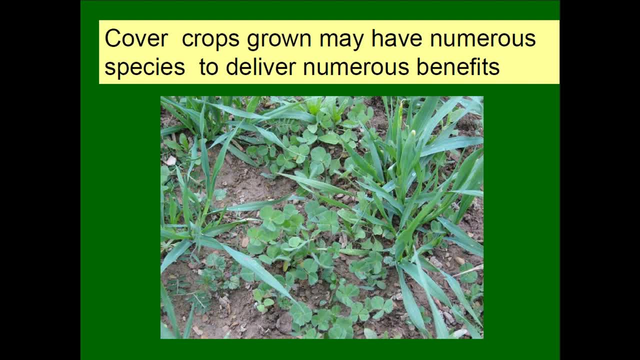 of diversity of cover crops to widen the range of benefits, including plants from several different plant families. This will increase the biomass, will diversify the benefits to the soil life, and that's one thing. The more different species of plants growing together or in the tight rotation, the wider 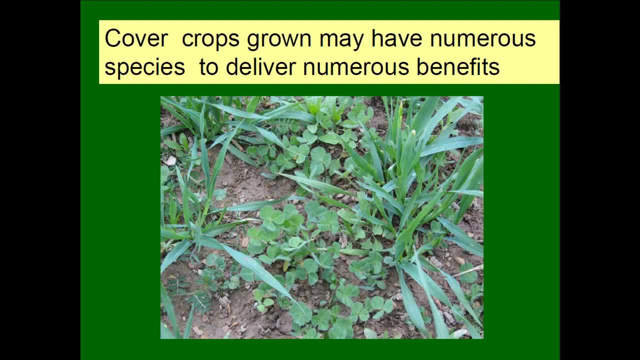 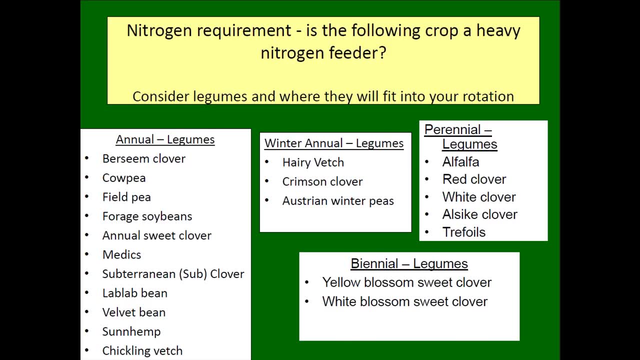 the diversity of soil organisms will be supported. Okay, next slide, Just a larger list of legumes. the challenge in a crop rotation, particularly a tight crop rotation, where a farmer, a vegetable producer, is growing produce on relative limited acreage with a very complex rotation, is how to fit the legumes into the production windows. 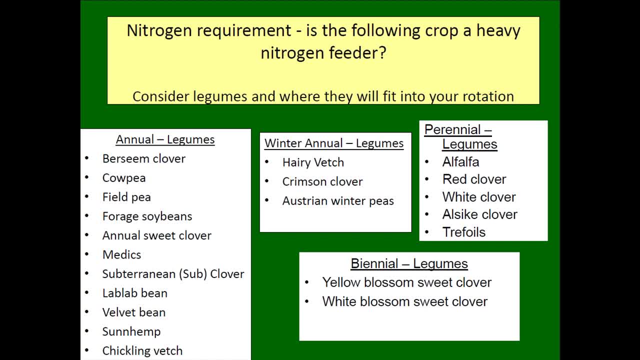 So there are summer annual legumes, winter annual legumes, Perennials for rotating a field out of intensive annual production into one to three years under a perennial sod. combining these with the grass is a very good way to rest the soil. 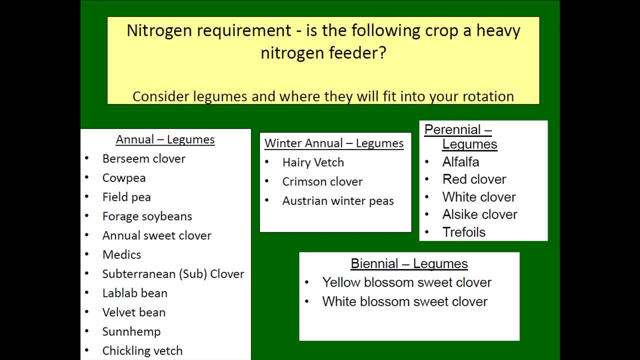 And then the biennial legumes are very. the sweet clovers have a very deep tap root and they're very excellent for breaking hard pan bio-drilling In a situation where you have a lot of production grass that is in rotation and cannot use the. 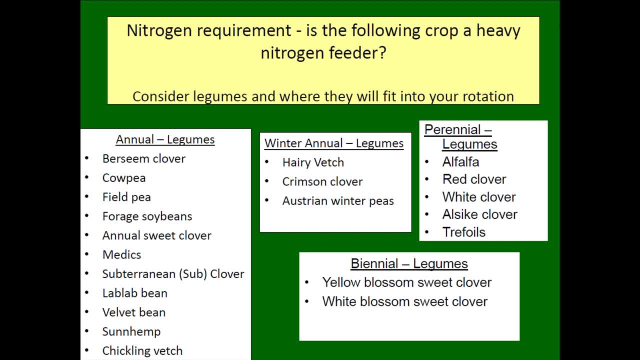 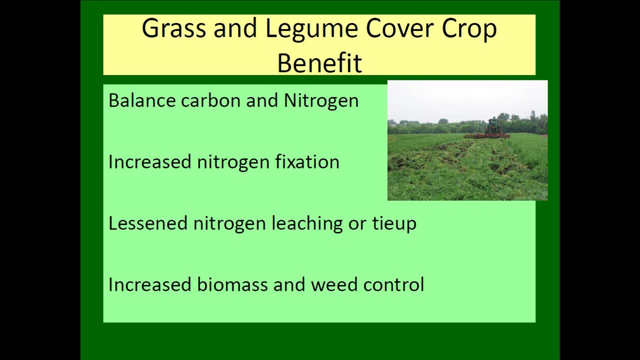 tillage radish because of rotation plant family concerns. the sweet clovers are very useful. Okay, next, One thing that is very often done and is very beneficial is to grow the legume cover crop with a grass. This essentially provides a balanced diet for the soil life, because soil organisms like 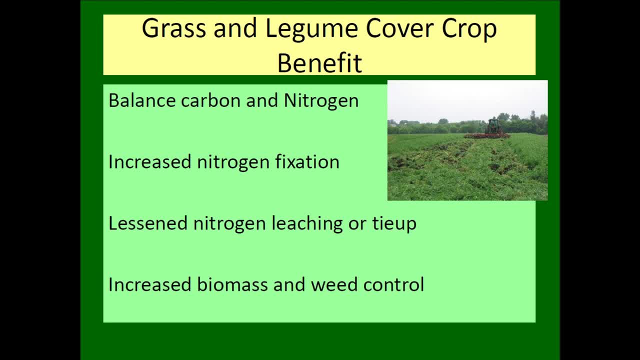 all life require both carbon and nitrogen as well as other nutrients, And the carbon and nitrogen should be in a balance of about 30 parts carbon to one part nitrogen. If you were to grow a cover crop of just rye and then roll that down, or especially if it's 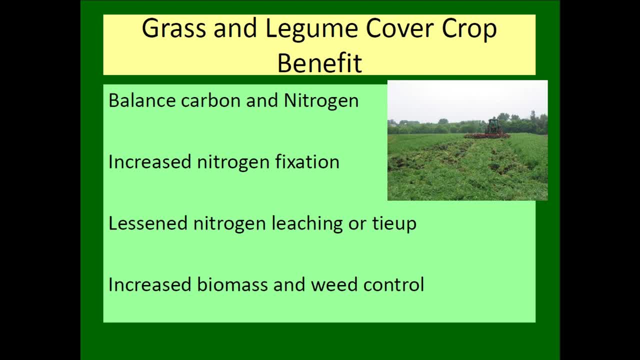 tilled in, you will have such a high level of carbon that it will tie up nitrogen. If you were to grow just hairy vetch, the nitrogen concentrations in that vetch tissue when it's turned under is so high that some of that nitrogen could leach away before the following. 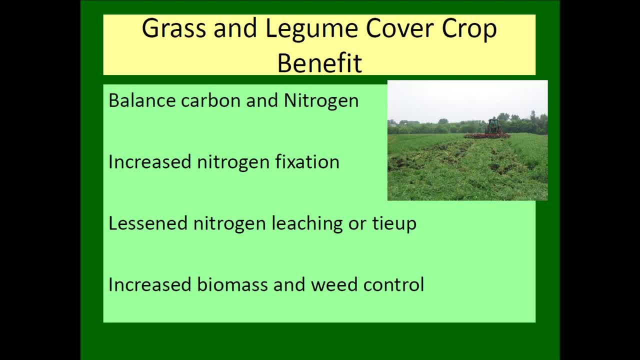 crop takes it up. However, if you have a rye plus vetch cover crop, the nitrogen input is going to be balanced. In addition, if you look at an all-rye field, look straight down from above, you can see. 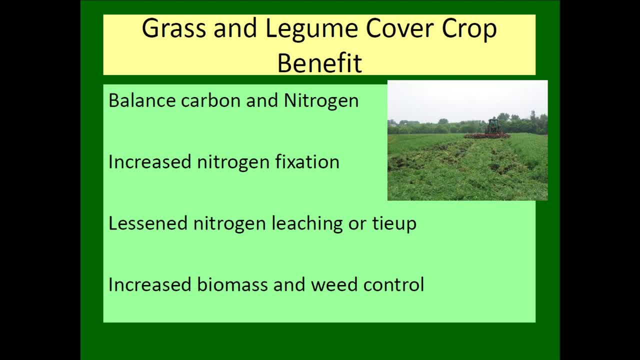 down to the soil surface unless it's an extremely heavy cover and there will be some weeds growing down there. If you have just vetch, it's just lying at the low mat and it may actually kind of smother its own growth to some extent and some weeds can break through. 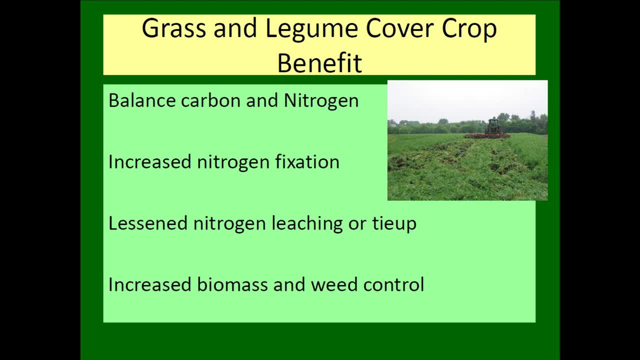 If you have the rye and vetch together, the rye is supporting the vetch and you'll get a much more complete soil coverage. This is also true for summer combinations like sorghum, sudangrass and cowpea. 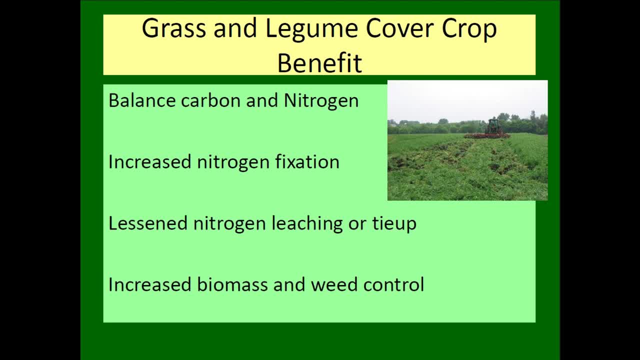 So what happens is you have enhanced biomass and weed control, And another thing is that researchers have found that if you plant a legume by itself, it will actually not fix as much nitrogen as if that legume was growing with a grass. The reason is that when the legume is planted by itself, it will use available soil nitrogen. 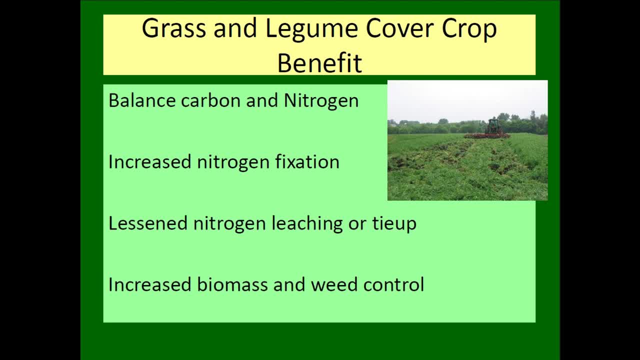 until that is used up and then it will begin to fix the nitrogen. However, if there is a grass like rye or sorghum sudangrass that's rapidly taking up all available soluble soil nitrogen, the legume will be stimulated to fix at its maximum rate. 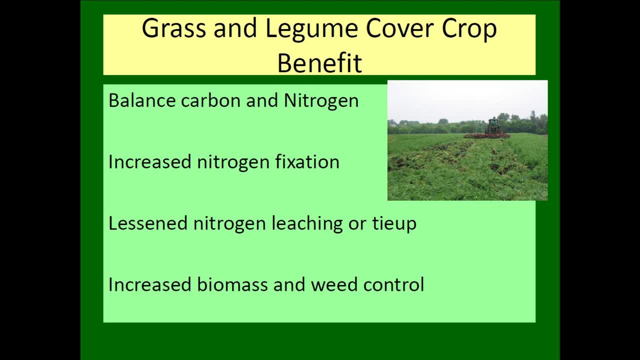 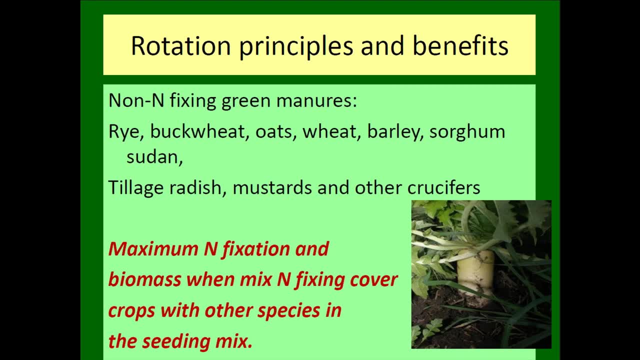 So you actually get an increase in nitrogen gain as well as by-products Next. So this has some examples of some other green manures that are not legumes. As I mentioned, the rye, oats, wheat barley and sorghum sudangrass are good grasses to. 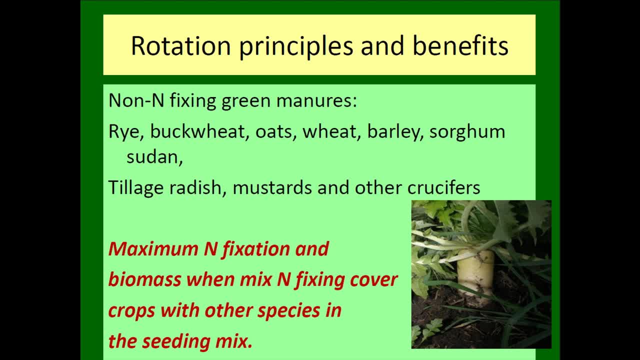 combine with legumes. There's also several species of millet that can be grown in the summer, either alone or with the cowpea or soybean. Buckwheat is very useful for a short fowl. during the frost-free period, It can very rapidly form a canopy and choke out weeds, and it will actually reach maturity. 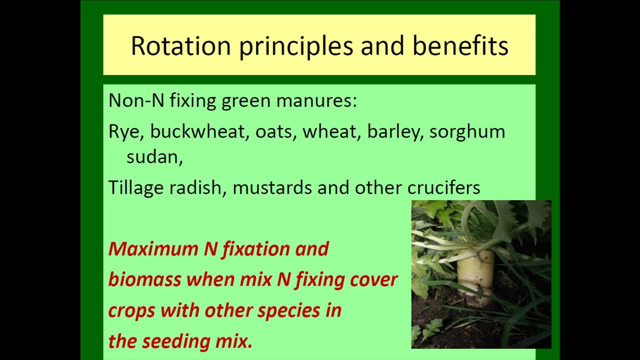 in 30 to 40 days. So that's very handy, Like if you have a rotation of spring lettuce and then you're going into a late summer or fall planting of another vegetable and you have a gap there of about four to six weeks. 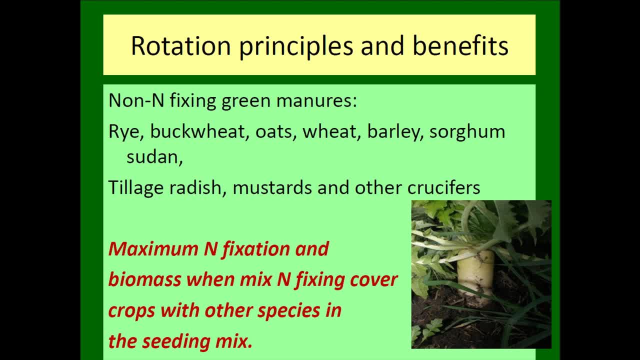 that's an excellent choice. Other non-legumes that are valuable are in the Cruciferobrassica family. These include the tillage radish that's shown here in the lower right. It's basically a daikon radish That's been selected for optimal cover crop properties. 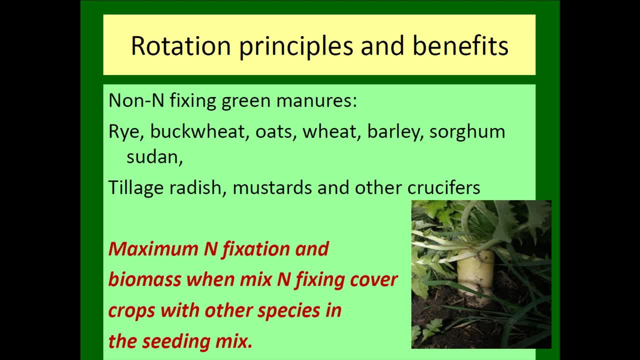 That deep root, that heavy tap root, goes down a foot or two below the surface and then there's a fine tap root that goes several feet down. It's often called biological tillage or bio-drilling. That can really help to relieve hard pan and avoid the necessity of deep tillage with an 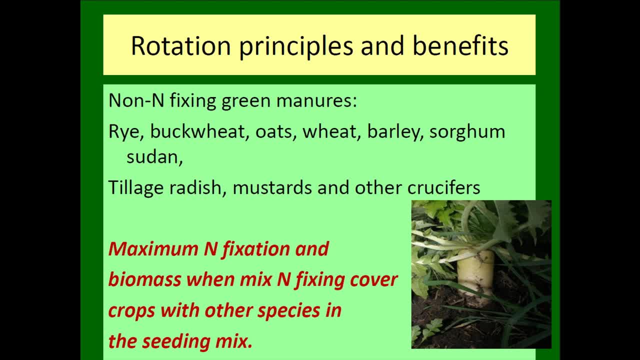 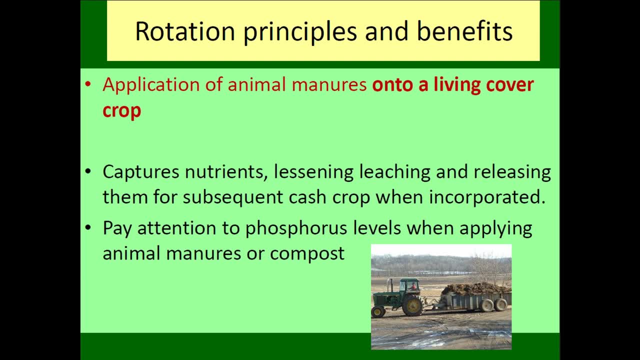 implement. So next slide. Another option that cover crops offer is how to manage manure, especially on a farm where you have both livestock and crops, or if you have a nearby source of manure and that's the most affordable way to obtain nutrients. 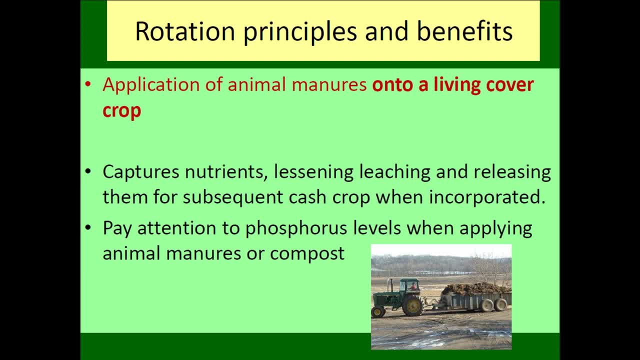 For example, if you have a soil that's testing very low in phosphorus and it would be very beneficial to bring phosphorus to the soil If you have a soil that's on in the form of this abundant manure resource, as you can. 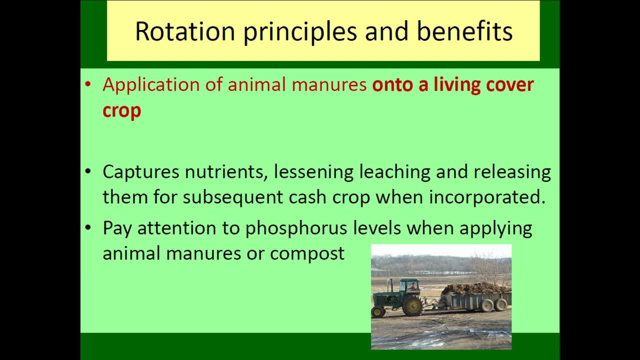 see from this photo, there are some hazards with spreading raw manure in the field. when it's bare, It could very easily run off or leach into nearby water sources. Another concern under the organic standards and just for food safety in general, is you. 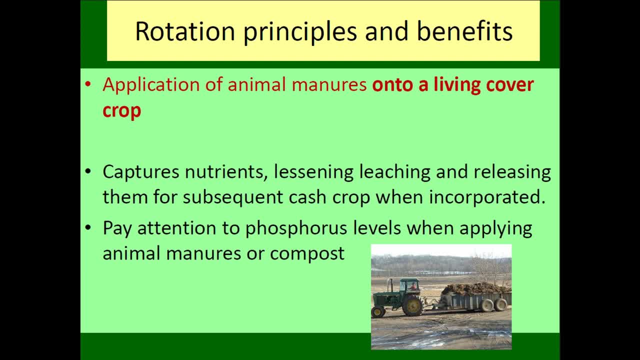 want at least 120 days before an application and incorporation of an animal manure and harvest of the next organic food crop, especially important for food safety around vegetables that are eaten raw or that are grown in or in close contact with the ground. So one thing you can do with a high crop rotation that includes cover crops is to spread. 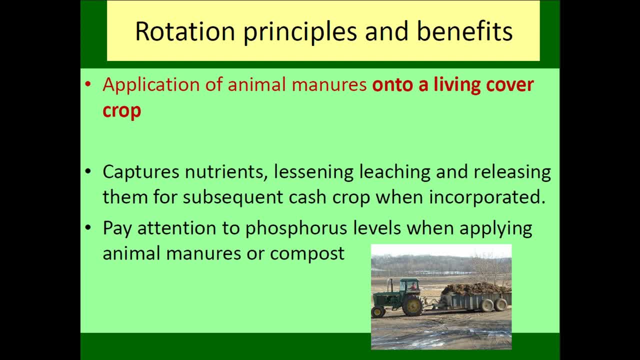 that manure on a cover crop or if your rotation includes forage crops- like you've been cultivating vegetables intensively for a couple of years- You rotate it to a forage- you could apply the manure to that forage and that could. 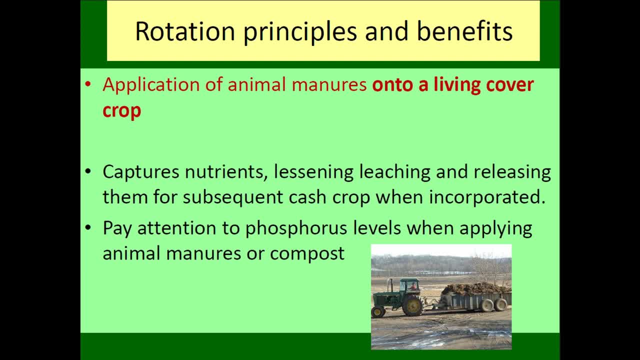 be a perennial grass or grass-like young combination, And the living plants will take up the manure, the manure nutrients, so that they do not pollute the water resources. An excellent crop for this is sorghum sudangrass. 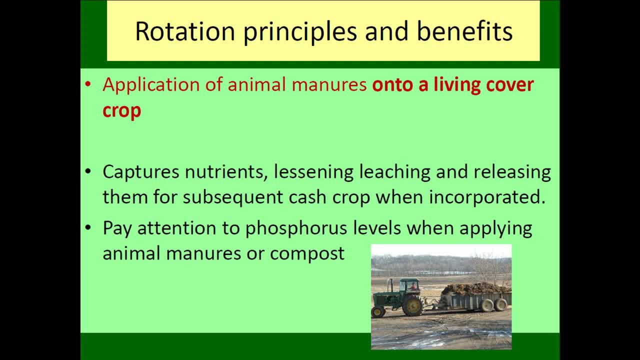 If you go out there when it's just starting its rapid growth and spread some manure or chicken litter, it's going to take up a lot of water. It's going to take up and hold all those nutrients and then return it in a much less. 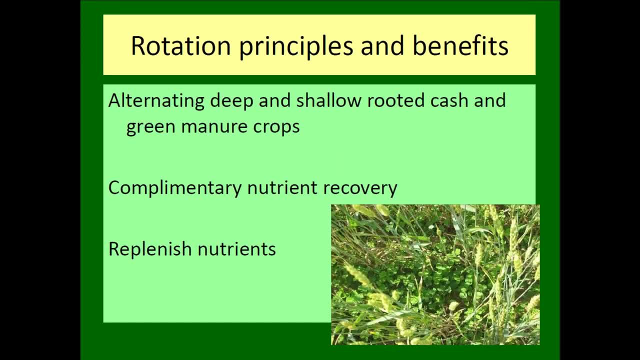 leachable form. Next, One thing I should have mentioned in that last slide is that organic farmers do need to pay attention to their soil phosphorus levels, because if you depend too much on compost and manure as your source of N, P and K, these materials tend to provide more phosphorus. 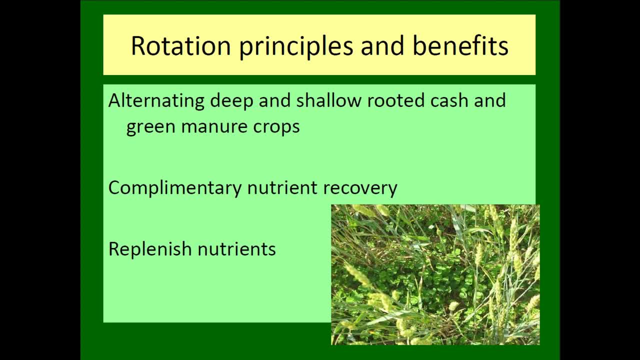 than the crops will need, and not quite as much as they need. They're going to need a lot of nitrogen And, as a result, phosphorus levels can build up, And once they reach the optimal level, the organic grower will want to cut back on the. 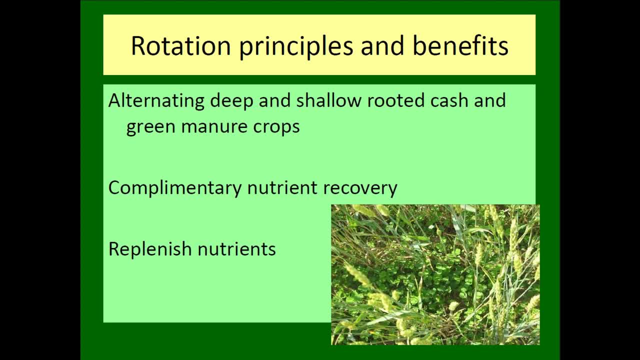 manure applications- this is true of all growers- and rely more heavily on the legume nitrogen fixation to ensure plenty of sufficient nitrogen. Okay, Another strategy in designing rotations is alternating deep and shallow rooted crops, And this applies to both cash crops and green crops. 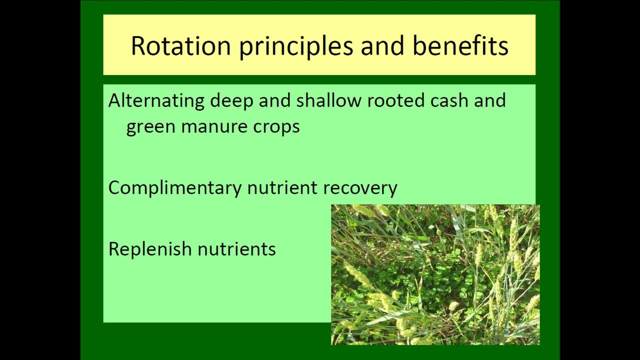 For instance, if you've been growing lettuce and spinach that have relatively shallow roots, if it's followed by tomato or squash, those production crops will actually send their roots three or four feet deep, And then you might want to follow that with a legume-grass combination cover crop in. 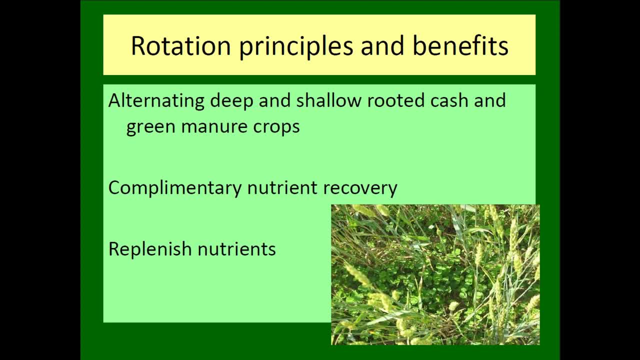 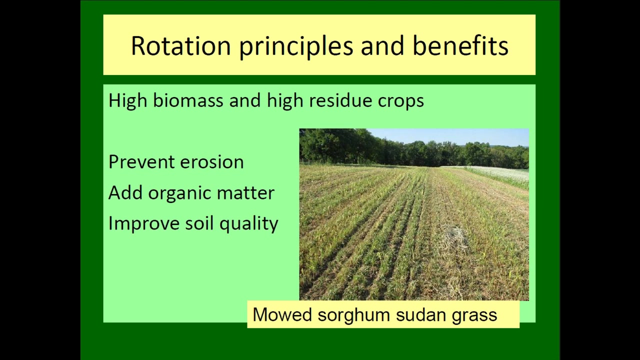 the fall, which is also fairly deep, And so you have a complementary use of nutrients, And it will also, If you're using legumes that are deep rooted, it will replenish nutrients to the soil profile. Next, Okay, It's always a challenge, especially in horticultural crop rotations, to ensure that sufficient 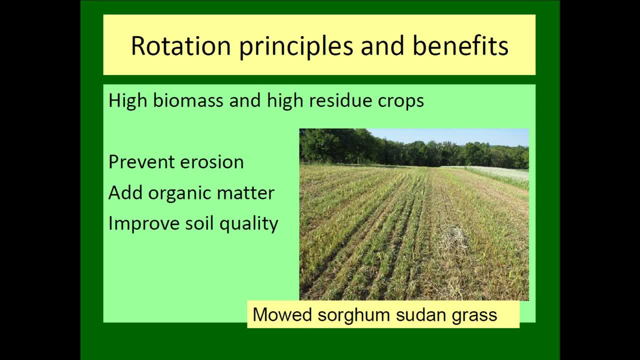 high biomass and high residue crops are included in the rotation. Of course, the cover crops help us out a lot there. However, remember also that there are several. There are a number of production crops that do as well. Cereal grains grow in four-grain production. 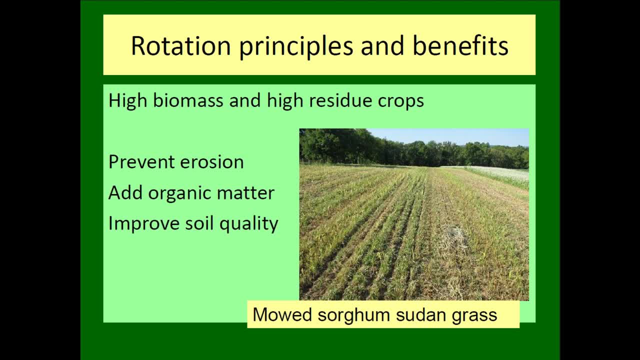 There is increasing interest in organic and specialty grain crops, And the residues, of course, are returned to the soil- Sorghum, sudan, which can serve as a forage as well as a cover crop- very, very high biomass Sweet corn. similarly. 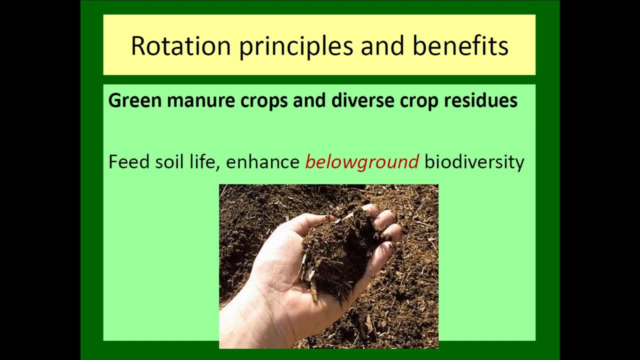 Okay, Next, Okay, Next Okay. One thing to keep in mind is that, again, the more diverse your cropping system, the more healthy and diverse the soil life, And you can look at it even just from the point of view of the physical architecture. 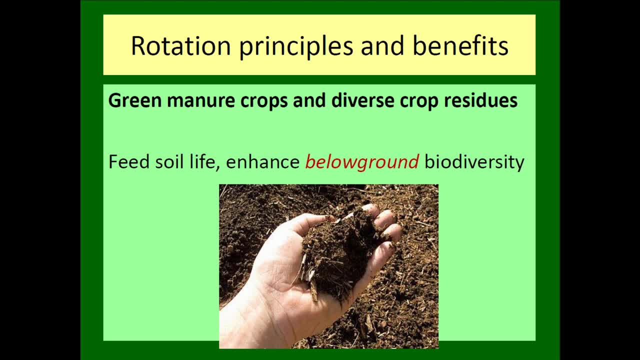 of the root system. Grass is a very fine fibrous net that just permeates entire topsoil. A legume like sweet clover or a brassica like radish will send a tap. A radish will send a tap, root down three, four, five feet. 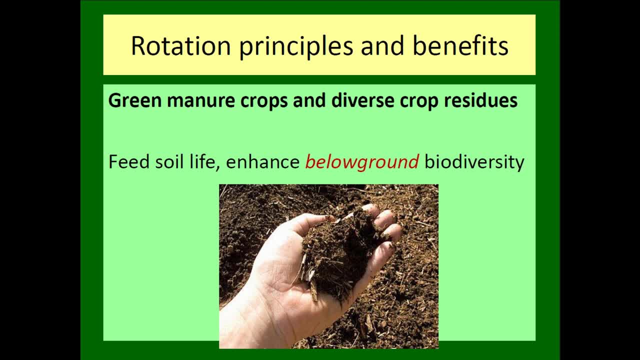 And various production crops will also have varying root architecture. In addition, every plant species gives off a distinct and characteristic spectrum of soil, of plant exudates. root exudates, Like just as a radish will taste different from a tomato, to us the exudates from a plant. 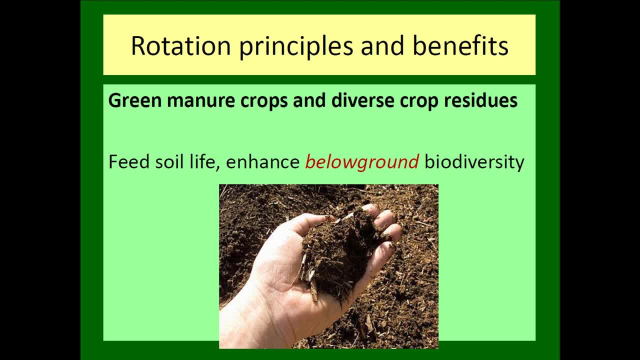 will taste different from a tomato. to us, Exudates from a brassica versus the exudates from a tomato family crop will look very different to the soil life. So different crops support different soil life And by varying this you will promote a greater diversity and balance in the soil life. 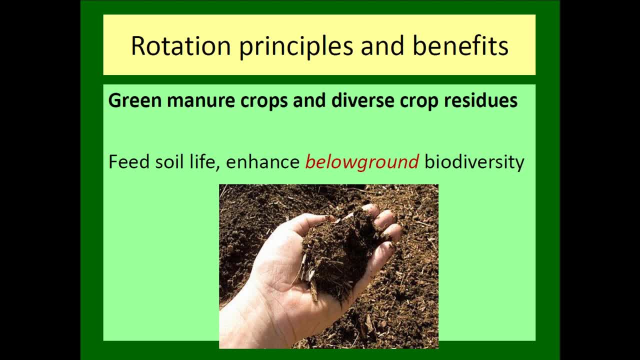 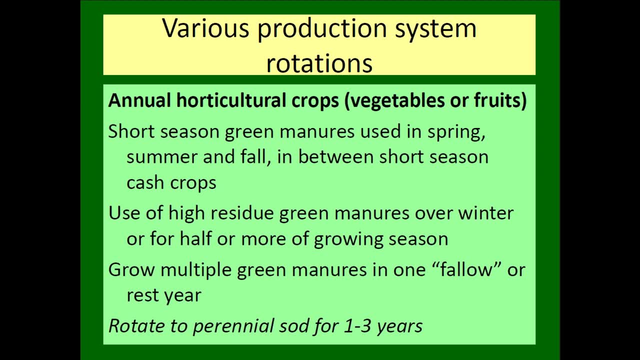 Next. Okay, So examples of rotation systems for horticultural crops. As I mentioned earlier, horticultural growers, especially in warm climates, will tend to try to grow two or three vegetable crops, like spring lettuce and late summer cucumbers. 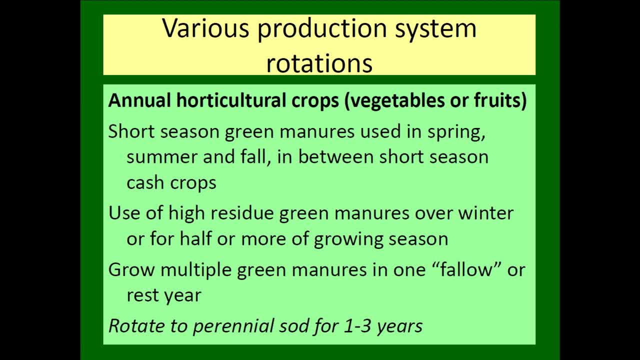 or a spring onion crop, followed by a fall broccoli. So the challenge is to incorporate into that rotation sufficient high residue and green manure crops to keep the soil life well fed And to Prevent erosion. Some examples are: you can grow a short-season green manure in the spring, like oats and 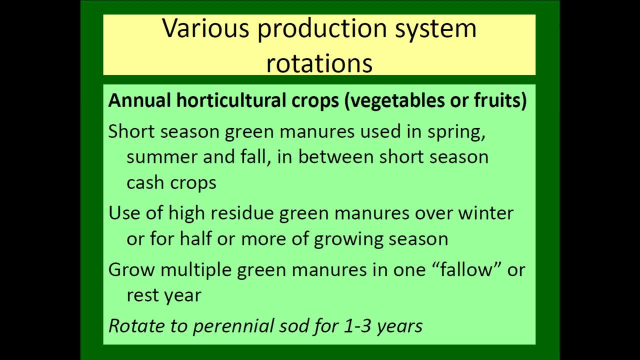 field peas And that can be incorporated in June in time for main crop tomatoes. It can even be in some cases rolled down After a spring vegetable, a mid-summer crop of soybeans and millet, or cowpeas or buckwheat. 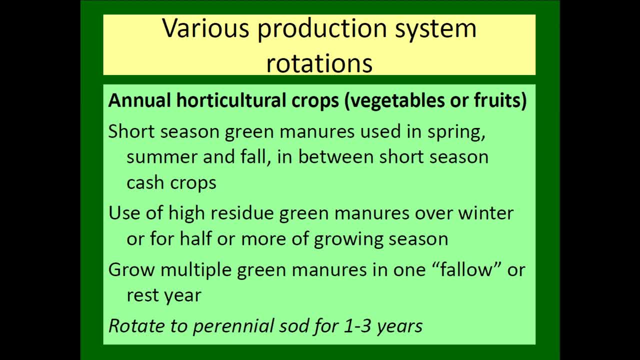 and that can often be followed by a fall planting, Such as garlic, which is planted pretty close to the frost date and is harvested the following summer. Many vegetable growers routinely use high residue green manures over winter, typically for rye or triticale or wheat, combined with one of the winter hardy legumes. 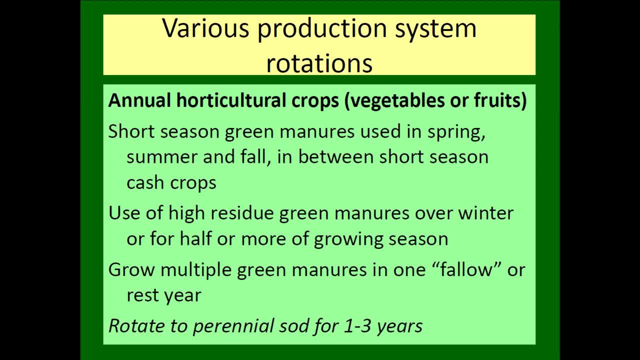 And also when the land resource, When the farmer has sufficient land to do this, it's really advisable- and it is often done- to rotate a field that has been worked hard for a few years into a full year of green manures. 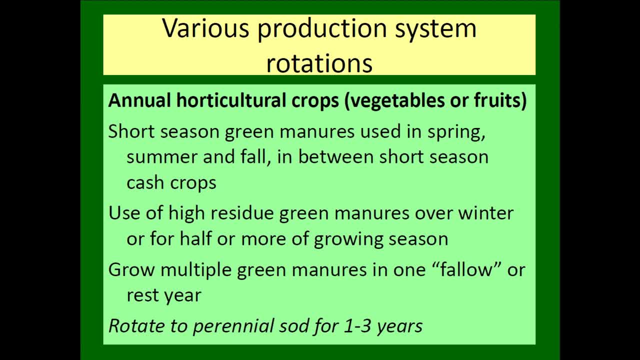 Either a series of annual green manures brought in quick succession after one another, or simply rotating to a perennial sod. You can sow a little bit of oats and then a mixture of perennial grasses and red and white clovers, such as perennial clovers. 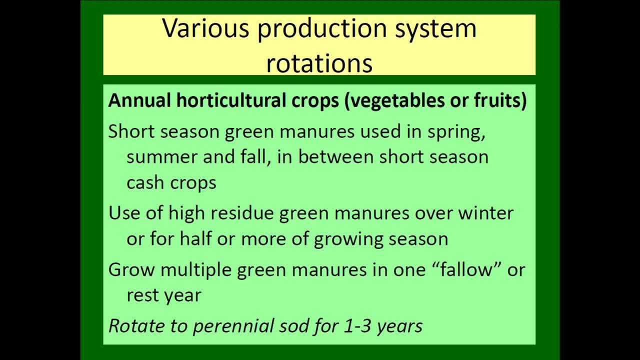 And then the oats can be mowed off or even harvested for grain, And the clovers and grasses can be allowed to grow one to three years. When that sod has been finally broken, the soil has had a chance to rest Very often. annual weed populations have reduced considerably. 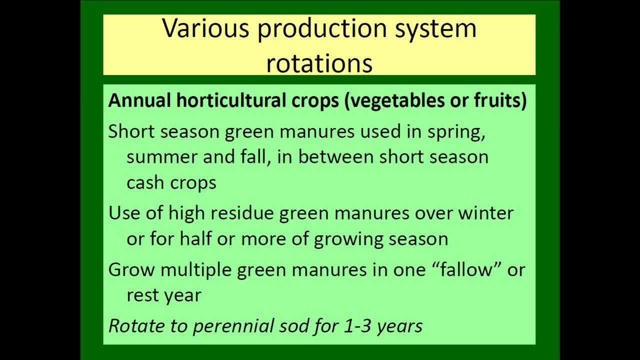 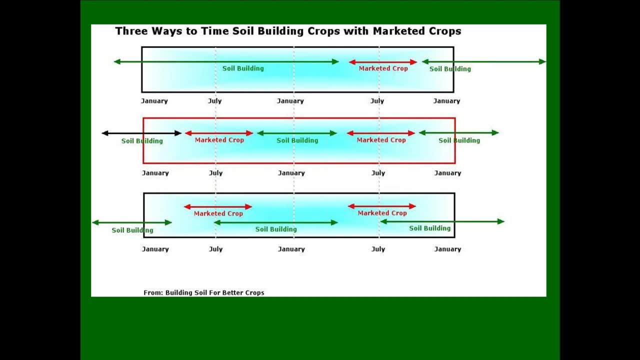 A lot of carbon and nitrogen has been returned to the soil And production often is. Many farmers have told me how good production is after that perennial sod year. Next, Here's just three timelines, three alternative timelines for soil building and production crops. 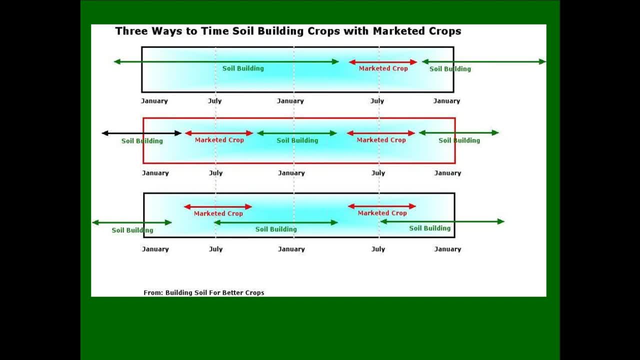 Some growers will actually have a rotation where they produce only in alternate years And then the intervening year again is either the perennial or a series of annual soil building cover crops. Farmers with a smaller land base may choose to do a marginal crop. 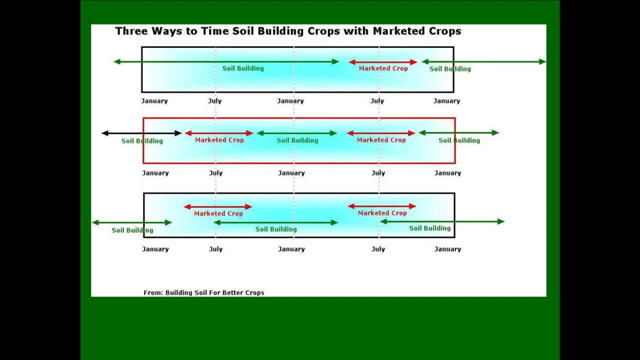 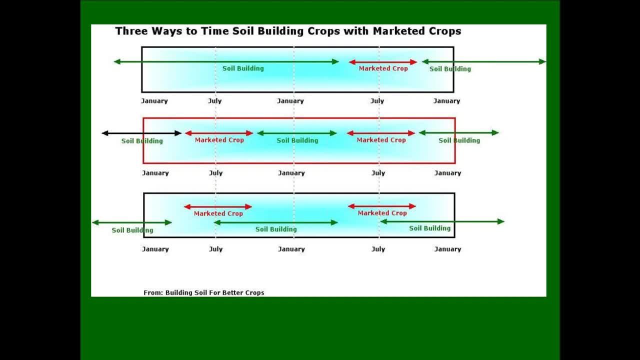 I would have to comment that on this diagram, if the rotation is on that schedule year after year, where the production crop is planted in the late spring, unless they are able to do no-till cover crop management, that can lead to a buildup of annual weeds. 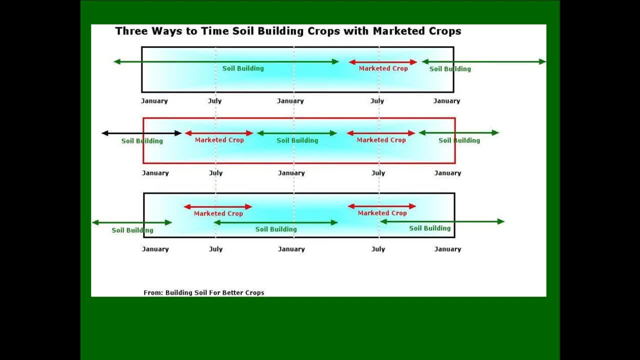 after several years, because the soil would be disturbed at the same time each year. Another strategy is to actually plant the soil building crop into the perennial soil building crop. when the production crop is established but is not yet mature, Then the soil building crop- typically a shade-tolerant species like clover- will get established. 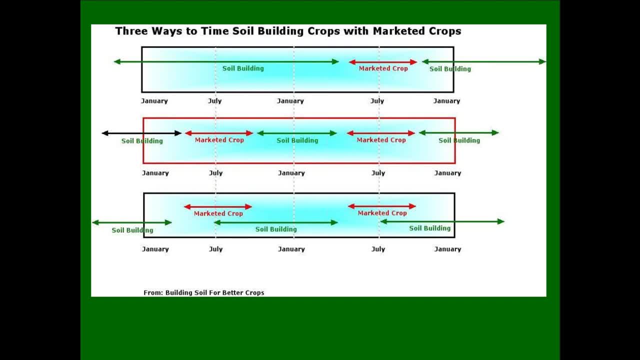 And as soon as the marketed crop is harvested off or cleared or is killed by frost at the end of the season, the cover crop then takes over. Many growers will seek to vary, make the rotation a little more flexible. They will be a little more diverse by varying the planting date of that marketed crop. 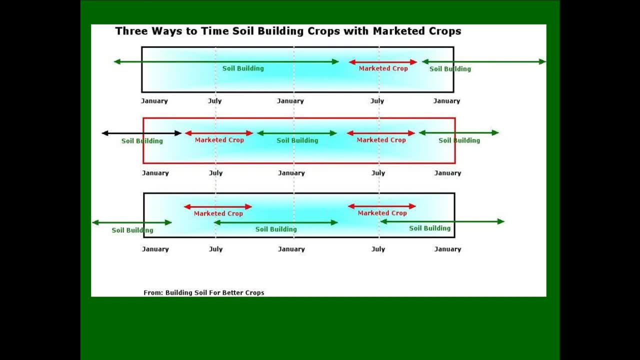 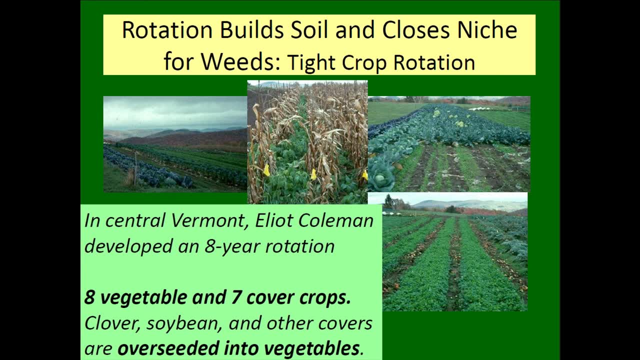 Next, Here's an example from central Vermont. That is a very cold climate about Zone 4.. This is Elliot Coleman's farm. I took these photos about 30 years ago when he was farming in central Vermont at about 1600 feet elevation. 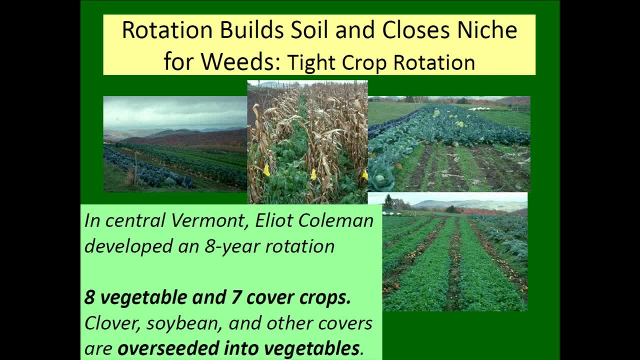 That's eight vegetable crops and seven green manures in an eight-acre farm And very little bare soil Again. that's that corn-soybean intercrop. He also has brassicas which are just in the middle of harvest. These photos were all taken in October after the first light frost. 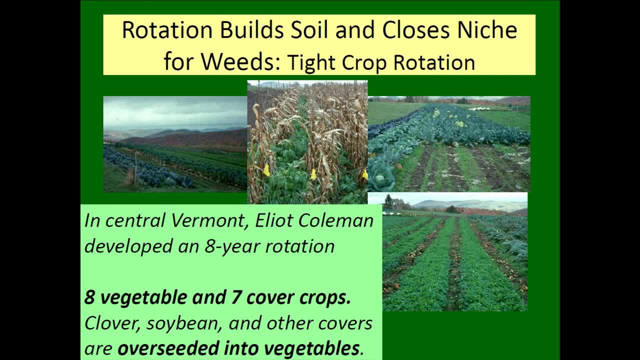 You can see as he's clearing the brassicas, the clover is already established, And below that, where the tomato harvest ended a little earlier and the plants were cleared, the red clover in the alleys is almost completely clear, And then the green manures. 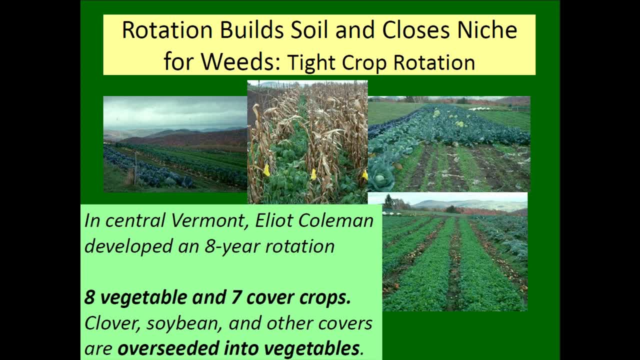 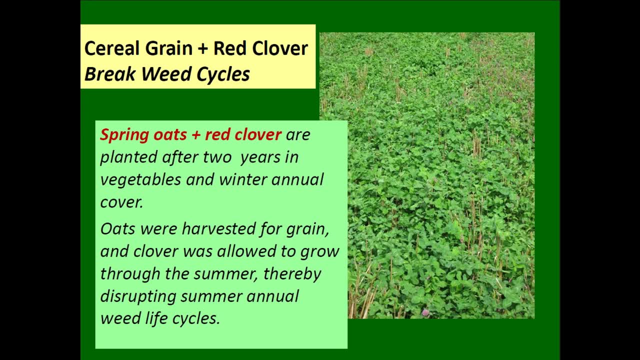 They're completely covered to ground. Next, Here's an example from here in Floyd, Virginia, where I live, This field was in intensive vegetable production for a couple of years: one or two vegetable crops and one winter annual crop each year. In the third year it was planted to a cereal grain, under-seeded with red clover. 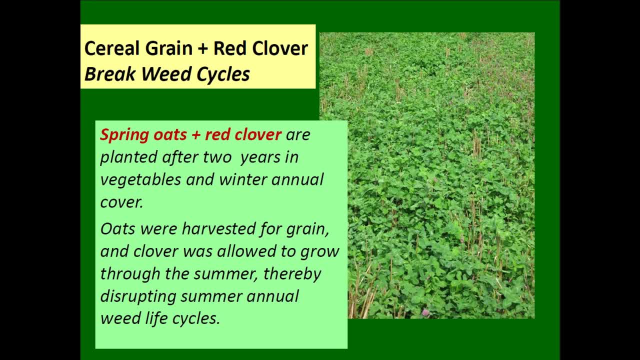 The cereal grain was harvested off and harvested as grain, and the red kohlrabi was allowed to grow for a full year. This is an example where you can get two years of intensive production and then one year in rest, Depending upon the soil quality and the needs of the soil and also the market needs of the. 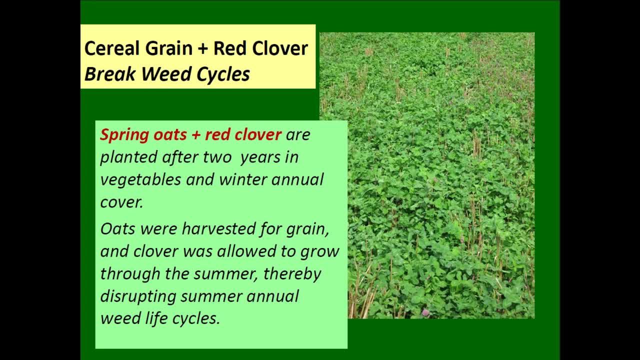 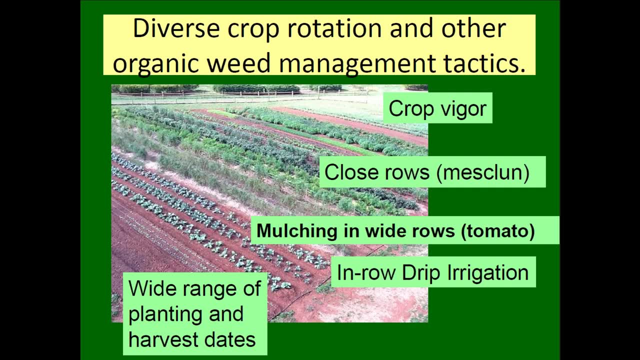 farm, that perennial period could be extended to two or three years. This is an example of how a vegetable farmer can implement a diversified crop rotation, not only in terms of plant family and crop architecture, but also in time. This is an aerial photo of a garden at Guilford College, a small farm. 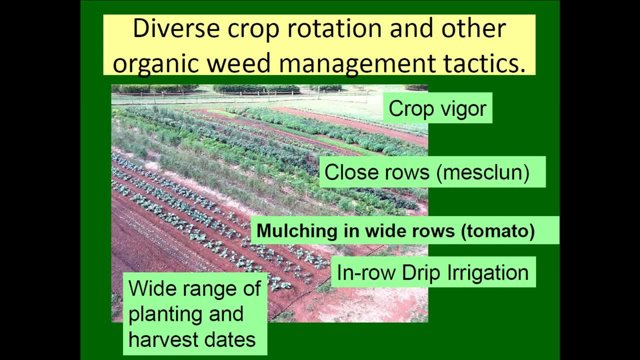 You can see that some crops are near harvest. They have completely closed canopies. some crops are at mid-growth, some have just been planted, Although we do see some bare soil there. you also see illustrated here the opportunity to vary the timing and the type of soil disturbance that each particular bed receives. 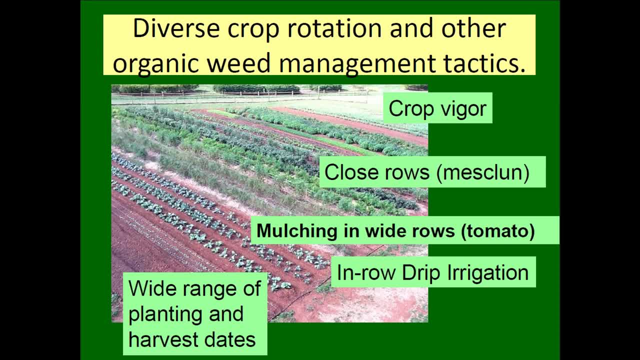 Because next year the position of all those crops will be moved, so that the ones that have been tilled and planted in mid-summer, just before this was taken, will be moved and would be planted early in the spring and would be under a heavy crop canopy mid-summer. 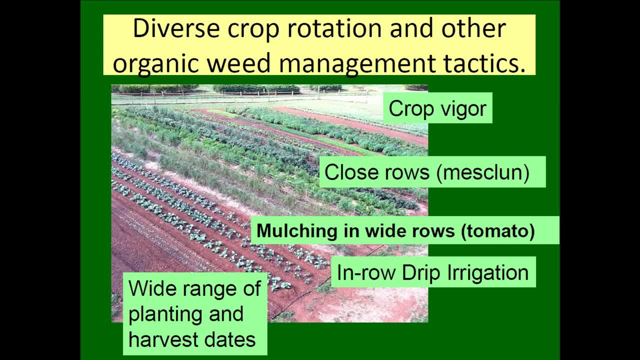 This can aid with weed management, and this is very important because weed management is the Achilles' heel of the organic producer and that often repeated cultivation is required. You see a number of alternate tactics here to reduce the need of cultivation. That in-row drip irrigation on all those beds means that they're going to have a lot of. 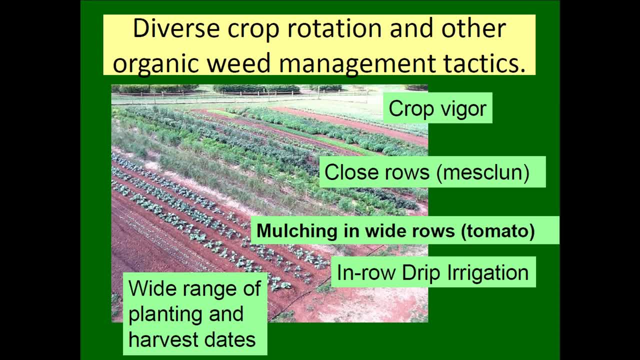 weeds. This means that the farmer is feeding and watering the crop and not the weeds. There are organic liquid fertilizers that can be provided, such as fish emulsion, right through the drip, The mulching and those wide-row crops. of course, that's keeping weeds down without. 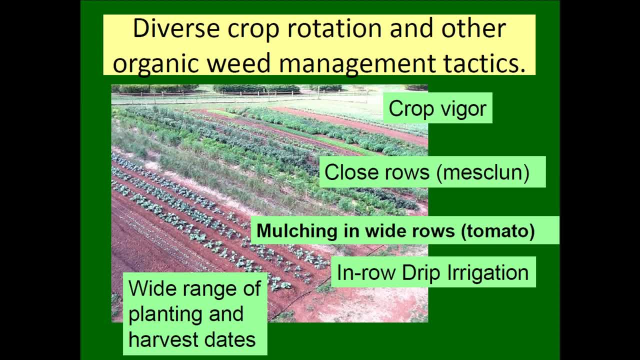 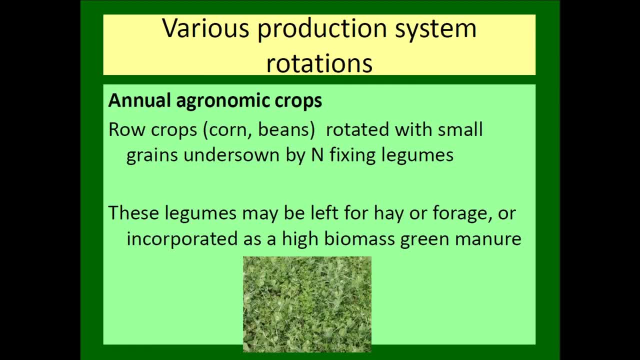 cultivation. The crops that have closed the canopy are providing their own weed control. Next slide: Okay, I'm going to talk a little bit about the more corn and beans. Even though these, These are crops that will go all season, those farmers also have a way of getting those. 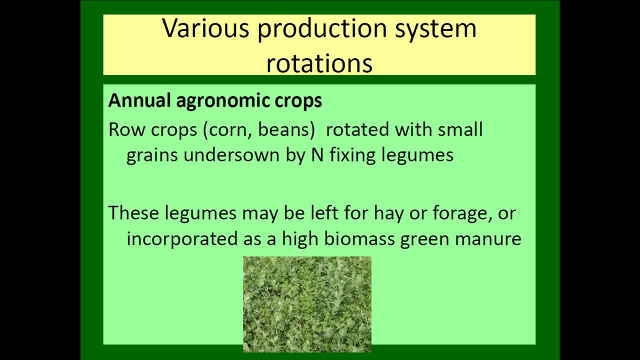 cover crops in. For instance, in Iowa I've seen quite a few producers come in very early in the spring, if it's dry enough, and they'll put in a crop of oats and then they'll have enough time to till that in before they plant their soybeans. 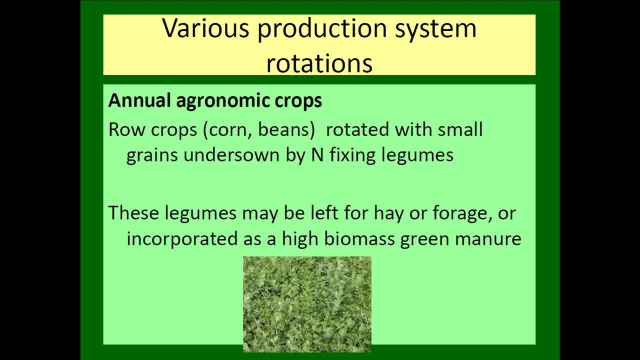 The same thing. They might come in after soybeans and put in rye And rye and vetch. So they'll try And even once in a while you'll see even some inter-seeding, let's say into corn at. 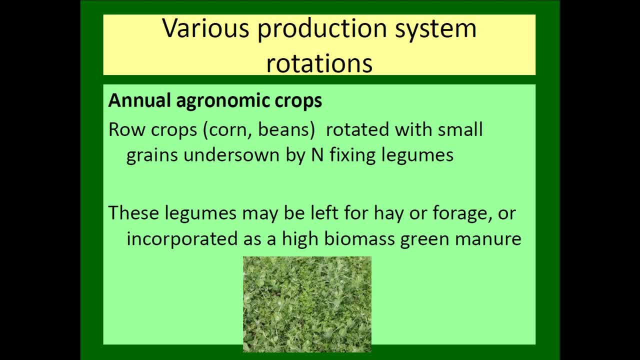 the last cultivation. They might have a broadcast feeder on the front of the tractor and at the same time they're cultivating and just kind of get that seed in Something fairly inexpensive like a red clover, or even throw in grasses and buckwheat, just. 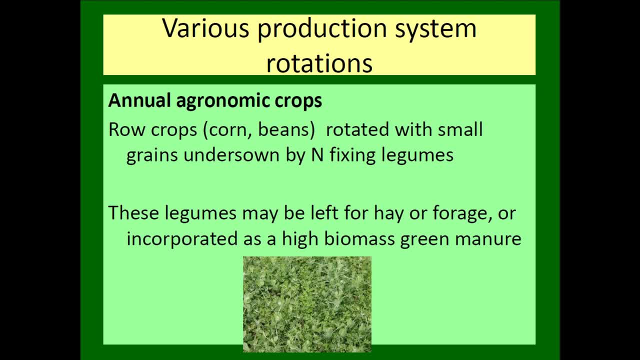 to get some cover on there. So there'll be something to till in before they get that seed, in something to fill in just some more biomass And of course in a row crop rotation they are going to be basically forced by the certifier. 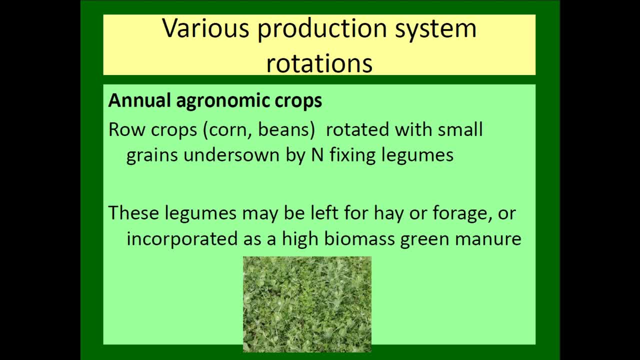 even if they don't want to do it, to put in some kind of small grain and legumes in rotation, And they may choose, even if they don't have livestock, that they'll put in a clover and then just fill it in. 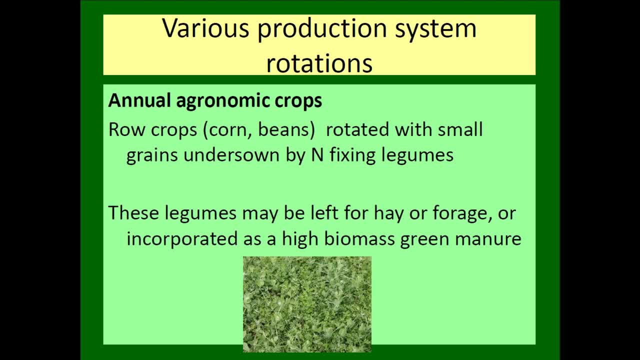 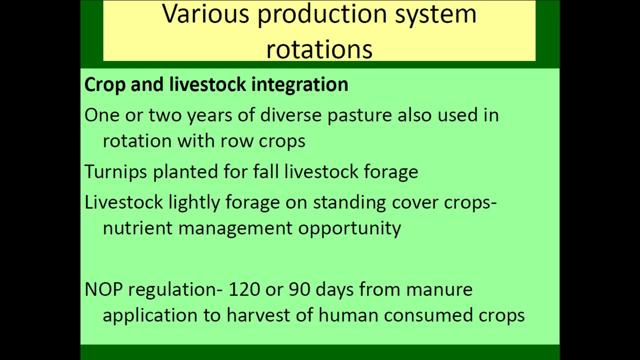 They might not even harvest it for hay, or they might have hay as part of their rotation Next slide. The other thing, too, is that if anybody has ruminants on their farm that are certified organic, they are going to have to get a significant portion of their feed value from grazing. 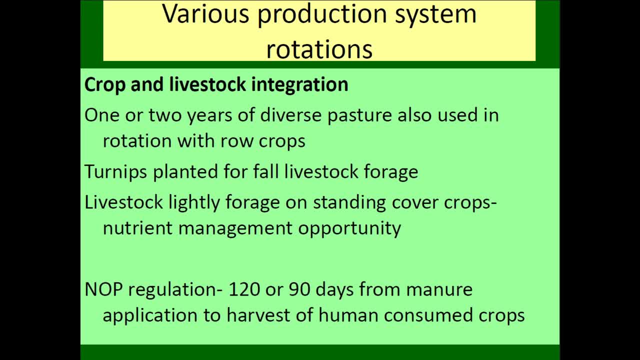 And so high-value pasture. pasture is very much a part of the crop rotation. The pasture on an organic ruminant farm- either beef or goats or dairy- is not shunted over to the kind of rocky side hills. It is very much right in there with the valuable fertile flat bottom land. 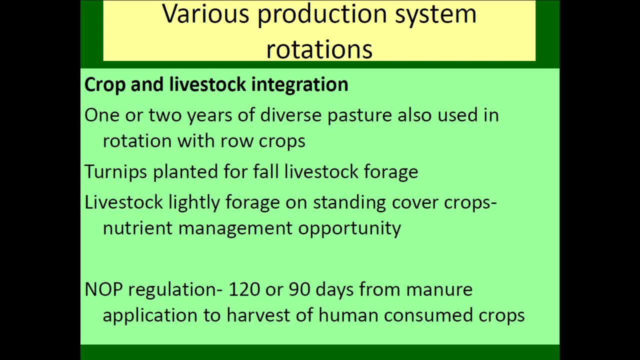 because they need that pasture as a significant portion of the feed that they're giving to the animals And so they include many times pasture And they're in the rotation. So you might see, you know, corn beans seeded to oats. 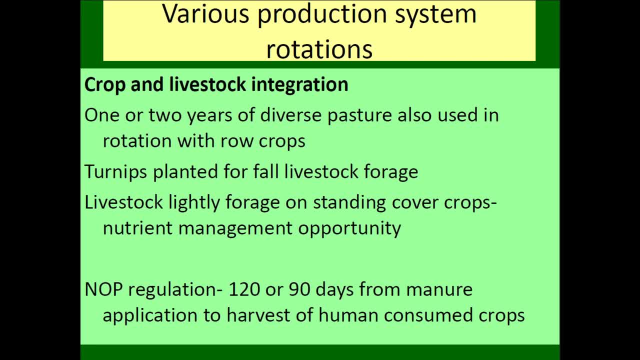 and then underseeded with a pasture mix, and then it sits in pasture for three years and then they go back to corn. You might see also that perhaps after a small grain is taken off, if it hasn't been underseeded, or even if it had been, they might till that in. 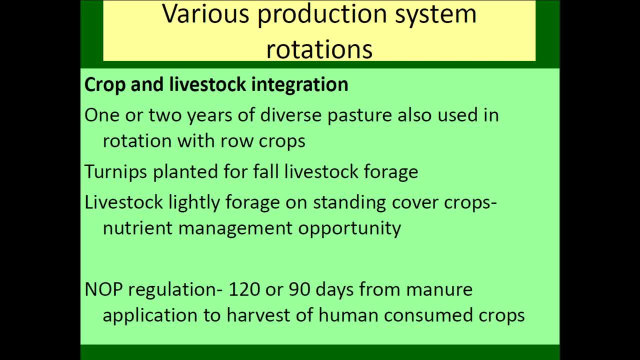 and plant turnips for fall livestock forage. You might see, you know a lot of the livestock perhaps out there foraging, you know, on the hay crop at last. Instead of taking a last cutting or taking a mid-season cutting, they'll rotate that as pasture. 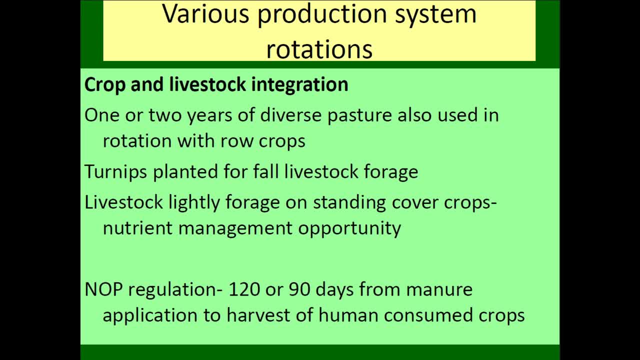 getting then the animal manure on those fields, on that living vegetation, and then rotating it back to a hay crop for the last crop or whatever. And again, as Mark said, if you are doing vegetables- and this is only for human-consumed crops- that there has to be a waiting period. 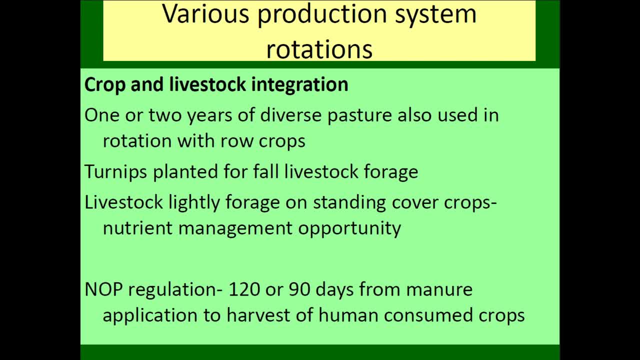 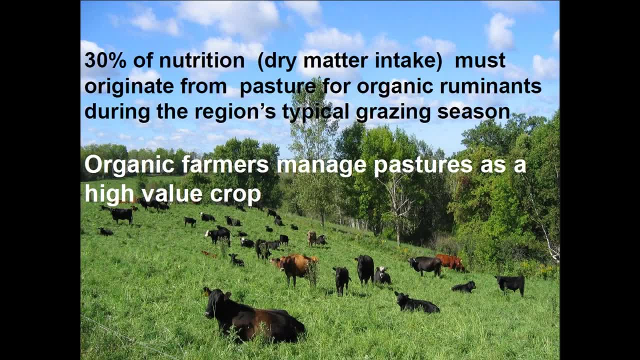 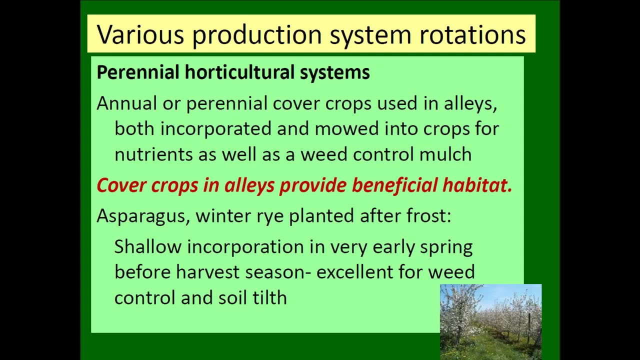 between the application of raw manures and the harvest of the crop. Next slide, Next slide. Somehow this slide doesn't like me. Hello, There it is. There we go. So the whoops No Too far Back to the grazing. 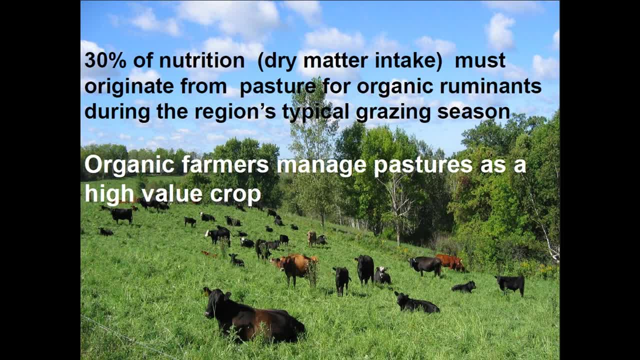 There we go. So, as I said that pastures are a high-value crop, because 30% of the nutrition during the grazing season has to come from pasture. A lot of times, too, you will see organic farmers. they underseed their small grains. 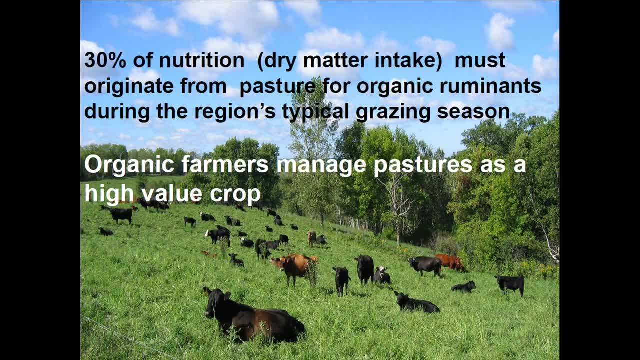 with some type of legume, whether or not they're going to harvest it as hay, because it underseeds It also again, typically will fix nitrogen. It will give them a wonderful green manure to incorporate And it also serves as a weed control because they don't have bare ground. 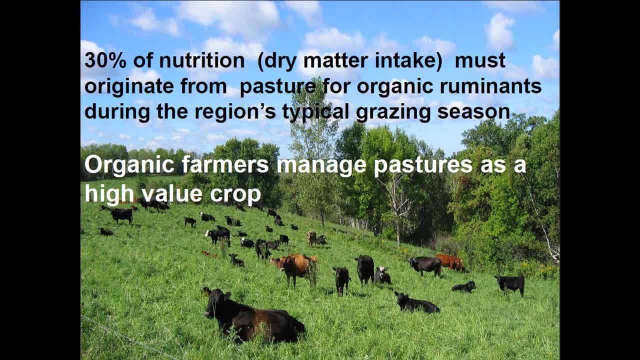 onto those small grains. they have it seeded down with clover or alfalfa. You'll also find organic farmers interseeding grasses into their alfalfa because they have that better carbon to nitrogen ratio when they till it in And also it is less than a year. 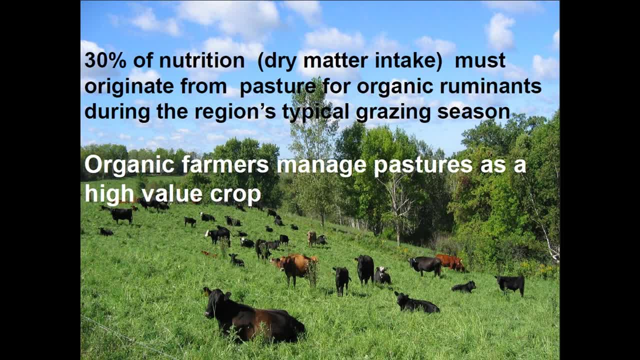 It is less attractive to leafhoppers if there's some grass in with the alfalfa rather than just having a monoculture. And lastly, it's better for ruminant health to have a mix of forage Instead of having 100% alfalfa hay. you've got those long-stem grasses. 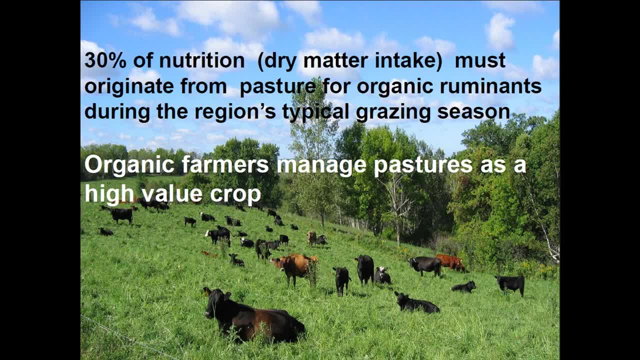 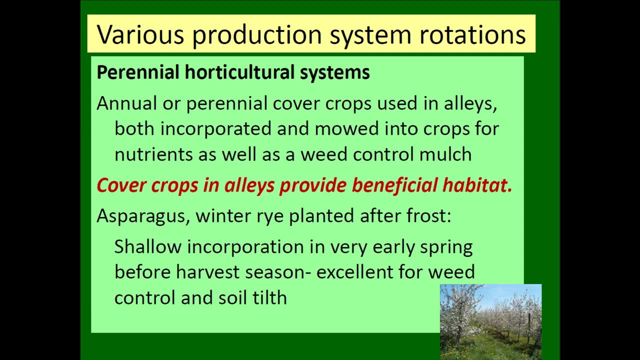 which are much healthier for those ruminants. Next slide. So in perennial horticultural systems there are many things that people can do. They can either plant annual or perennial crops in the alleyways that are mowed And then actually the mower can then blow that cut crop into the area under the trees. 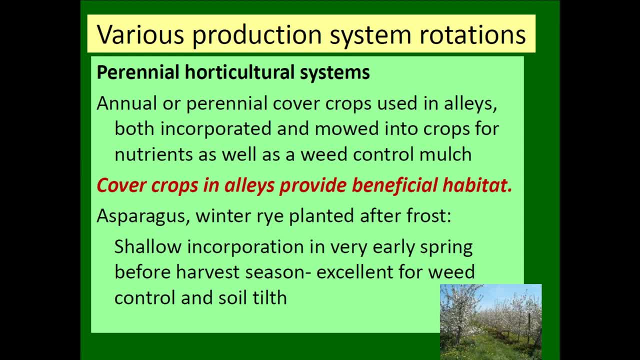 And then they have a mulch. They can grow beneficial insect habitat during the season with something like buckwheat or other perennial crops, And here in Wisconsin I see a lot of asparagus growers And these can be people. I've seen people doing it at even the 50 to 100-acre asparagus farm. 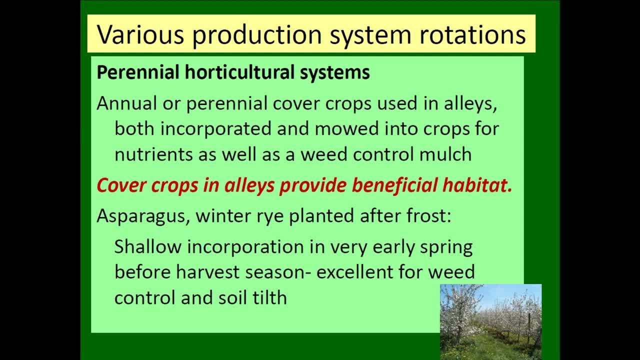 where they plant winter rye after the frost And then in the early, early spring they will shallowly incorporate that And that does a great job, for then you know, keeping that perennial crop, improving that soil tilt, And it offers weed control. 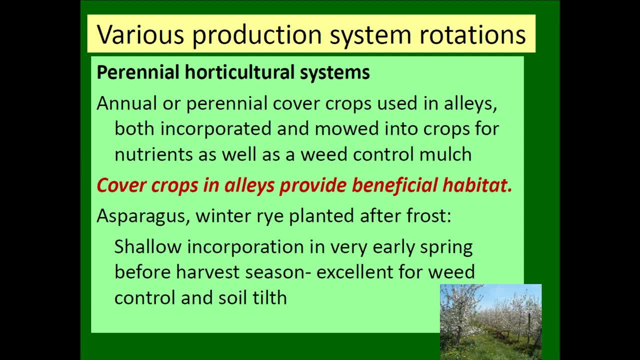 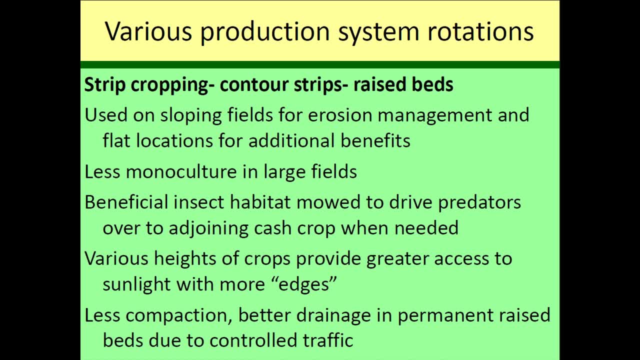 So that's one of the things that we do, And that's one of the things that we do Next slide. So even in the agronomic system, you can have strip cropping, as the NRCS has a practice standard on that. 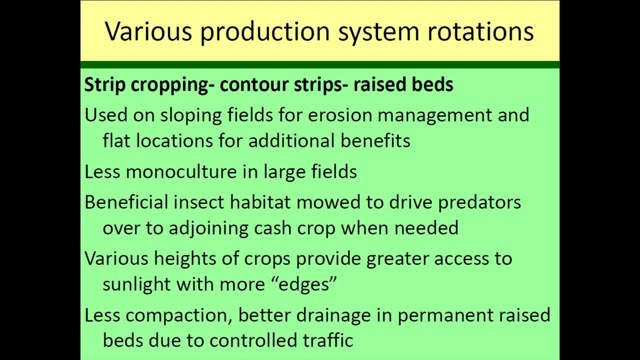 And by breaking those monocultures you're breaking those diseases, breaking those insect cycles. You'll see a lot of organic farmers wanting to put in field borders and conservation. You'll also see them growing thin strips of beneficial insect habitat annuals, let's say. 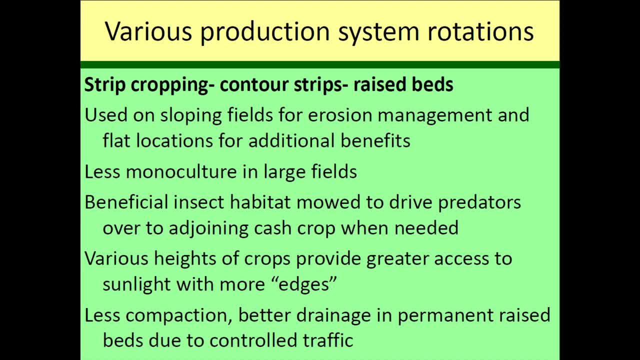 down the middle of their field and then mowing them off when they start noticing insect pressure in their cash crop, driving those beneficials over into their cash crops when they're needed. So you basically kind of raise them and then kick them out of the house and say go to work. 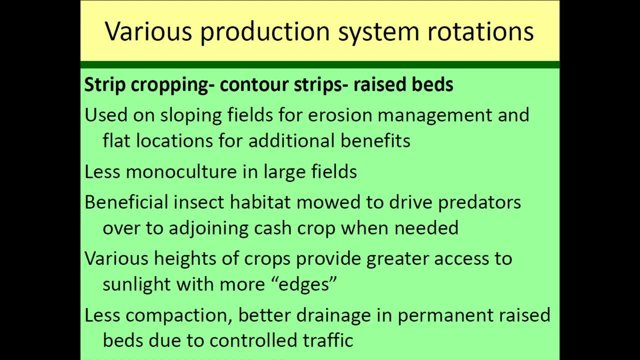 Another thing too is strip cropping. By having various types of crops, like having soybean strips next to a corn strip next to an alfalfa strip, you get more light along those edges and increase your yield. And those organic farmers who are doing vegetable crops and they have permanent raised beds. 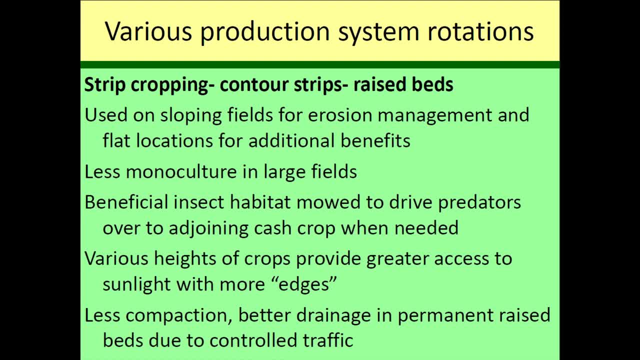 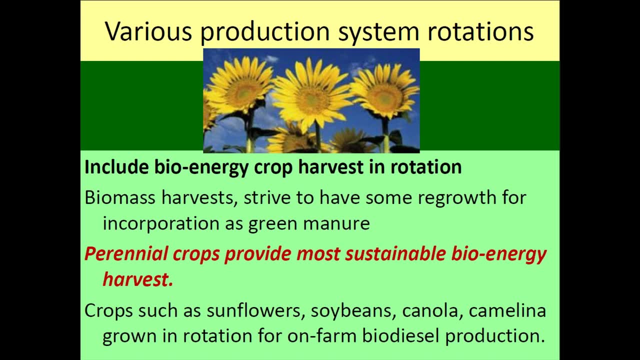 they have much less compaction in those beds because the wheels of the tractors are never driving over where they might grow. So that's a little crop in the future. Next slide. Another thing you'll see is bioenergy crops. A lot of organic farmers and conventional farmers are interested in saving money. 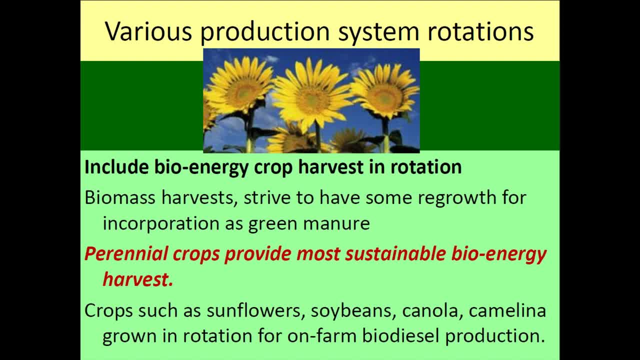 And they are, you know, very attracted to the fact that maybe they could change their diesel tractors over to something that can run on biodiesel and they can actually, you know, produce their own fuel. So you'll see sunflowers, soybeans, canola, camelina grown in rotation on many farms. 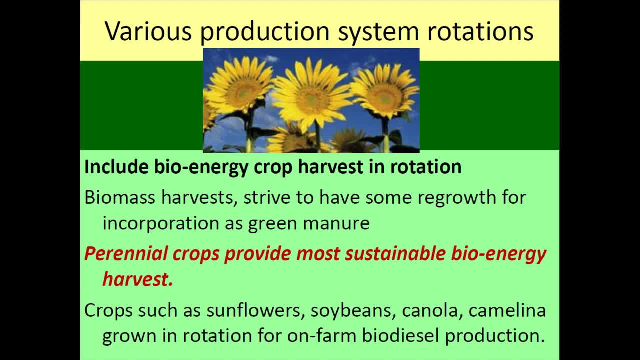 for that biodiesel production. Another thing you see a lot on organic farms for vegetables I have seen is taking those smaller tractors- things like Alice G's and those older Farmalls- the A's and the C's- and actually making them electric tractors. 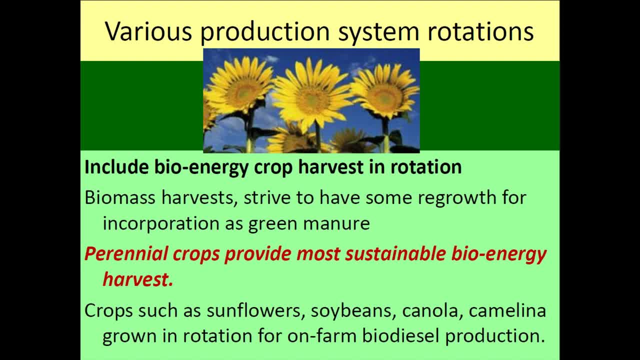 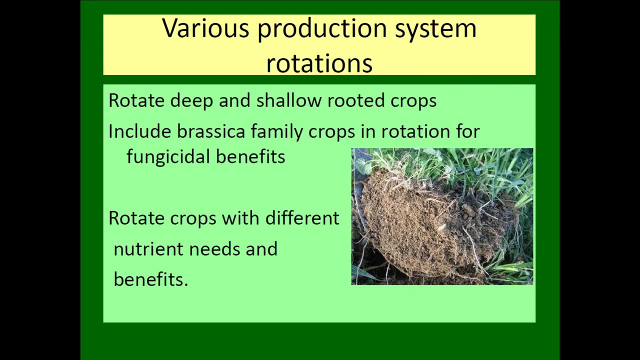 And then I've been talking about that. You can go into farms that have windpower or solar And then they plug in those tractors And all that fuel for running their tractors is all coming from renewable resources. Next slide, So just to kind of wrap up. 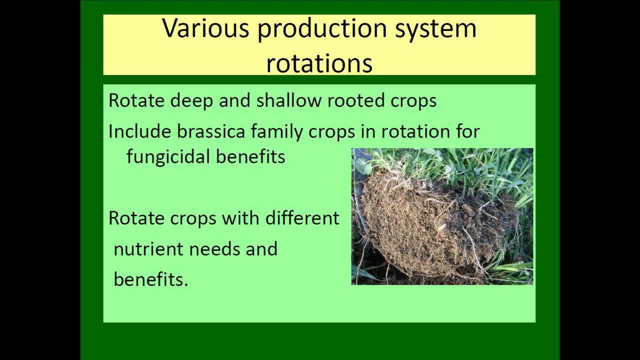 People are, you know, are looking to it. This is something that organic farmers really think about, both agronomically- crops like corn and beans and small grains, As well as, As you know, the horticultural crops to really rotate those deep and shallow rooted crops to 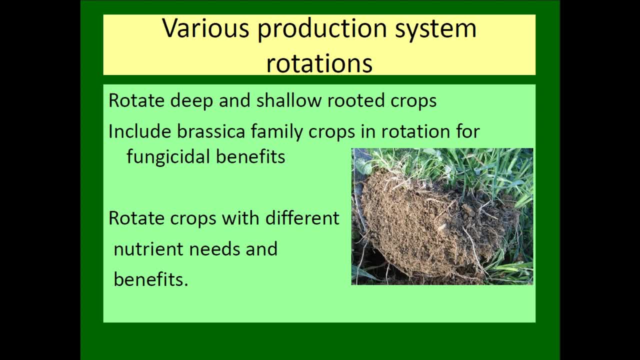 think about rotating crops to offer benefits to the succeeding crops. so the Brassica family has some fungicidal benefits. so if they're following with another crop that they've had some issues with a fungal problems, especially root problems, they might say, well, I really need to. you know, put Brassicas in. 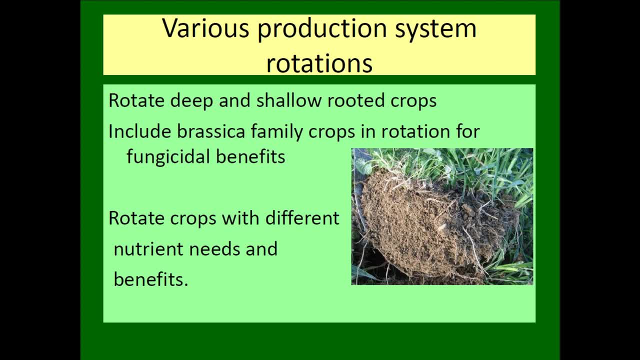 before those crops and, of course, always looking to rotate the crops with different nutrient needs and benefits, and this is something that's been done for generations. you know there's always been at the alfalfa, at least here in the upper Midwest, with dairy farms. you know they always follow the corn crop after. 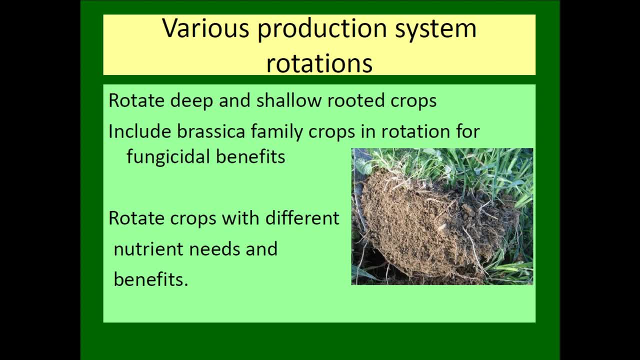 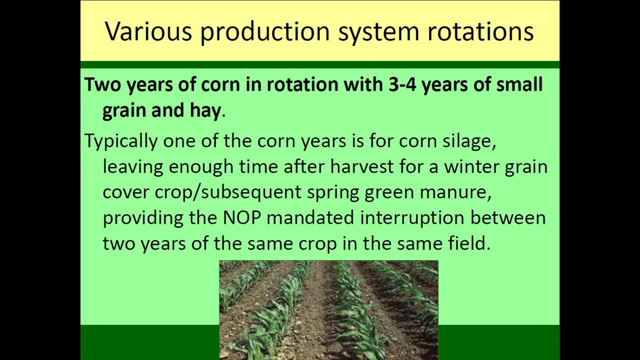 they plowed in their alfalfa. next crop, next slide. I'm already a pick about crops, so you're going to see a lot that in a five-year rotation crop. you're going to see a lot that in a five-year rotation crop. you're going to 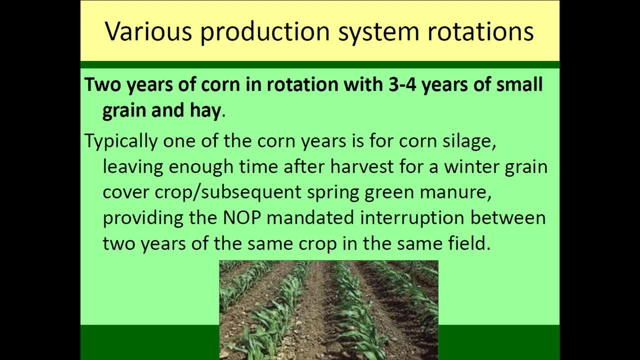 also see a lot of long rotations on organic farms, anywhere from three to four years to seven and eight years, where they're growing a whole variety of crops to break those monocultures, to break those weeds and pest cycles. you might actually see at times on an organic farm, especially a dairy, where 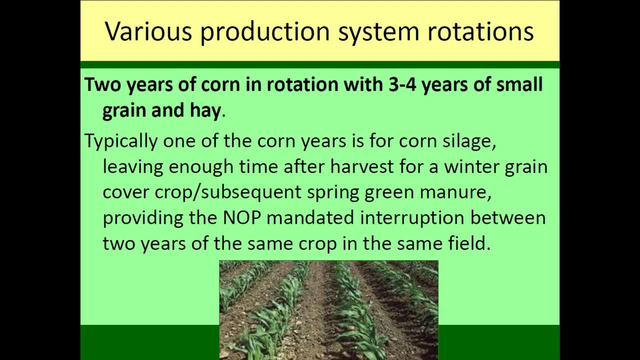 they might grow two years of corn in succession, which technically doesn't meet the organic regulation, but then they are putting in a small grain and leaving it in hay for another four to five years, and so when you're looking at that seven to eight year rotation, there's only two years of road crop. it's 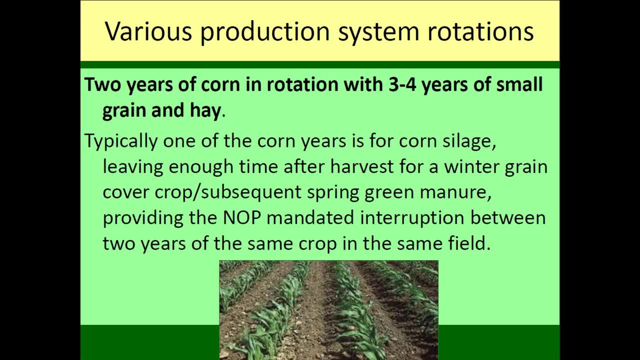 much more of a soil building rotation, and so this organic certification agencies have found that to be acceptable. another thing that I see people doing is perhaps putting in a rye crop. there's, let's say that first corn crop was a corn silage. they would have enough time to come in and Thursday and 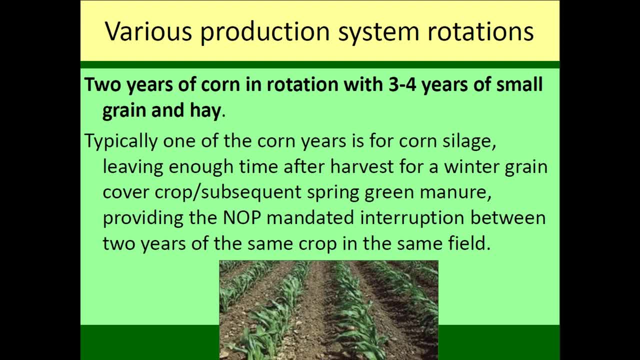 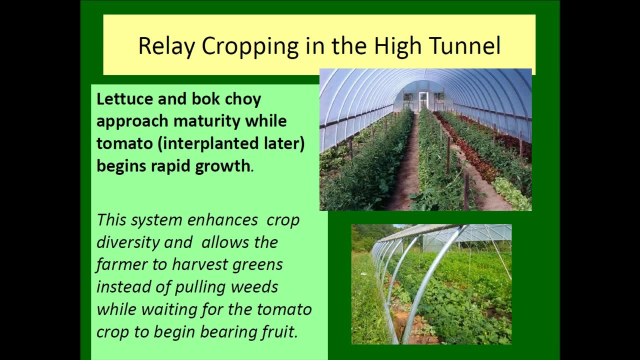 that residue, plant rye for the winter and then the next spring fill that in and plant corn again, And then they've had that mandated interruption between two years of the same crop in the same field. Next, slide In high tunnels, you'll. 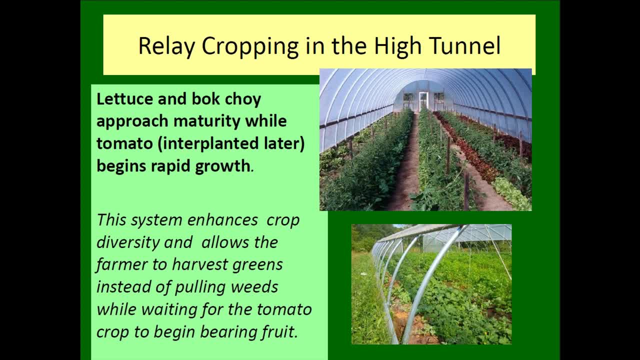 see that again, that they shouldn't be growing tomatoes and tomatoes and tomatoes. They're rotating various high-value crops. They might even try to grow some lettuce, let's say, next to the young tomatoes, and by the time the tomatoes are shading out that lettuce and going into production. 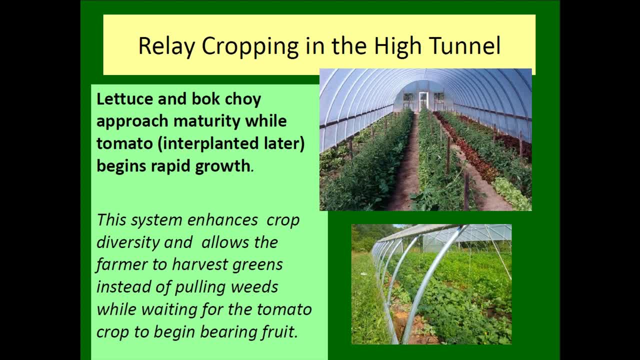 the lettuce has already been harvested. So in that high-value real estate under that high tunnel, they are really paying attention. And then the picture on the bottom is actually my high tunnel And you can see I've got some melons and there's some young tomatoes that you 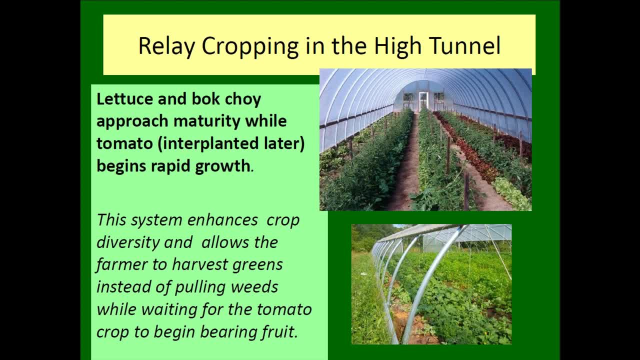 can't quite see there, And then I've got most of it in in a in buckwheat, because I grow- mostly in that high tunnel through the winter- spinach and lettuce here in Wisconsin And last year I sold greens every week from October to May. 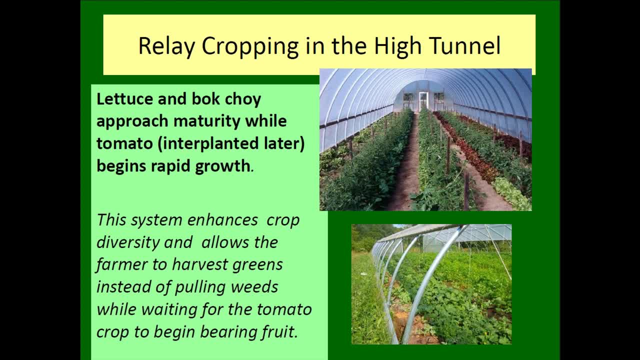 And so for me, I wanted to make sure that that that soil in there was was fertile and that I was dealing with the soil that was in there. And then I've got some with my weed problems And actually I tilled in that buckwheat and right now I 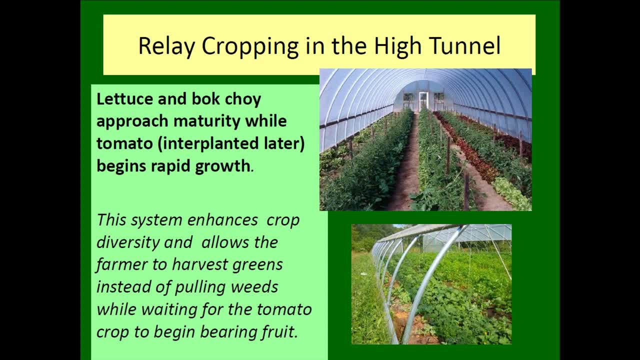 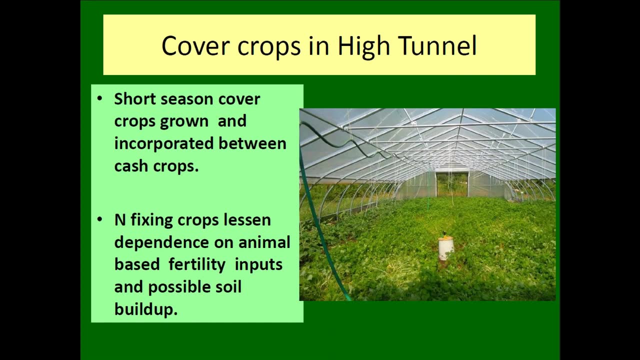 have a mix of tickling vetch and oats growing in there And I will be tilling that in in a couple of weeks and then planting my spinach and lettuce for my winter season Next slide. So for for both agricultural producers and agronomic producers it typically can. 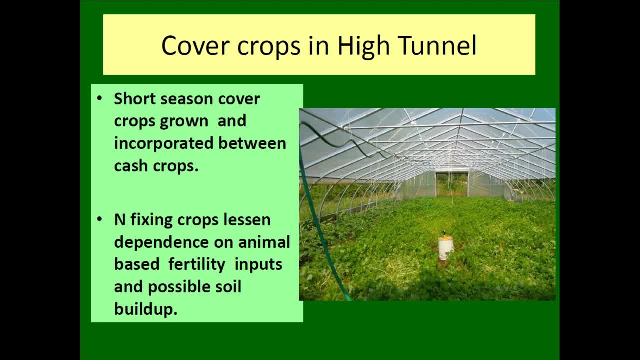 be a window in the beginning of the season, at the end of the season, or if someone's growing a small grain, even mid-season, to put in a short season cover crop. You'll also find that organic producers are using things like planting oats in the fall and letting it winter kill, And that can be done, you know, on a 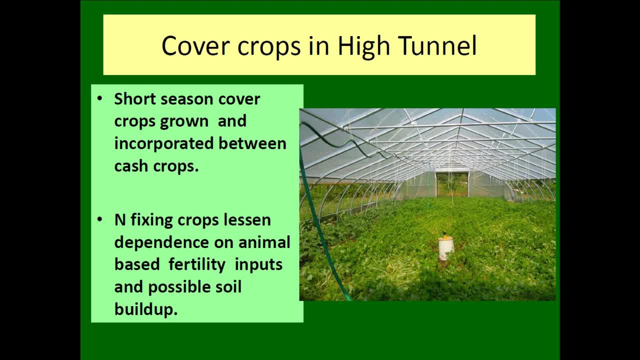 farm that's growing corn just to kind of protect that soil over the winter. But then they don't have a living crop they have to incorporate if they want to put in an early season crop, let's say, like corn or spinach. They just basically have. 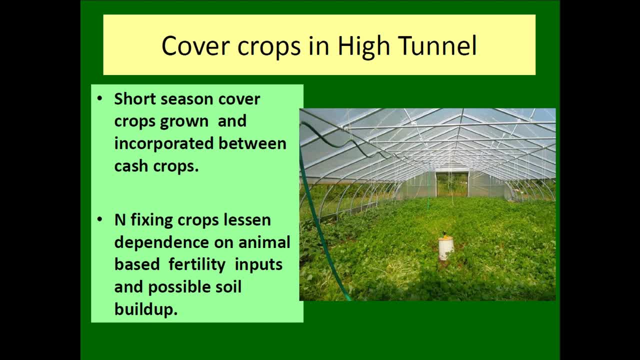 a kind of a mulch that died in place And of course the oats, even planted this time of year, would not go to seed. You're just going to get that green vegetation. Another thing that I see agronomic producers do is they plant rye in with. 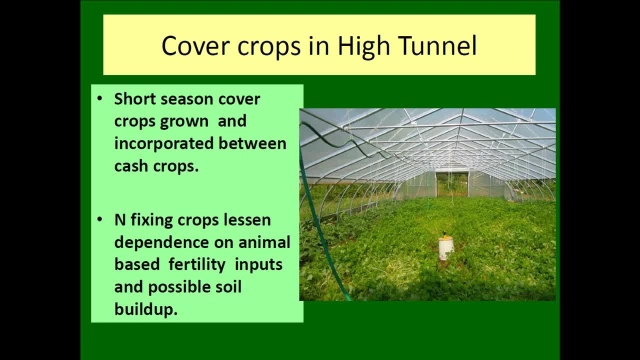 their drilled soybeans in the spring, And the rye is a very good source of fertilizer, So rye actually then crowds out any other weeds that grow, And those would be mostly for producers who are growing livestock feed grade soybeans, because there will be some staining of the beans when they're combining them. 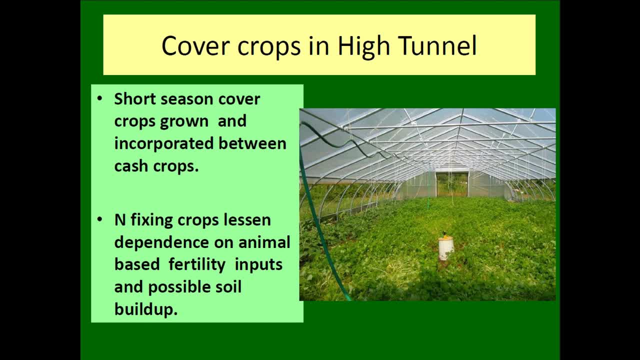 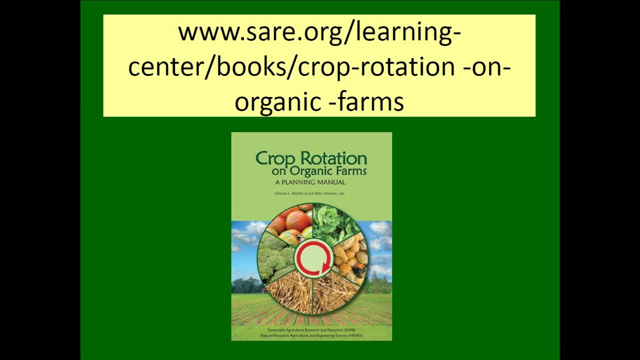 But it does work quite well. And of course, then you don't have a monoculture either. Okay, next slide. This is an excellent book put out by the Sustainable Agriculture Research and Education Fair. This is the website and you could go there and, you know, download it PDF by as. 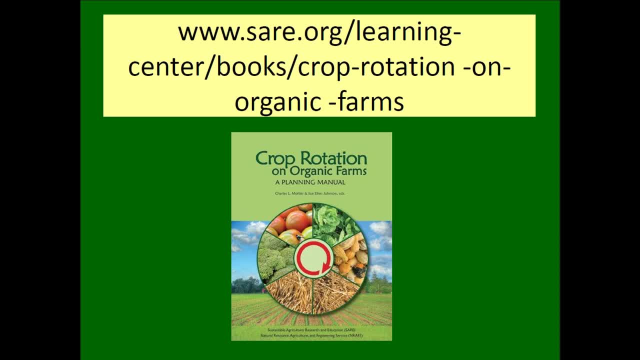 a PDF, chapter by chapter, Or you can purchase the whole book, and it's an excellent book which has a lot of different rotations for different types of farming systems, A lot of ideas for various cover crops and how to fit them into the rotations, And so I would recommend that to anyone who wants to. 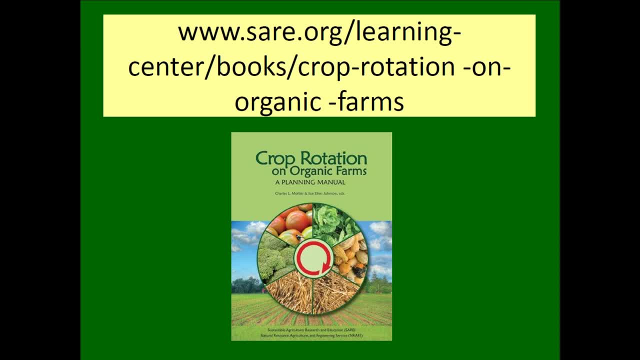 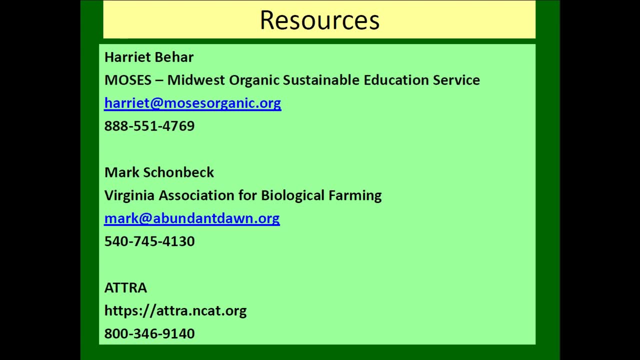 learn more Next slide. And here's my contact information: Mark and Atrus. Thank you, Harriet and Mark. Thank you very much. It's a lot of information and we've had a lot of questions. I'm sure we won't be able to get to all of them. the 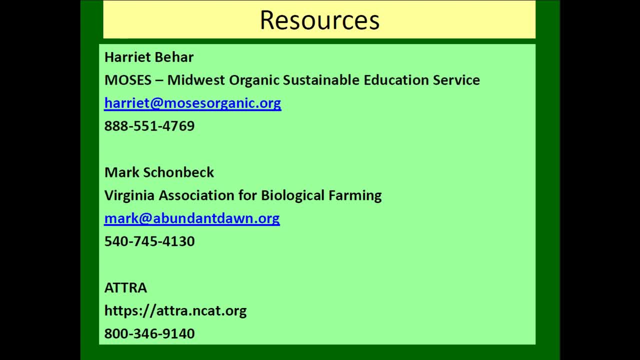 remaining time we have, But I'll start down the list and see how far we get. A collar has a small avocado orchard and has some extra room around on the outside of the orchard And it's a very good source of fertilizer And it's a very good. 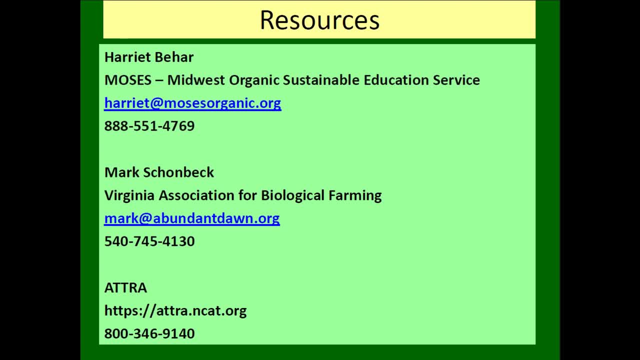 source of fertilizer And it's a very good source of fertilizer And it's a very, very good source of fertilizer. And they're wondering whether cover crops- I guess they're kind of hinting at orchards- and cover cropping And I guess it's not exactly a rotation- But are they useful? 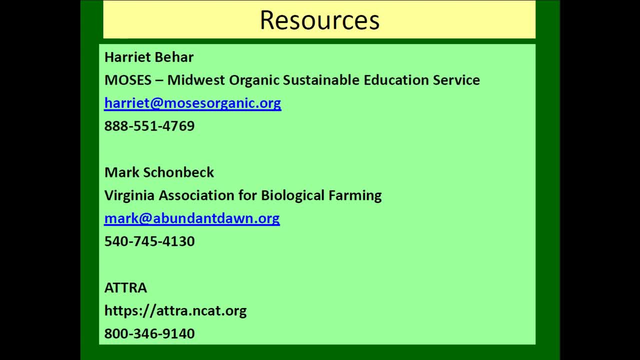 for orchards. Do you have cover crops? Well, yes, I've seen them. Well, mostly. I'm not familiar that much with avocados- We don't grow them here in the upper Midwest- But we do have apples and raspberries And, like I said, you can do. 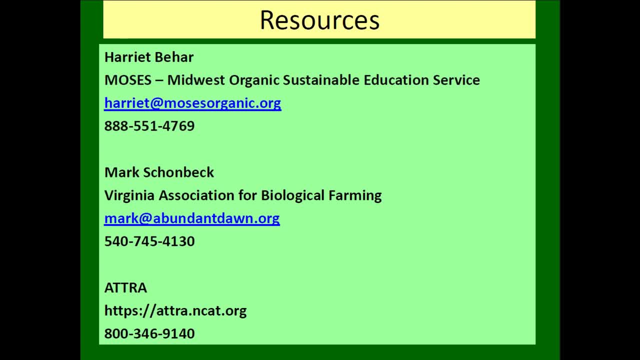 cover crops. You could use fresh avocado and other hard fruits. You could produce a lot more, But as it's kind in the alleyways, You can even do some cover cropping under the trees, And there is something called a weed badger, which is basically a mower that mounts on the side of a tractor. 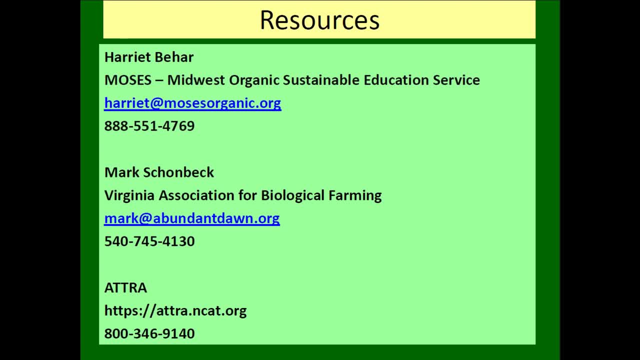 that has kind of an arm, that when it hits the tree it kind of rolls around the tree and then continues And it does a very shallow incorporation of whatever cover crop you might have planted there. So, yes, cover cropping can be very useful. Also, I think that avocados 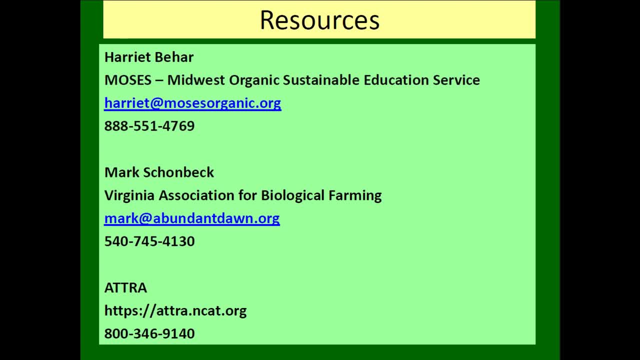 are not as long-lived a tree- I might not be quite correct about that, but I think that they're not like apples- And so thinking about having a couple of years of cover cropping before you plant to really increase that soil tilth and organic matter so that when it does, 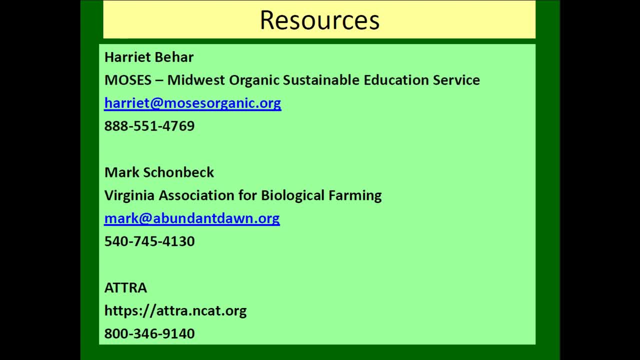 rain. you know you hold on to that. You have moisture, You have better soil structure, so the roots go deeper. All those things can be done in a perennial system right before you plant your orchard and also even while the orchard is in existence. 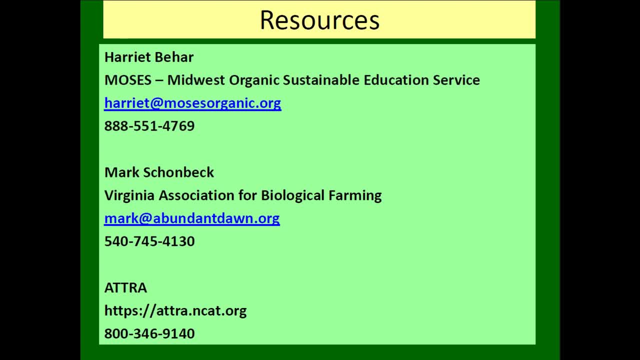 Mark, did you have any comments? I heard you. In addition, this is a tremendous opportunity to grow beneficial habitat by selecting a diverse mixture of flowering plants. Legumes can be used and periodically mowed to provide some nitrogen for the trees And 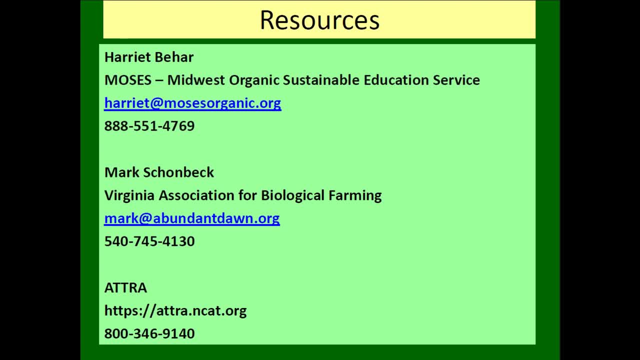 it is vitally important to keep those aisles covered. I think that there's nothing harder on the soil than just to have wide bare soil stretches between your rows of avocado or apple trees or any other fruit. I think that's one challenge is to make sure that the flowering of the ground cover does. 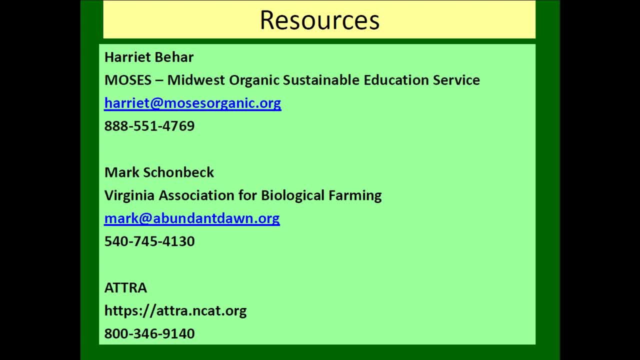 not compete with trees- And I think that's one challenge- is to make sure that the flowering of the ground cover itself does not compete, especially when the trees are still young. That just takes some careful management and timely mowing. Thank you, Here's a very somewhat specific, but I think it gets to the issue of continuous 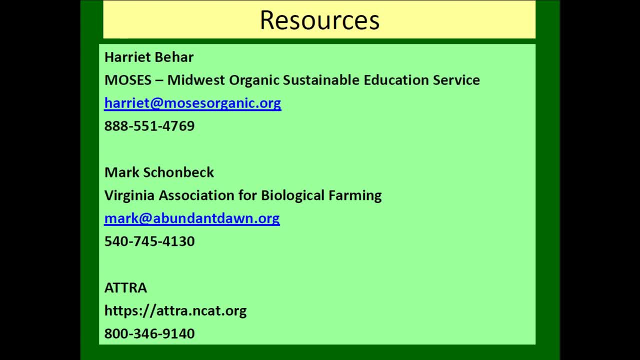 row crop. Where in the NOP rule does it state: continuous row crop is not allowed? Somebody seems to not agree with that, I guess. Well, it's that definition. It's not the definition of crop rotation. So that's the same crop, But it's also a 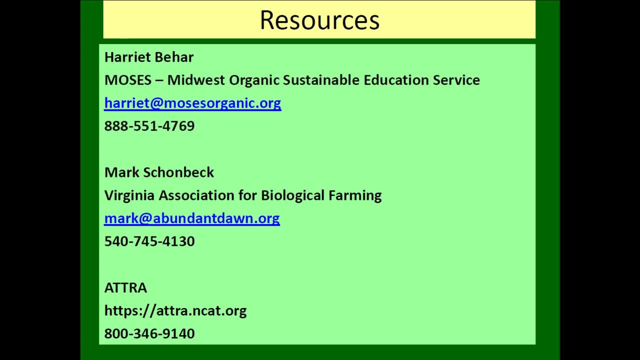 mandate for soil building rotation And that was discussed. the must manage crop nutrients to maintain or improve soil organic matter content And unless you have some sort of cover cropping or sod crop in that rotation you are not going to be able to grow any more. 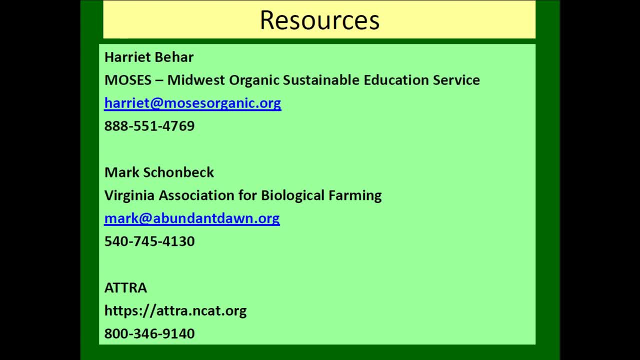 soil And that's going to be maintaining or improving that soil organic matter content. Continuous row cropping, with the need for the tillage to control the weeds, is going to be destroying organic matter rather than improving it. Now to go back, perhaps if someone could figure. 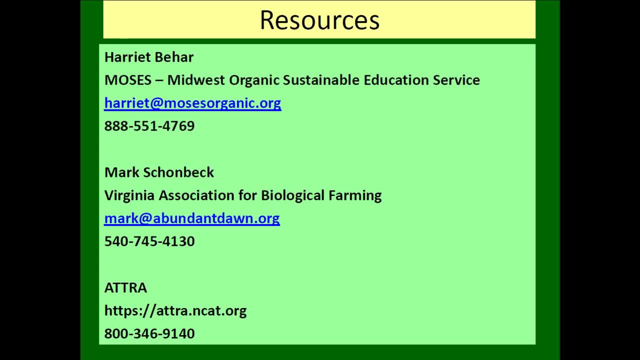 out a way to do continuous organic no-till, where they are rolling down a cover crop and are continually doing row crops in a A mechanically tilled mulch. perhaps you could do that, But it's a little bit difficult to do a continuous no-till mechanically tilled mulch row crop system. 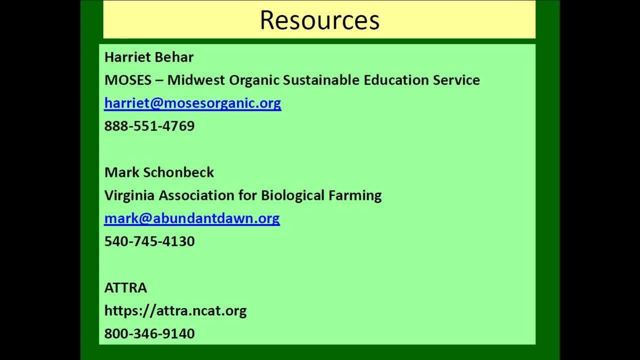 Mark any comments? I think that the comment is referring to like you wouldn't want to do continuous corn corn after corn, even with a winter rind that you cover crops with. I think that the comment is referring to like you wouldn't want to do continuous corn corn. 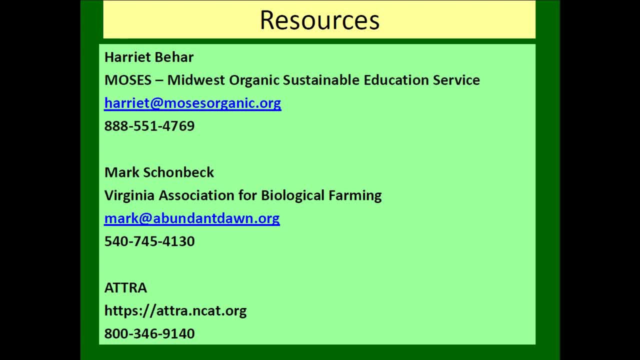 after corn, even with a winter rind that you cover crops with. So you could do a more gentle no-till crop. that would not be permitted. But if you had a row cropping system where your row crops were corn, then soy, then cotton. 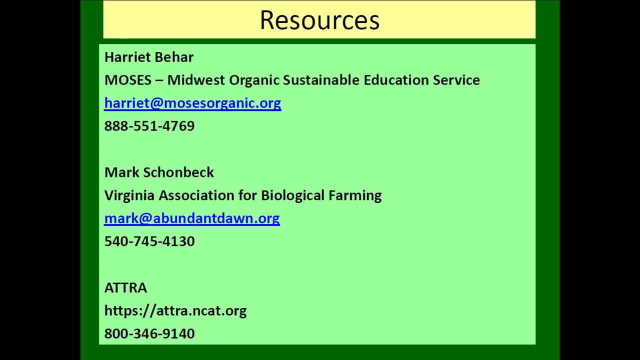 then you had a couple of winter cereal grains in there and you had a couple of legume or legume grass cover crops. You could have a production system that agronomic crops every year, so long as there's sufficient diversity and sufficient residue return. 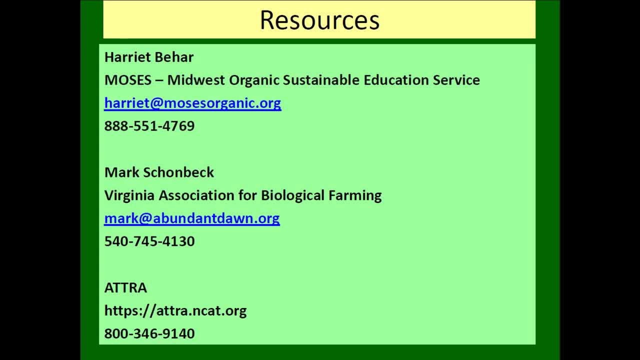 Sure standard says that the crop rotation to build and maintain soil quality would include, but not be limited to, legumes, green manure, sod crops, etc. So we didn't mean to say that you could not have a cropping system that all the production. 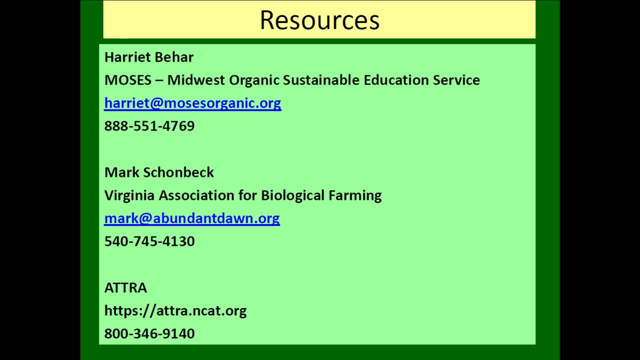 crops were agronomic crops, only that there needed to be sufficient diversity and sufficient soil building crops included, Right? I mean if someone could work out a system where they were intercropping, underseeding red clover in their corn, and then the next year they did beans and they had rye out there. 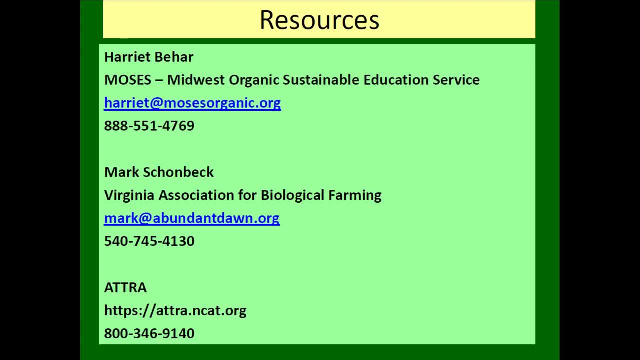 with the beans, then they could go back to corn again, because they will be improving the soil organic matter, because they're not doing quite as much tillage and they actually have more than just crop residue to return to the soil every year. If you remember that one slide from 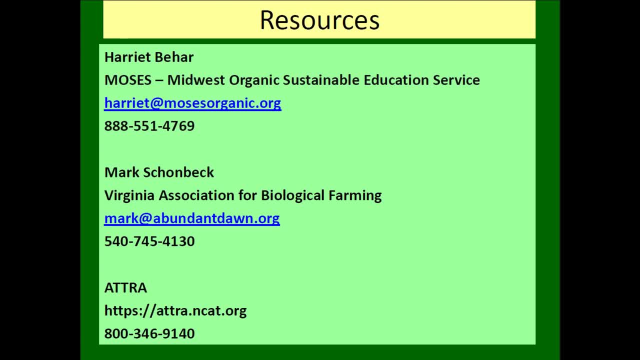 Rodale, the difference between just returning crop residues in a row cropping system whereas a cropping system which also included cover cropping and animal manures, the difference in the color and tilt of those two soils. And that's what we're trying to go for. 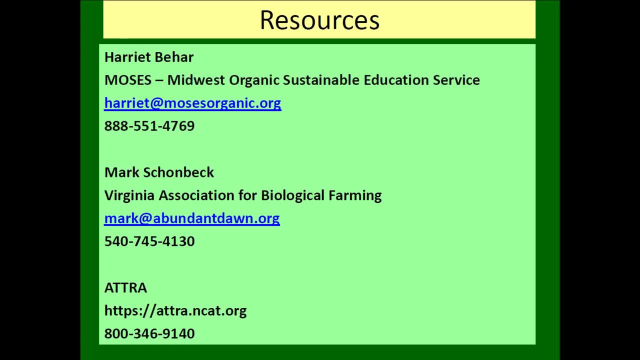 So I mean I suppose someone could do a corn-bean, corn-bean, corn-bean rotation, but they would have to have, you know, be doing some kind of experimental And interesting things with interseeding and getting in those cover crops. so they would. 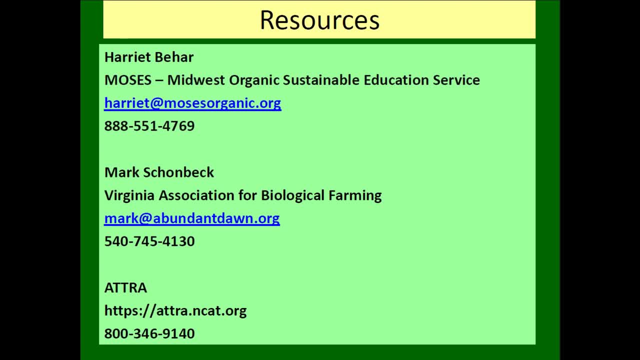 be improving that soil organic matter. Thanks. Here's a. Do cover crops that provide habitat to beneficial insects also provide habitat to insect pests? That is a very important question and that's where the issue of plant families come in. A legume cover crop. 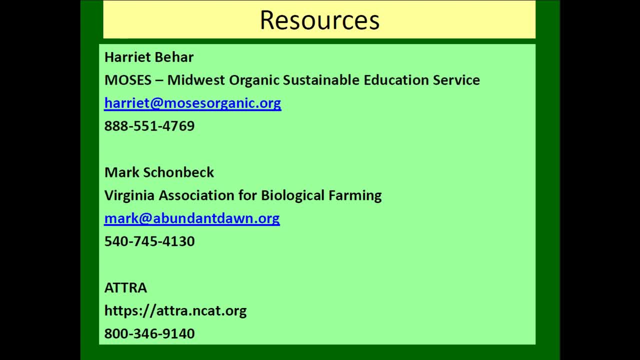 If you're following it with English peas or snap beans, you could run the risk of a pest or disease being harbored. On the other hand, if you are burying the plant family, you're much less likely to run into this. Sometimes, a cover crop will indeed harbor aphids or caterpillars. and that's not all. 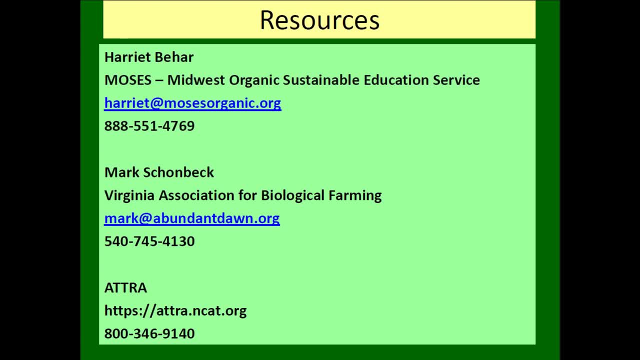 bad because the beneficials come because the plant-eating insects are there. You just want to make sure that If you're growing a small grain or a legume that is creating this ecosystem, where it's got aphids and ladybugs and lacewings- that you don't then try to grow right next to it. 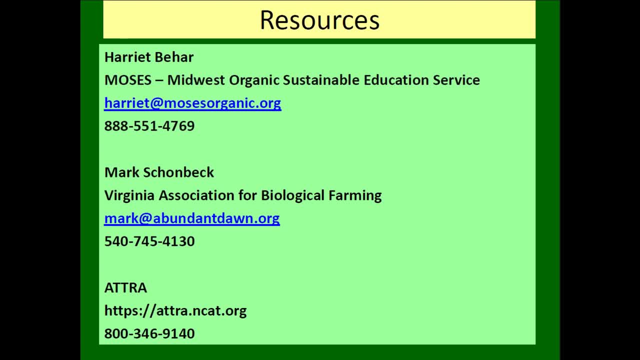 a production crop that is susceptible to the same aphid. Now the biggest challenge comes up with pest nematodes, And, for instance, pest nematodes will oftena given. nematode species such as root knot will attack several plant species. 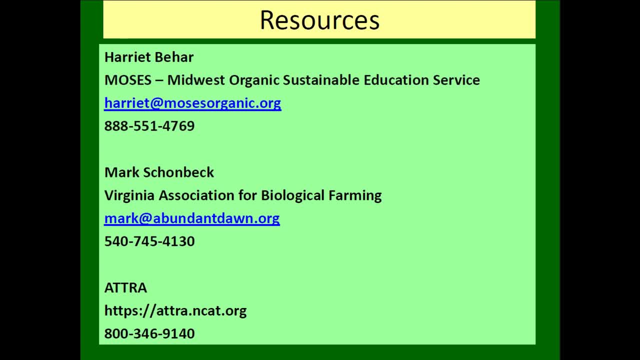 So if you're in an area with root knot nematodes, growing crimson clover or red clover ahead of tomatoes is not a good idea. Now, if you're in an area where there isn't much root knot nematode, no problem. 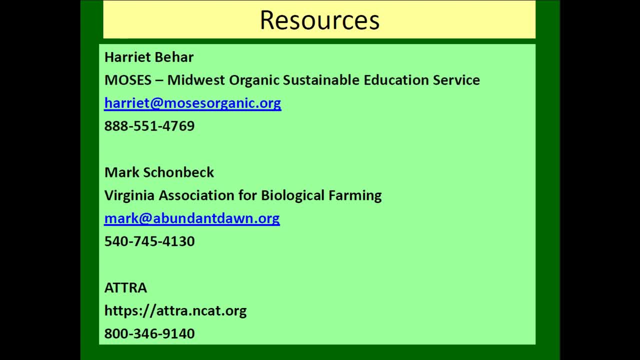 The tomato is going to thrive on the legume nitrogen and there will probably be beneficials that the legume has, encouraging the soil organisms for insects. Now, one thing to remember about pest nematodes is their abundance is often as small as they are. 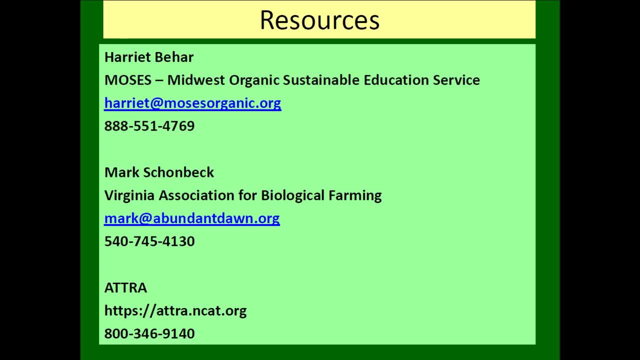 It's a symptom of poor soil quality and low diversity of the soil biota. So just by implementing a good crop rotation and ensuring adequate soil organic matter return, perhaps using some compost to provide an inoculum for beneficial organisms, will in general tend to reduce nematode problems. 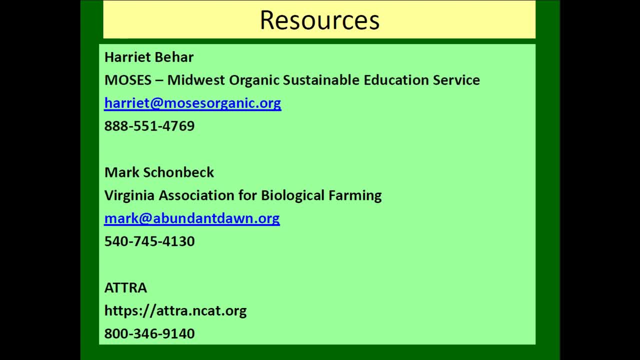 There are situations, however, even with those measures, that a certain nematode pest will be a serious problem. This question- The crop rotation manual that we discussed a few minutes ago- is an excellent resource on determining whether there is a nematode carryover problem between a particular cover. 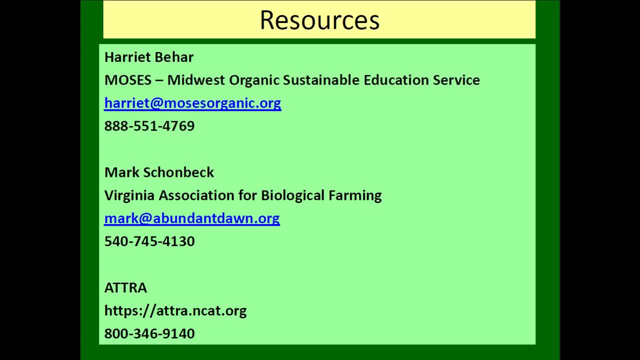 crop and the next production crop. Thanks, Mark. This is from central Florida and it maybe also helps with another question that was more general about tropical and maybe semi-tropical. We did have a Okay, A webinar on this earlier in this series, which I would also point folks to see on the. 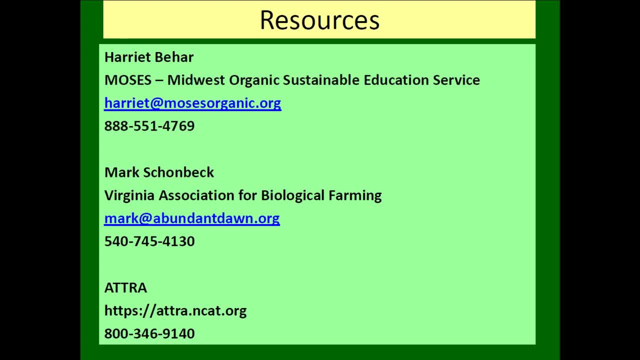 ATRA website. But the caller says: I live in central Florida where we get loads of rain bugs and fungi during June through September. Do you recommend no growth during this period or any other recommendations? And that's actually. Some people are talking about having a kind of fallow period, I guess, as well as part. 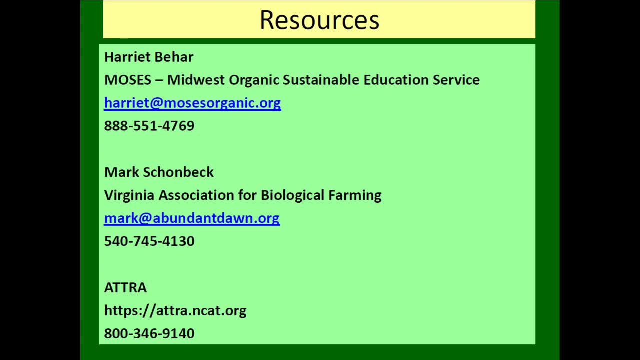 of a rotation. This is Mark. again, I would say, in a hot, humid climate like that, avoid bare fallow like the plague, But by all means take a break. Don't be going out there trying to battle insects and harvest vegetables in 100 degree. 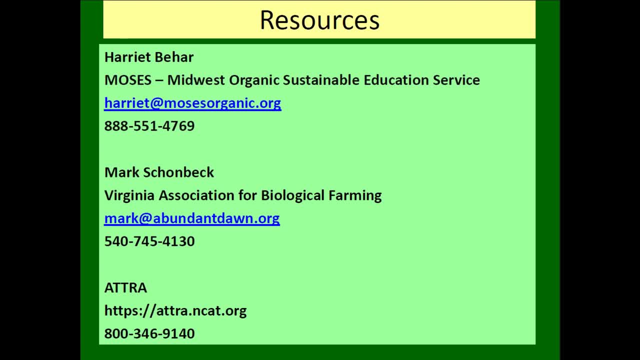 heat and humidity. Plant it to a very heat-loving cover crop like sorghum, sudan or pearl millet, along with a vining cowpea, And just let that field make biomass And plant it in a very humid climate, And then you can. 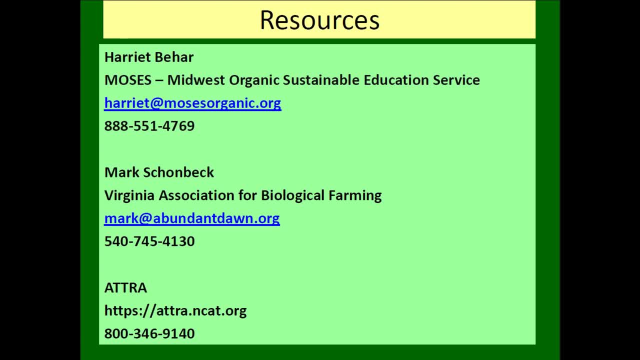 The bugs are gonna be suppressed, The weeds are gonna be suppressed. You're gonna be breaking up your fungal disease life cycles by not planting their favorite production crops. The rain is just gonna make those crops give you tremendous biomass And I'd say, make sure you have a flail mower or other means to manage the biomass when. 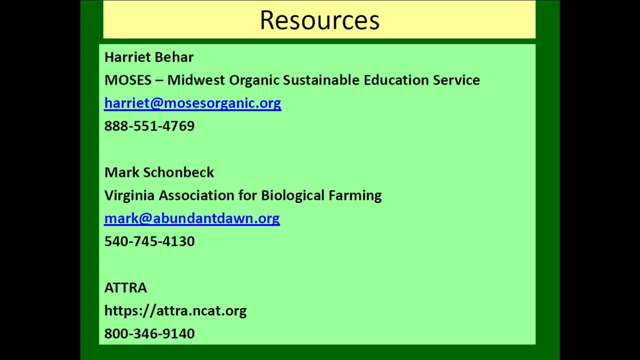 you're ready to plant your fall crops And you might even be able to no-till them. Yeah, I agree. Any kind of black fallow, just bare dirt, Especially if it's a very hot, humid climate, If it's a very hot, humid climate. 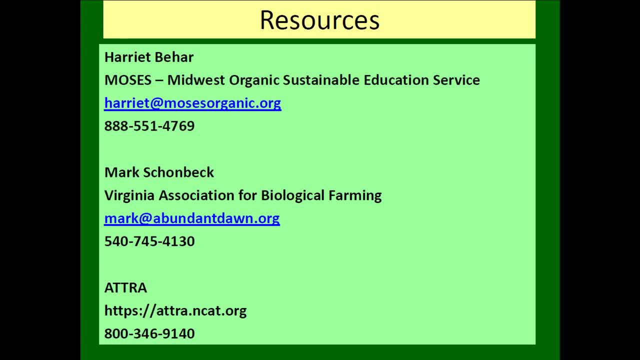 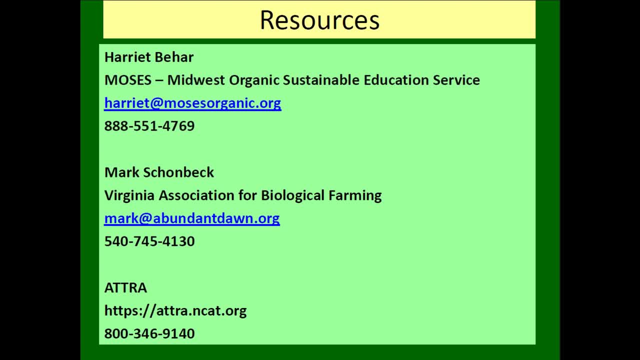 And I think what Mark suggested was a good idea. I don't know, There might even be other cover crops that grow real well in your region, But since I'm from Wisconsin I don't know Florida that well. I just want to add that there is an extension person in Baton Rouge, Louisiana. 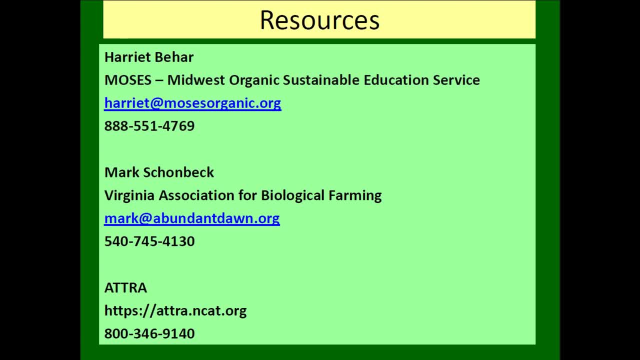 Her name is- Yeah, Her name is Milagro Berhani, And the way she has dealt with the severe weed pressure is to grow a spring vegetable, rotate into a summer cover crop of cowpeas or cowpeas and sorghum, and then back into 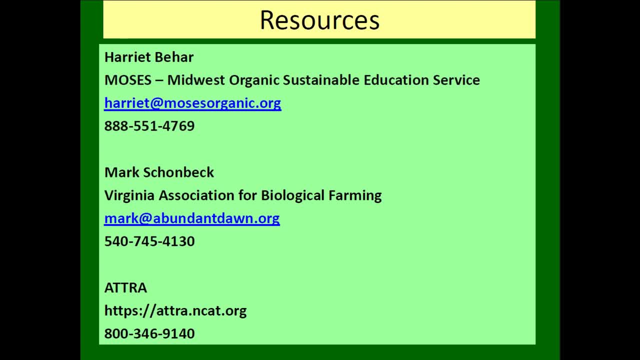 summer vegetables. I just found that that solved a lot of the weed problems, in addition to restoring soil quality. So there's a lot of practical examples of this. Mark will probably appreciate this question And I Um. Are there ways to objectively measure improvements in soil quality to ensure that these soil 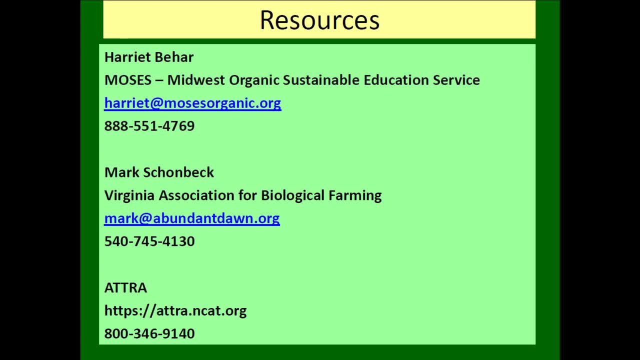 building practices through rotation and cover crops are actually working. Oh, that is a tough question. I have found that measures of soil organic matter percentage. they're very approximate. You can get very variable figures. that can be frustrating if they jog up and down. 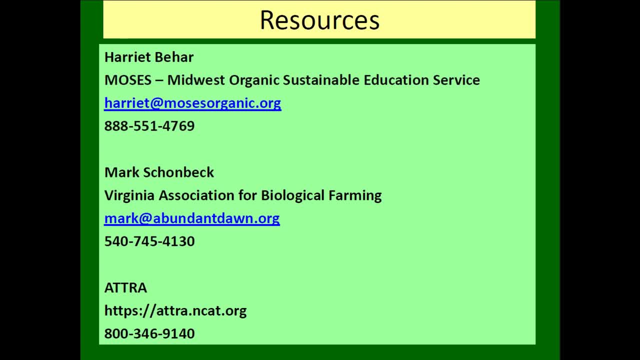 There's a newer technique of measuring what's called accuracy. I don't know. I think it's called accuracy. I think it's called accuracy. So we're measuring what's called active organic matter, That's, the recently formed and broken down organic matter that turns over relatively. 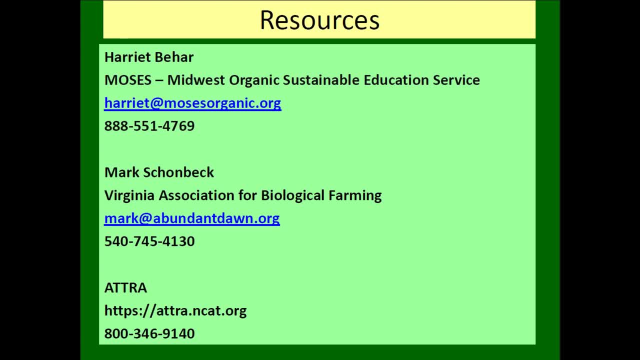 rapidly consists of the soil biota, and it's an immediate byproduct and is the source of the slower-release nutrients that I mentioned. If your soil is being well taken care of, it will tend to have more active organic matter. However, I 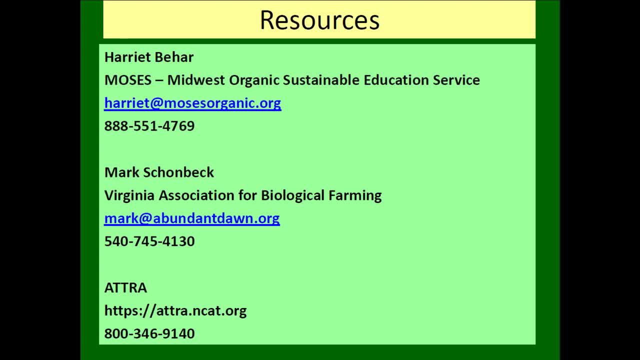 At this point I would say that just the visual observation of things like the color and texture of soil, like you saw in that side-by-side picture and applied to a fan, and also the on that side-by-side comparison in the slide of the Groddale experiment, the crop performance. 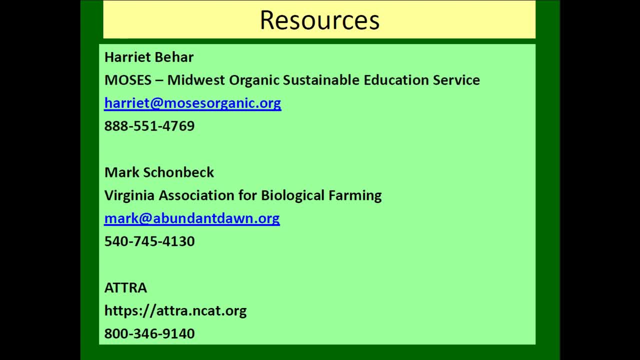 The farmer really knows when a field is getting tired. It really needs to be put down to a perennial cover or a very high biomass annual cover And on the other hand, farmers can see very clearly. You'll see it in crop performance. You get a dry summer like a lot of people have had this year.